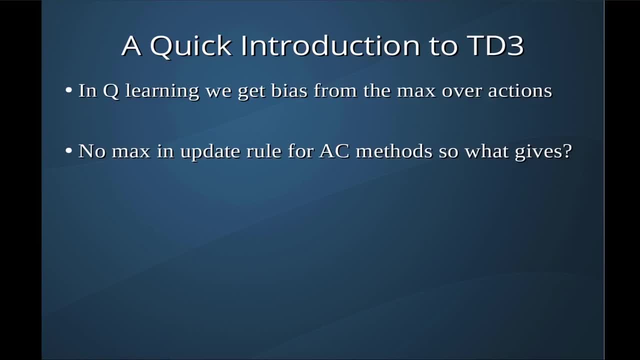 of it is that we have stochastic gradient ascent or we're attempting to maximize the product of our probabilities, our policy and the rewards or returns the agent receives over time. so there is some implicit drive to maximize score over time and so when you get natural variation in your rewards or 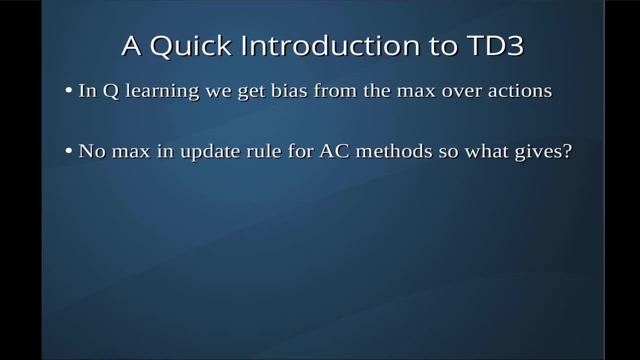 in the trajectory through the state space, you can end up with some incorrect estimations of the values of states because of natural, you know, high variance, which is typical for deep reinforcement learning problems. however, more fundamentally, overestimation comes from approximation errors. now, this isn't something they prove in the paper, because this is a result that dates all. 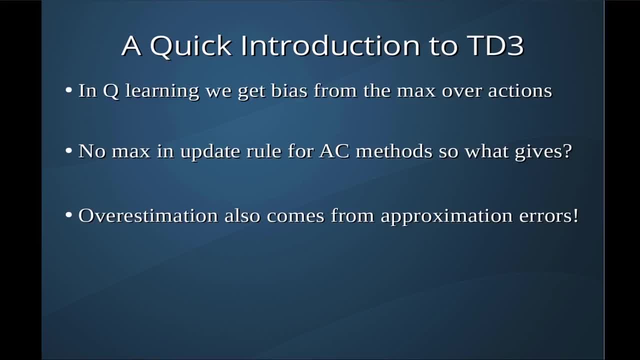 the way back to the early 1990s, when people were just starting to talk about Q learning, and so it's been known for a while. but the basic idea is that when you attempt to use some mathematical apparatus to estimate a function in a high dimensional space, you get. 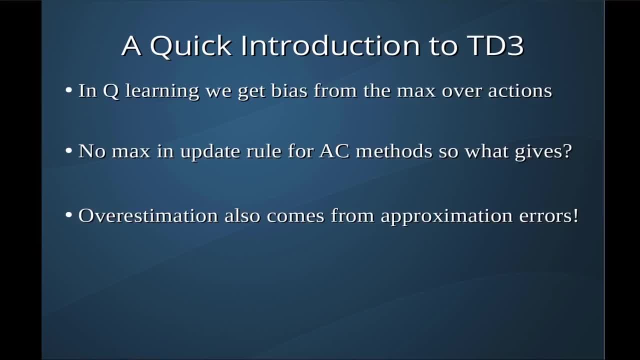 approximation errors and that results in overestimation. now what is our source of overestimation or approximation error? in this case, it's going to be a deep neural network. neural networks are, of course, universal function approximators mostly. there are obvious exceptions. you know discontinuous functions, they can choke. 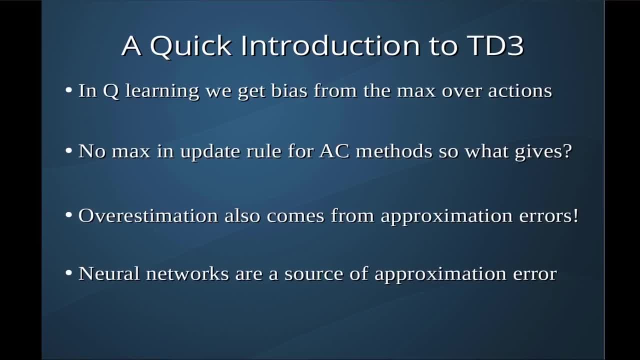 on, the function has to be differentiable and all that good stuff. but for all the stuff we deal with- neural networks- are you going to be a universal function approximator and so that leads to a source of error. now, this is inherent to any approximation method, either tiling, 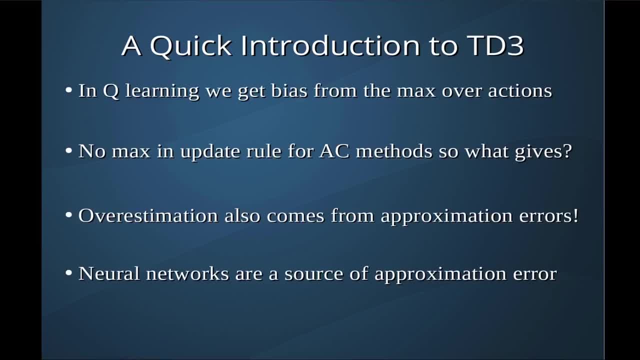 like binning, anything like that. so it's not that neural networks are bad, it's just whenever you have a function approximation, you're gonna have some error. okay, because you don't have an infinite amount of time to collect an infinite number of samples to get infinite precision. you're always gonna. 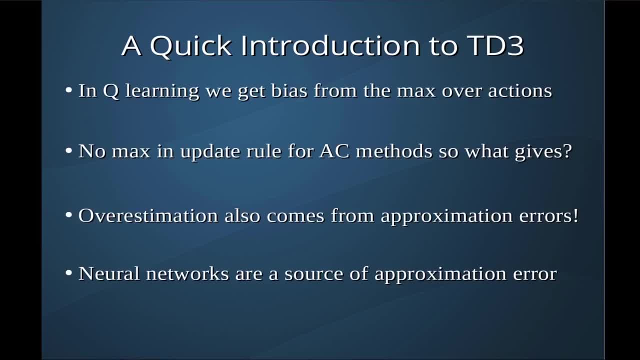 have to lop off your estimate at some point where there are more decimal points waiting for you should you be able to collect more data. worse yet, actor critic methods are bootstrapped. what this means is that we're going to be using our initial estimates to 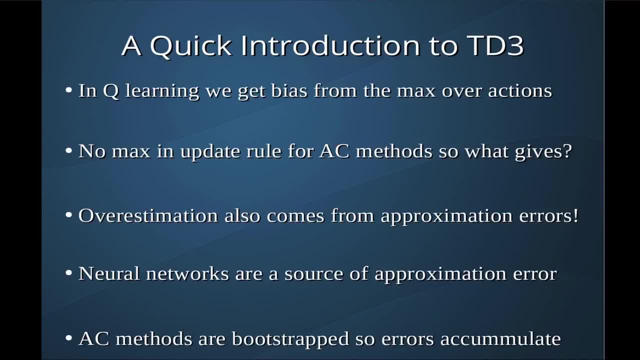 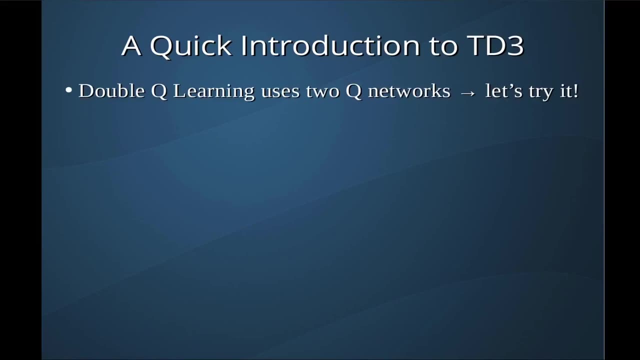 perform updates to later estimates, and so you have some errors in your early estimates that propagate to your later estimates over time. so you get an accumulation of error over time. now, naturally, there are other ways of dealing with this and, in fact, Double-Q learning, a rather ingenious solution. they use in that algorithm two different Q networks. 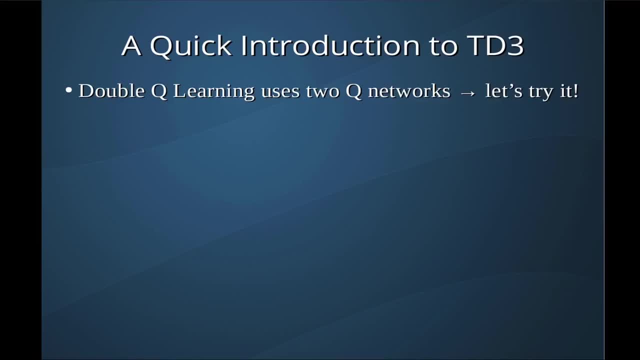 and you alternate their use in the update rule, and so you're never taking a max over actions of the same network that you use to choose an action when you're trying to update the value of that action, and so it seems like it's a reasonable thing to try. so, in particular, that's what they do. now I want to point. 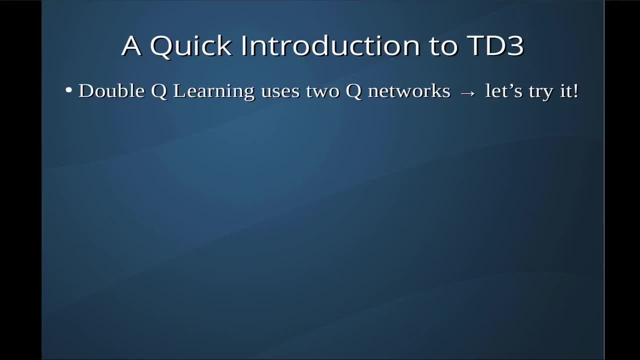 something out that in double Q learning- deep, double, deep, double Q learning- they use a not exactly analogous solution to the tabular case of double Q learning. they use something slightly different which doesn't work in actor critic methods, as they detail in the paper. they're going to use a more exact 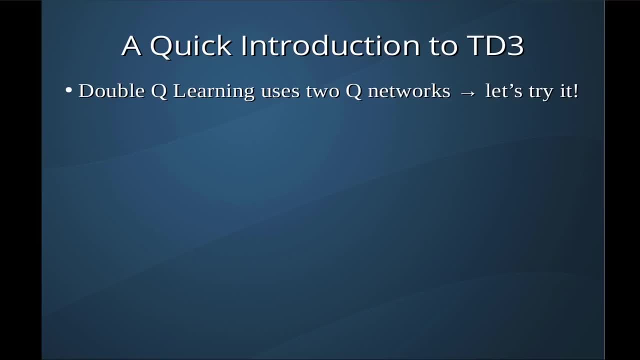 replica of the tabular versioning of double Q learning, and they're going to perform a slight modification where they're going to clip the inputs of the actions to the Q networks, the double Q networks, which is going to tend to underestimate the actual Q learning that they're doing, and so they're going to 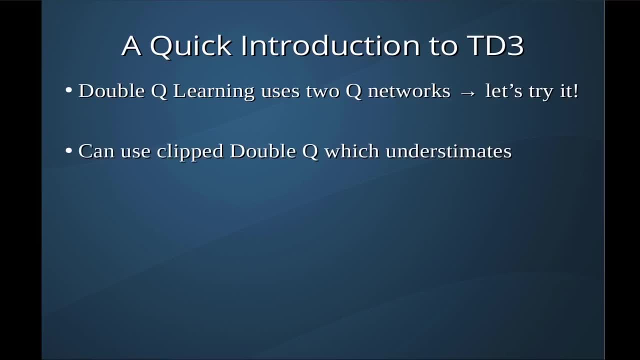 underestimate and we're going to be taking a min. so later on you'll see in the algorithm that we're going to feed some clipped actions to our Q networks and then take the minimum. so whatever the minimum value is, we're gonna take that which tends to underestimate. now you may say, dr Phil, isn't that a? problem? not really. and the reason it's not a problem is because if we underestimate actions, those actions become less attractive to the agent and so it's not likely to take those actions again, and so that kind of dampens that out over time. it's a natural feedback mechanism. 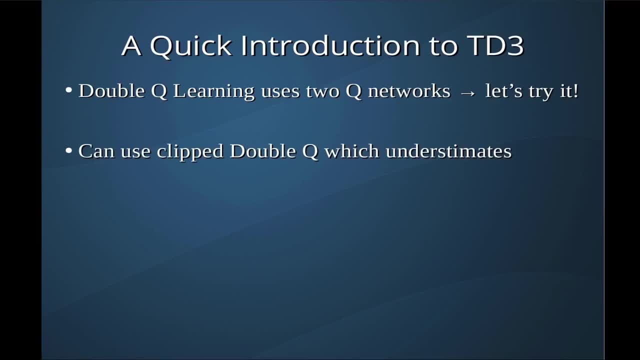 to deal with that issue. so that is rather nice and it's baked right into the algorithm. the other innovation is that they're going to delay policy updates to give the critic network time to converge. so the policy network is very slowly changing function, whereas the Q network can change much more. 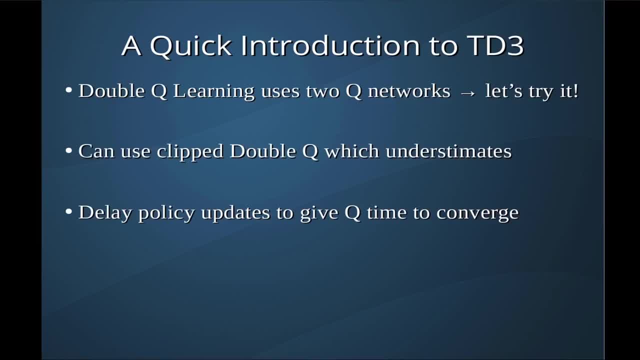 quickly. so you have two different time scales there, and that's where the delayed part comes from. another innovation is we're going to use target networks for the actor and both critics. since we're doing an analog of double Q learning, which uses two Q networks, it stands to reason we're gonna have two. 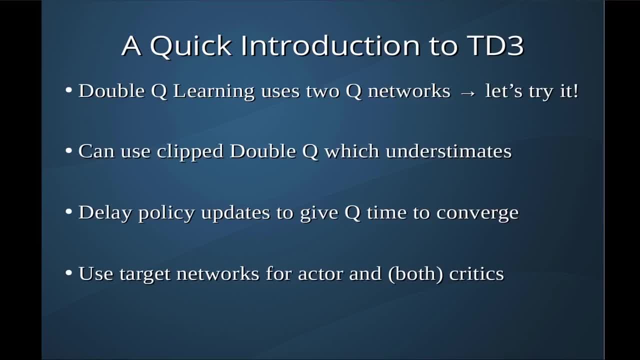 critics and we're gonna target networks for all the things. so we're gonna have an actor, a target actor, two critics and two target critics, so a total of six deep neural networks. we're gonna have all the neural networks in the world. the other thing we're gonna need is a soft update. 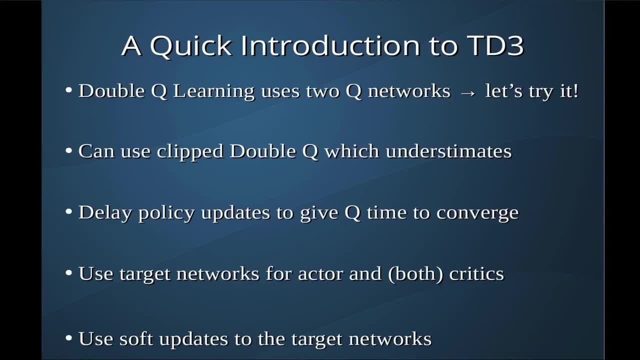 to the target networks. so you have a couple of options for updating the weights of your target networks. one is you could do a stochastic gradient descent on those directly. another option is to take the parameters from your online networks that you're actively performing gradient descent on and copy those to the target networks directly. or a third option is to do some 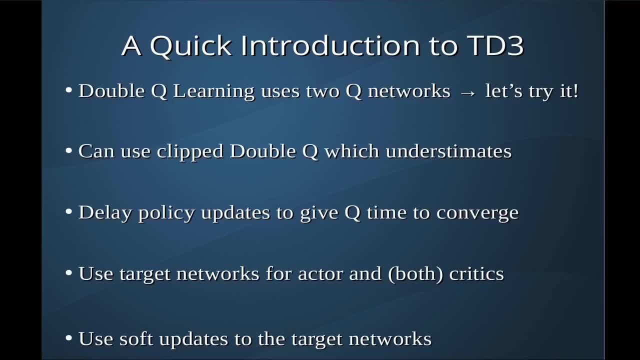 slowly varying, interpose between the two. so you're gonna update the online network and update follows the target networks every time step or every end time steps. Are you in search outcomes for the past few months? zoomed in to the review page in the case of the policy and then you can do some slowly changing update to. 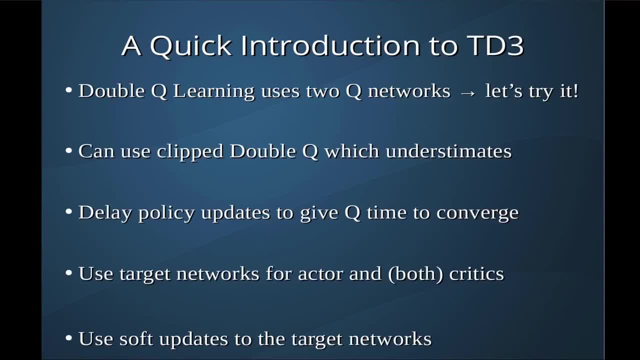 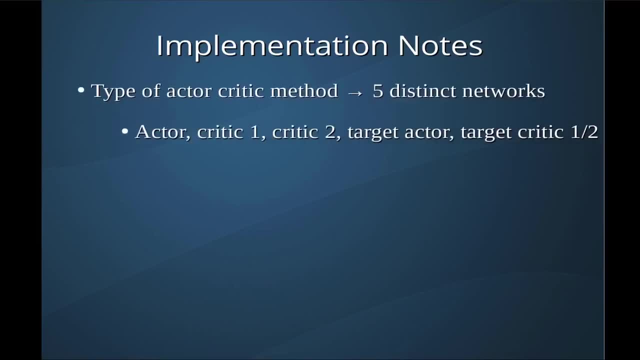 those target networks and that will introduce an additional hyperparameter called tau to our agent, which you will see later. so this is an actor critic method and we're gonna have actually six distinct- I have a typo there, sorry, I can't count, despite having a PhD in physics. so we're gonna have an actor two. 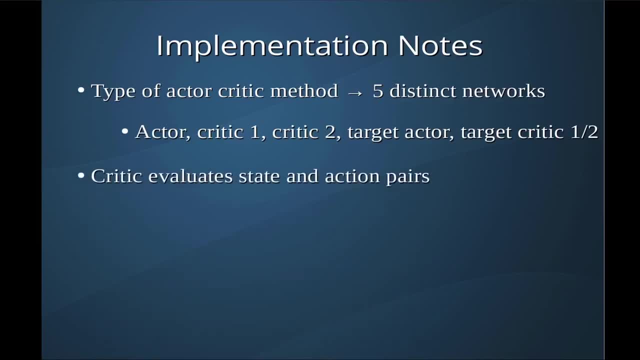 critics: a target actor and then two target critics. as I said, three, two end. we have the over eight point check on the Heiminger 계ип contractor versus a. the purpose of the critic is to be critical. It is to evaluate the values of state and action. 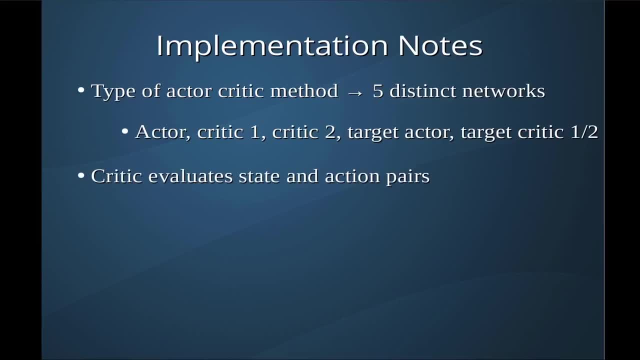 pairs. So it says, hey, in this particular state we took some action. I think this was valuable or not, And that will help to update the agent's estimate of the values of those pairs and to choose better actions for given states over time. The actor will decide what to do based on the 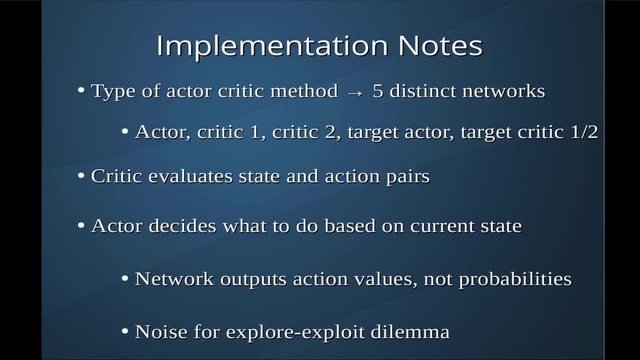 current state, And it's important to note here that our deep neural network is going to output action values, which are continuous numbers, not discrete numbers, not probabilities. Now, that makes this a deterministic algorithm. That's where the name of the algorithm comes in. 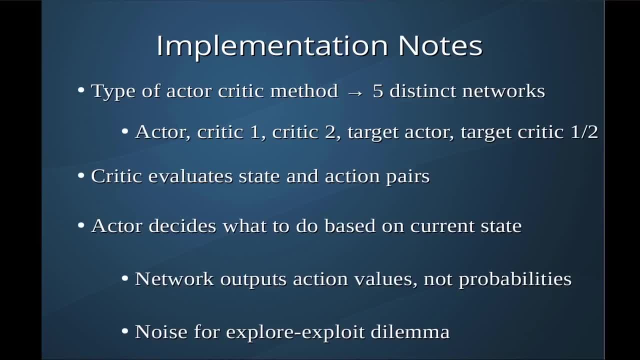 twin delayed deep deterministic policy gradients. It's an extension of deep deterministic policy gradients, And so we have a bit of a problem there, because we're dealing with approximation. right, We're approximating a Q function, We're approximating a policy, We're approximating all the things and we never know exactly how accurate our 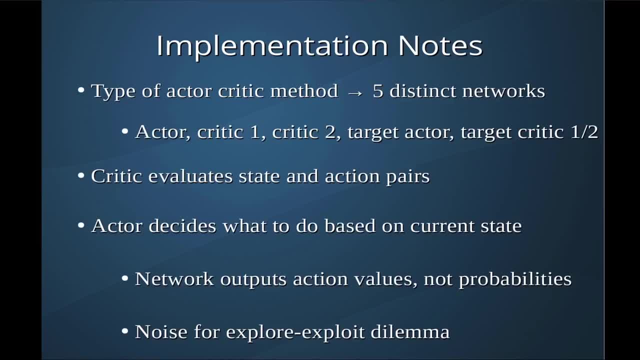 approximations are, And so we never know if we are correctly evaluating states and action pairs. So we never know if, given some state, if this action is really the most beneficial action we could possibly take, or if there's some other more beneficial action out there waiting to be. 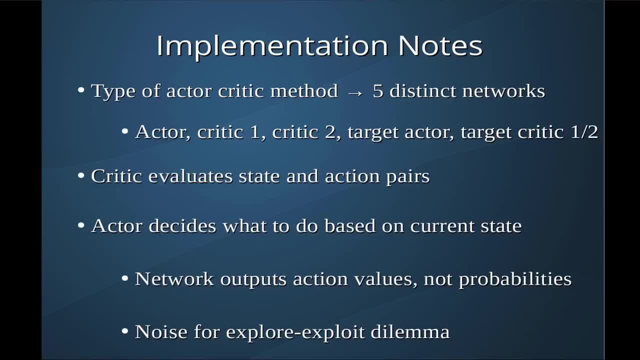 discovered. That is called the explore-exploit dilemma. Do we explore suboptimal actions or exploit what we think are the most beneficial actions? And the extent to which you engage in those two activities is the dilemma, And there are a number of solutions to that. Deep Q learning uses, epsilon, greedy action selection, where you just take. 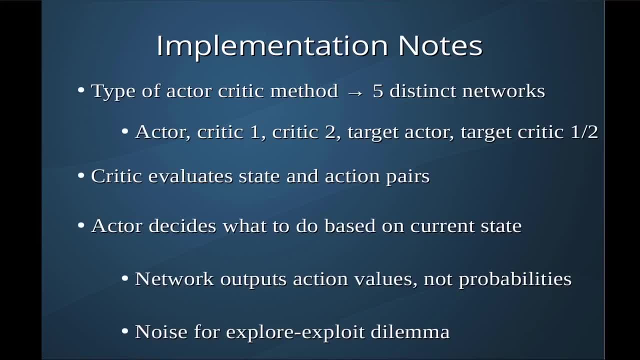 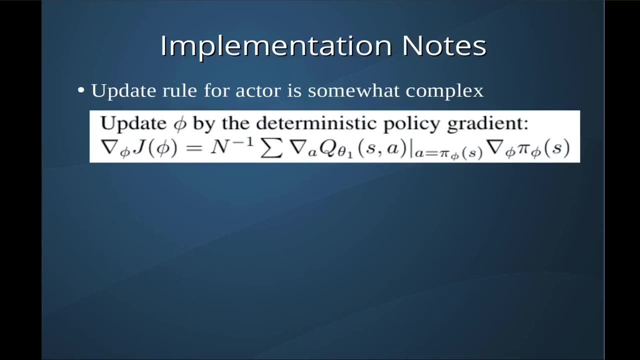 random actions some fixed proportion of the time, But in this case we're going to be adding noise to the output of our actor network when we decide what actions to take. The update rule for actor looks a little bit scary, but it's actually not, So this is the. 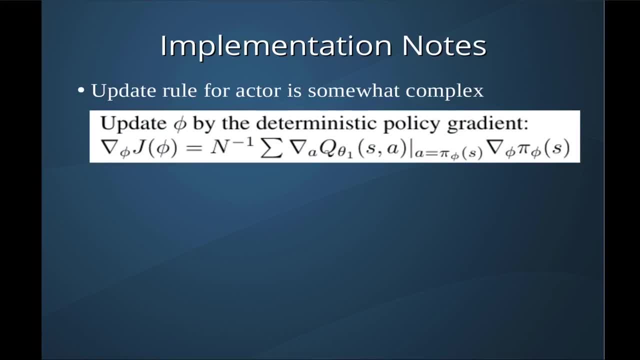 update rule from the page And it's a little bit scary but it's actually not So. this is the update rule from the page. J is going to be our loss function for our actor. it's a function of Phi, the parameters of the policy network, and you want to take the gradient of the cost. 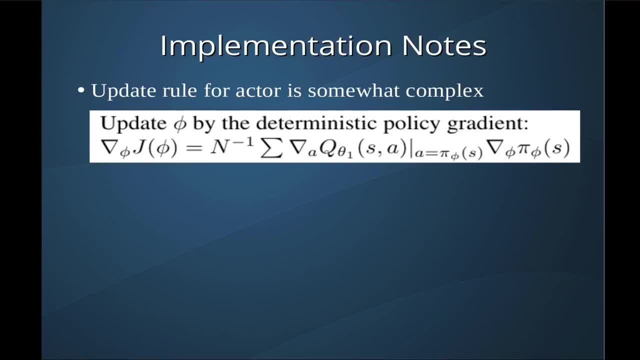 function with respect to the parameters of the policy network and it's given by 1 over M times the Sun, the sum or a mean, an average. so our loss function is going to be a mean and it's going to be the product, in this particular equation of 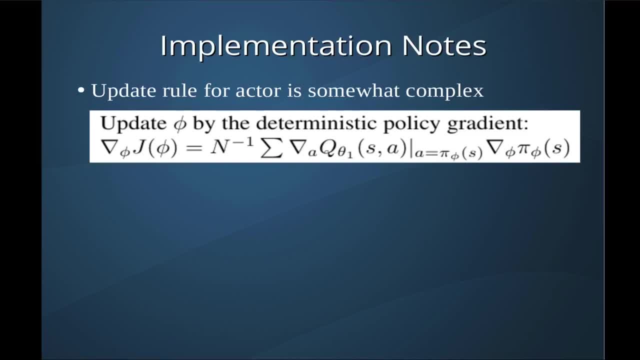 the gradient of the first critic network with respect to the actions chosen by the policy network, multiplied by the gradient of the policy network with respect to its parameters. now this looks intimidating, but it's actually not. this is the application of the chain rule to the loss function. so they have. 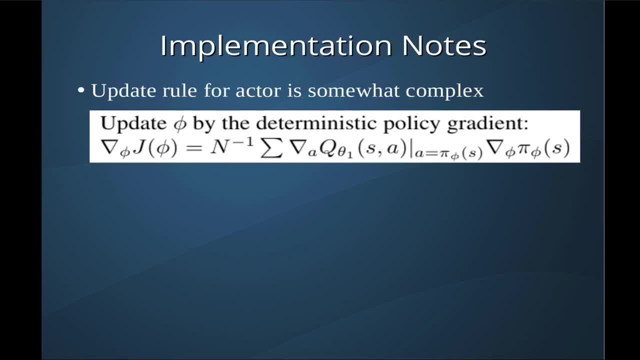 taken the gradient of the loss function with respect to Phi. but the loss function is proportional to the output of the first critic network. of course the first critic deep neural network has its own set of neural network parameters. it doesn't have an explicit dependence on the neural 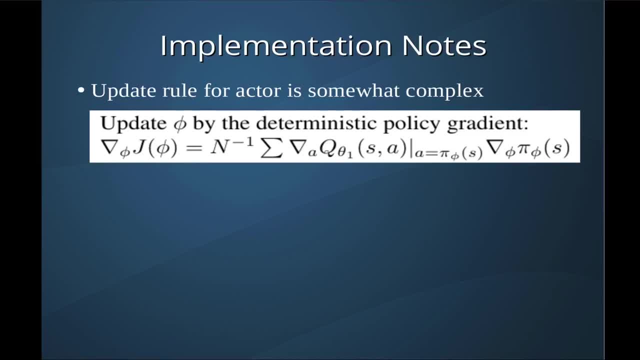 network parameters of the policy network. so it's very difficult to take a gradient right of something that doesn't depend on something else. so the dependence is implicit. it comes from the fact that those actions are chosen according to the output of our policy network, and so you have to apply the 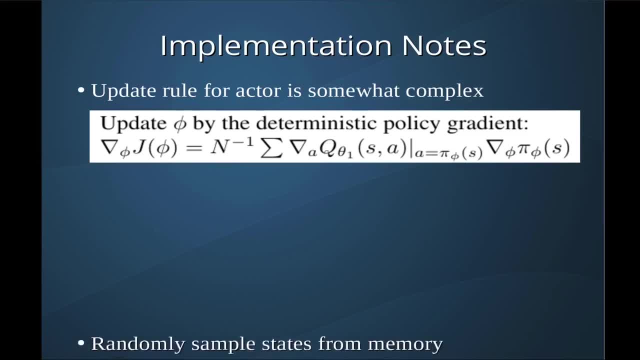 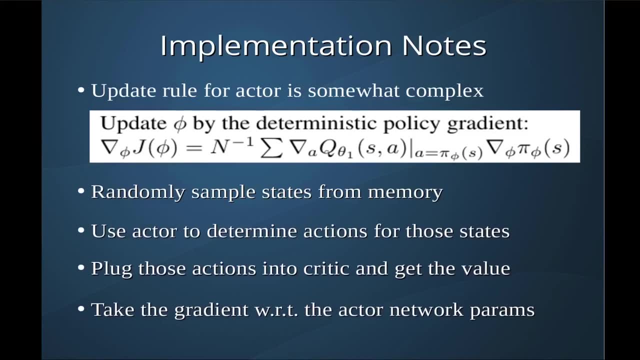 chain rule. in reality, all we're going to do is the following: we're going to randomly sample states from our memory. we're going to use our actor network to determine actions for those states. so we're not going to be using the actions from our memory. we're going to figure out what actions the 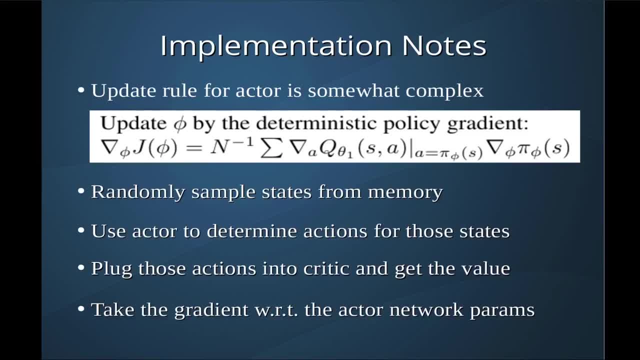 agent thinks we should take. now we're going to plug those actions into our critic and get some value, specifically the first critic, never the second, only the first. that's just by design. and then we're going to take the gradient with respect to the actor network parameters. now we don't have to calculate that. 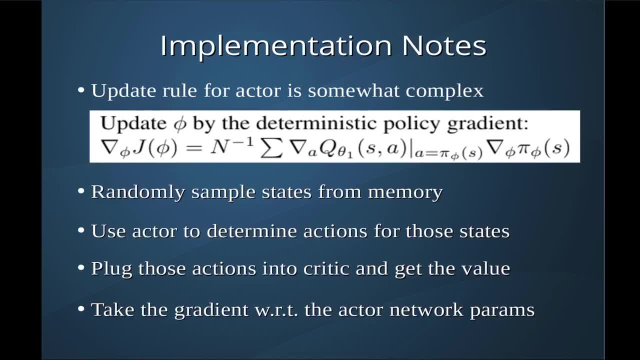 gradient tensorflow is going to do it for us. we just have to do the first three things where we sample states, use the actor, determine actions for those states and plug those into our critic along with the states to get some value, and then take the gradient with respect to the actor. 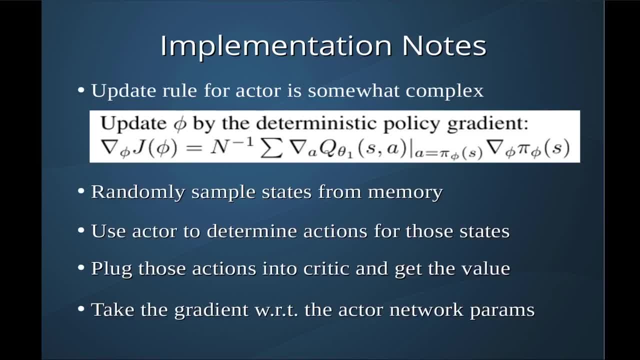 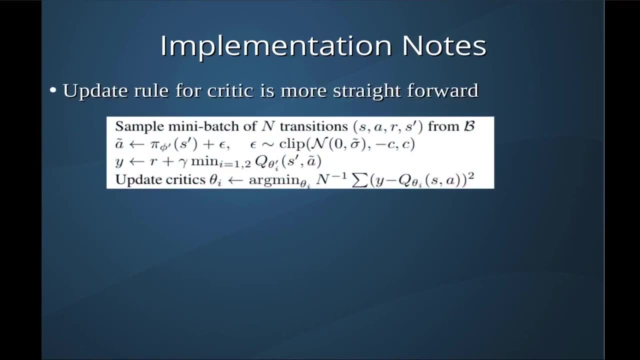 network parameters. now keep in mind that this update isn't performed every time step. it's performed every other time step. how often? e performant is a hyper parameter of the algorithm, but it is not every single time step. now, nominally, the update rule for the is a little more straightforward. So again you're going to sample a batch of transitions from your 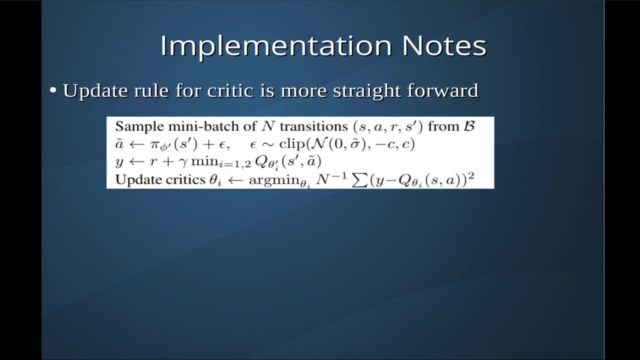 memory. You're going to put the new states that the agent observed after taking some action through the target actor network. That's that A tilde parameter there- And then you're going to add in some clipped noise. It's just going to be a normally distributed noise with mean zero and 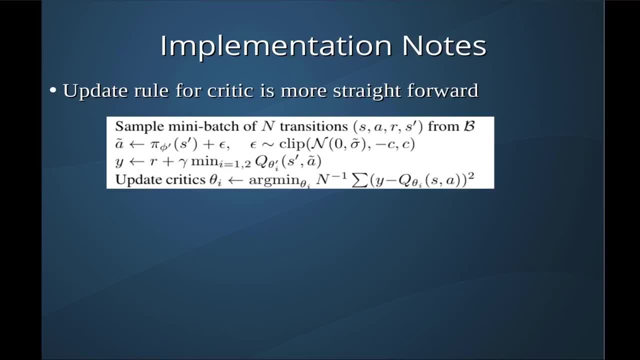 some standard deviation, something like 0.2. And we're going to clip it in the range of minus 0.5 to positive 0.5.. So that's where the clipping comes in for our double Q learning And the actual double Q part comes in when we calculate our targets Y. So we're going to take the reward. 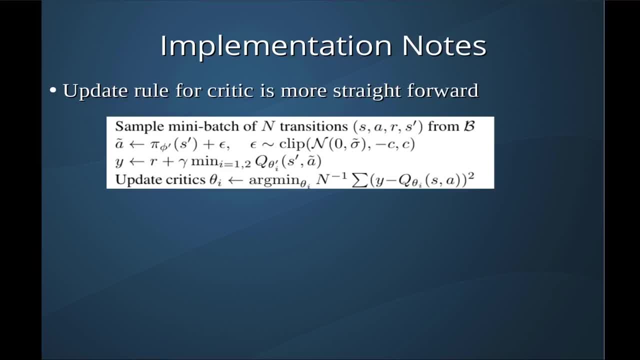 that we sample from our buffer and add it to the product of the gamma, which is the discount factor- 0.99 or so- And we're going to take the minimum of the output of the two target critic networks. So we'll say we're going to feed the new states through 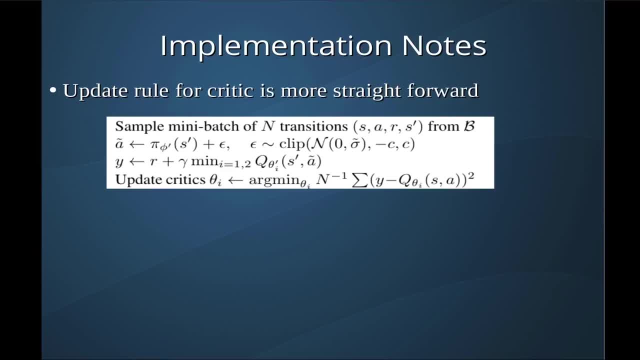 the new states are going to feed the new states through the new states. So we're going to feed the new states through the new states And we're going to feed the new states and those clipped actions through both target critic networks. And then we're going to see: 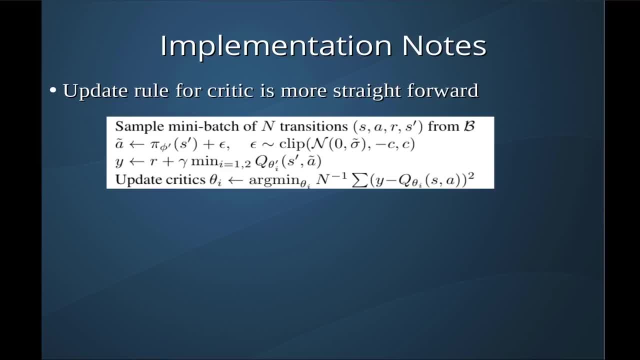 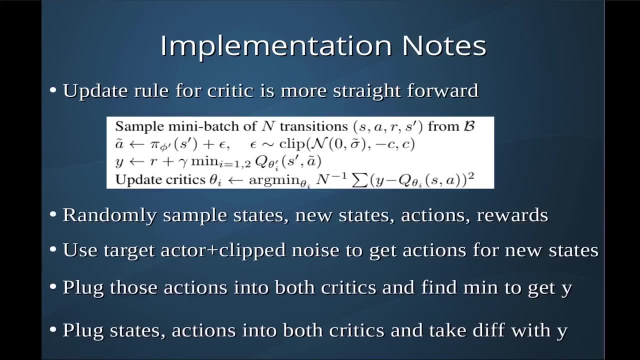 which one is the minimum, and take that for our target value And then we're going to input that target value into our loss function. Again, you have a one over N multiplied by some, multiplied by something squared, That is a mean squared error And it's the mean squared error between: 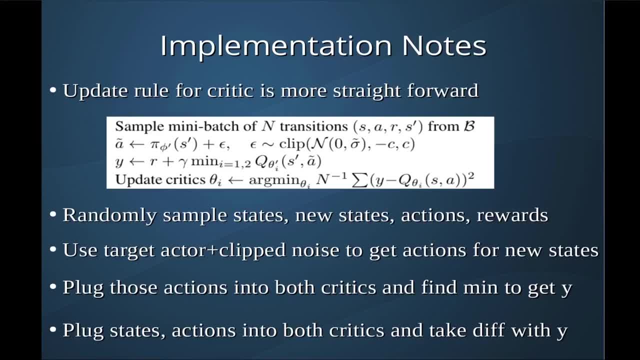 that target Y and the output of both of our critic networks. So our loss is going to have two different components. It's going to have two different components. It's going to have a loss for critic one, where you have Q sub theta sub one, and then it'll have a loss for Q sub theta. 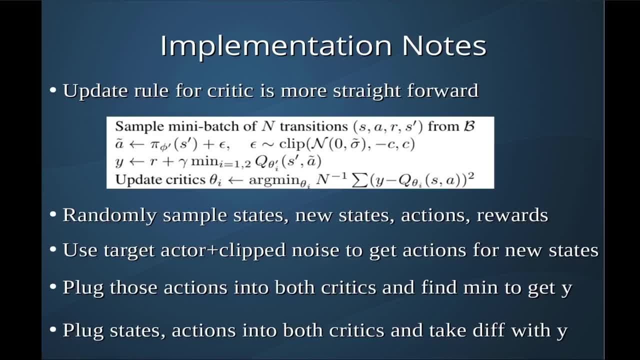 sub two. So we have two losses. And in TensorFlow 2, when we do our gradient tape we're going to have to pass in the persistent equals true flag to our function call so that it keeps track of network parameters between gradient ascent steps. And so these the rest of this verbiage is just. 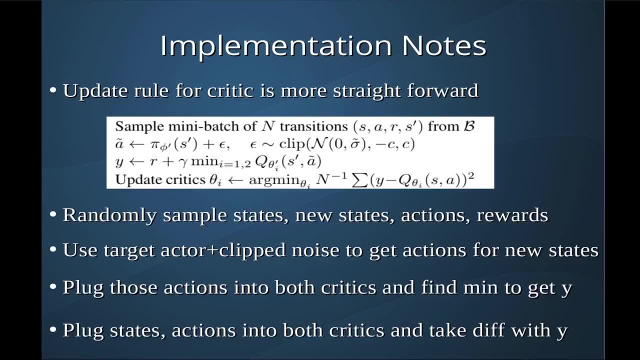 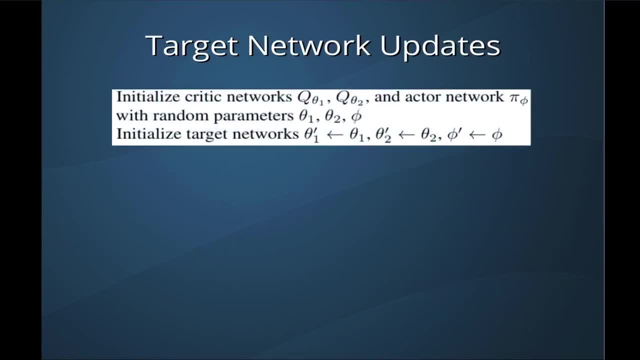 kind of the verbal description of what we want to do. It's going to be much easier when the argument is built. Once you see it written in code, I assure you it's not that difficult. Next, we have to handle the question of target network updates. So at the very beginning, 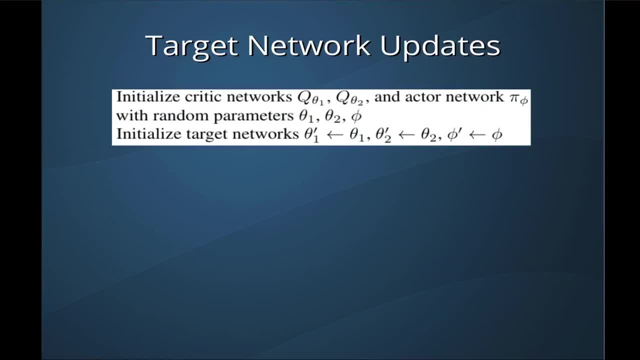 in our constructor, for our agent class. we're going to go ahead and initialize actor, two critic networks and then a target actor and two target critic networks And when we first start out we want to initialize those target networks with the exact values. 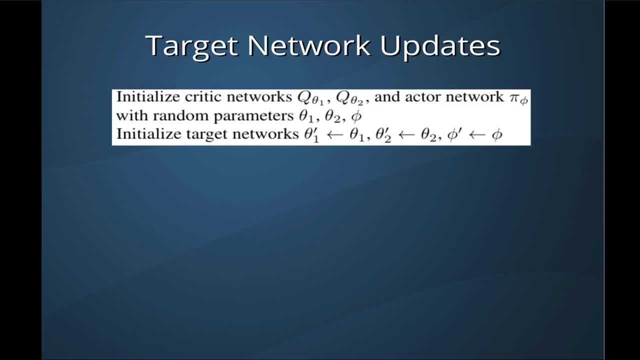 of the um networks, and so we're gonna have a special case in our target network update function that handles the very beginning of the program. every other time step we're gonna use the following expression to update the weights. so on the left side you have theta and Phi Prime, where the eye on the theta D denotes either. 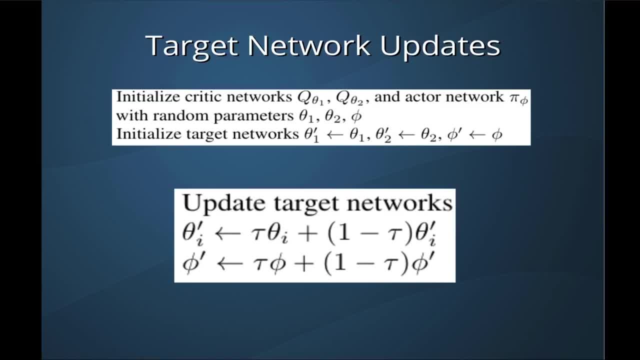 critic one or two. Phi is the parameter for our critic network- excuse me, policy network- and the Theta's are the parameters for our critic networks. and so you're gonna multiply tau, some small number, point, zero, zero, five, in this case, by the values of the current online network and add in one minus tau times. 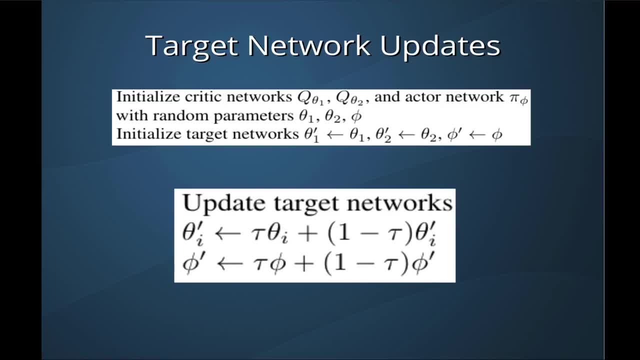 the old values of the on the critic networks. so it'll be a small number multiplied by the current values of your online networks, plus something that's almost one multiplied by the old values of your target networks. it's gonna be a slowly changing update to our target networks. other thing to note is that 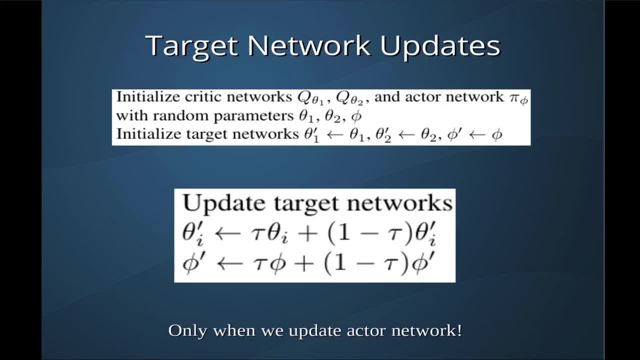 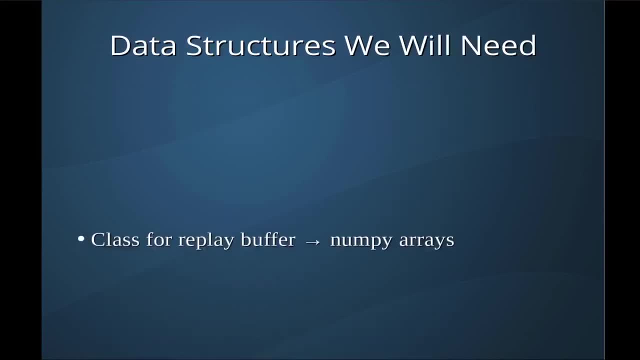 we're only we're only going to be performing this update when we update the actor network, so it's not every time step in this case, it'll be every other time step very, very important. so for this program we're gonna need a number of data structures. 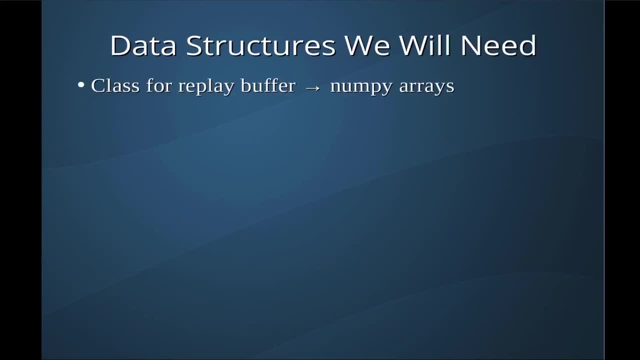 we're gonna need a class for our replay buffer, the agents memory. now I like to use numpy arrays. it is not the best way or the only way to do it, it's just my preferred way. so follow along with me in the tutorial, do it that way and then 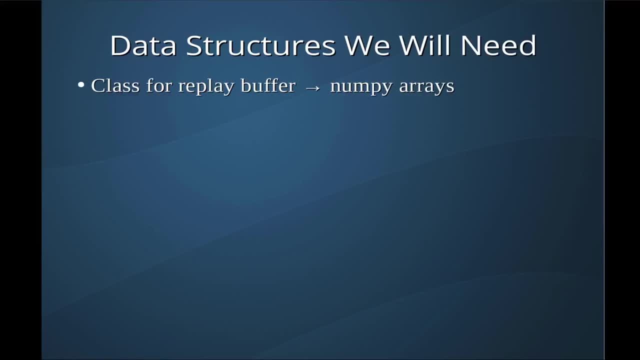 when you play around with the code later to understand it better, go ahead and rewrite the replay buffer to something that makes more sense to you. that's a great way to get started with. modifying the program is with the replay buffer. next we're gonna have classes for our actor network and our critic network, and those 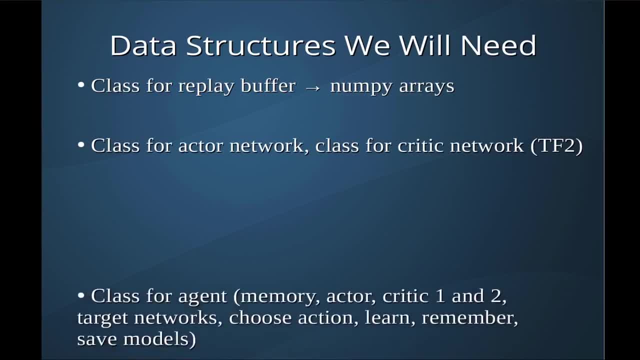 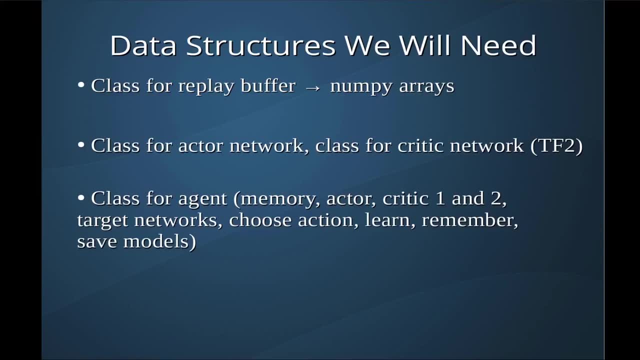 are, of course, written in tensorflow too. we'll have another class for our agent, and that is really gonna tie everything together. it's gonna have a memory that keeps track of transitions. it's gonna have an actor, two critics, target networks- for each of those a function to choose a. 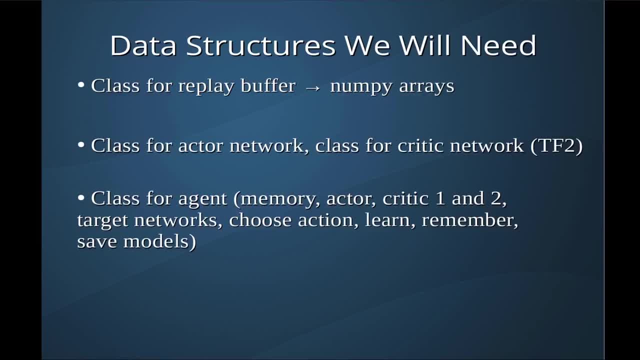 function based on the current state, a function to learn, that performs the update rules. we just went over an interface function with its memory that I call remember, just to store transitions in the agents memory, as well as functionality to save models and perform target network updates, which I forgot to. 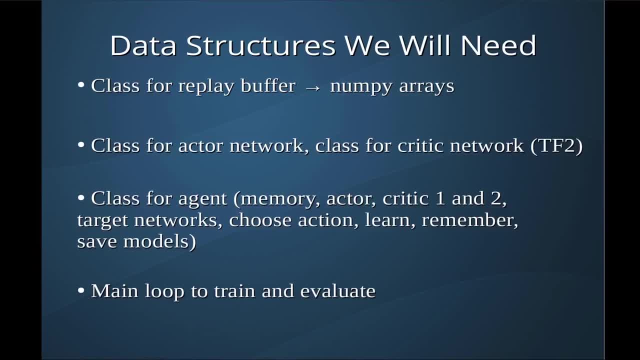 write here. finally, we're gonna need a main loop to train and evaluate our algorithm. so we're gonna be using the open AI gym in the bipedal Walker in particular, because this is a kind of difficult environment for other algorithms. it's a continuous action space with a pretty 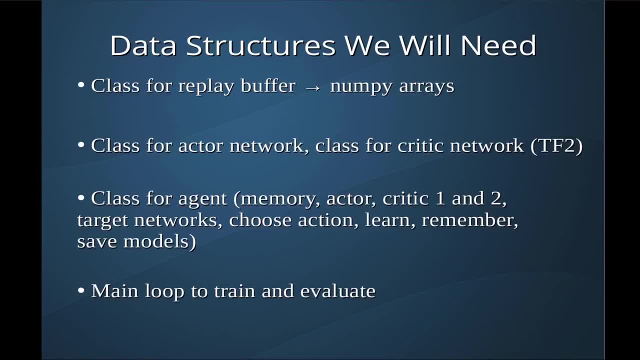 large state space. I think it has 24 different components in the state space, if I'm not mistaken. some are all to be large number. so it's a bit difficult for agents to learn and in fact it's gonna take my computer around six or seven hours to complete the evaluation. I'm filming this after I do the code, so 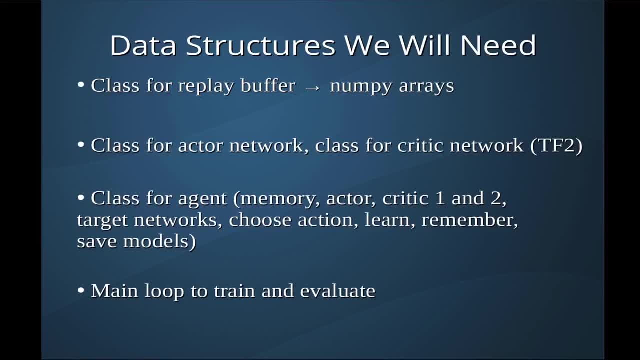 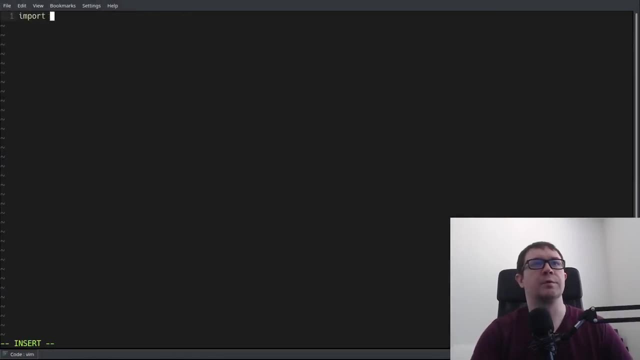 it'll take a while to run. so if it takes forever on your computer, don't don't panic. that's normal, quite normal. so all that out of the way, let's go ahead and get started in the coding portion of this tutorial. all right, so we begin, as usual, with our imports. we will 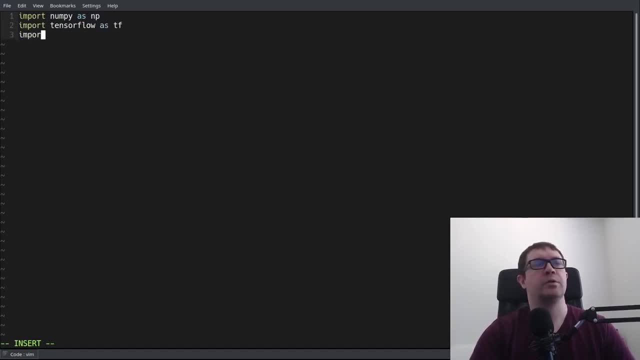 need numpy, the base tensorflow package, we will need tensorflow dot keras, we will need layers from- yeah, important- dense, that is for constructing our deep neural networks, and then we'll need the code that we're going to use for the model and we will need our atom optimizer or the gradient descent, and we 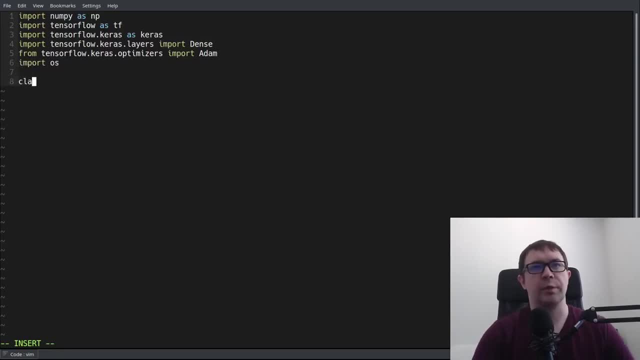 will need OS for file joining operations, for model checkpointing. let's start with our replay buffer class now. this should be very familiar to you. for deep used to a deep Q learning, we'll need a max size, input, shape and number of actions as input to our constructor. so we're going to need a max size, input, shape and number of actions as input to our constructor. so we'll need a. 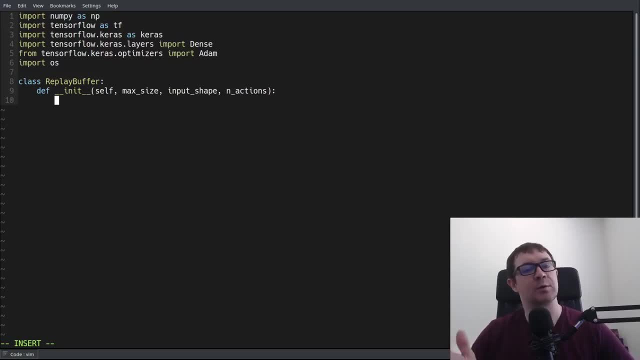 max size, input shape and number of actions as input to our constructor. so we'll need a- now remember we're dealing with continuous action spaces, so this number. now remember we're dealing with continuous action spaces, so this number. now remember we're dealing with continuous action spaces, so this number of actions is really a number of components. 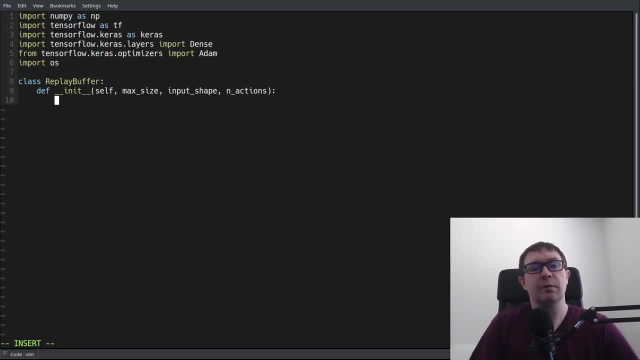 of actions is really a number of components of actions is really a number of components to our continuous action. I just name it to our continuous action. I just name it to our continuous action. I just name it that for consistency with my deep Q. that for consistency with my deep Q. 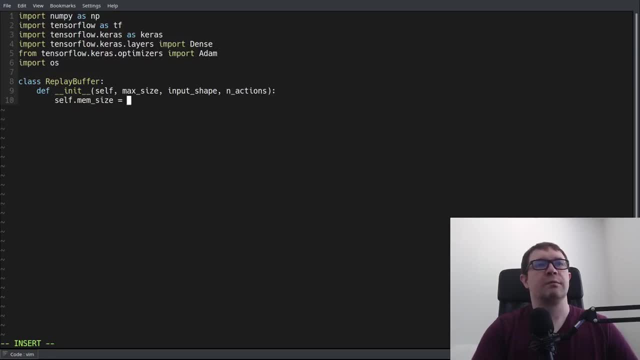 that, for consistency with my deep Q learning code. so we will save the learning code. so we will save the learning code. so we will save the appropriate member variables. we use a appropriate member variables. we use a appropriate member variables. we use a memory counter instantiated at zero. 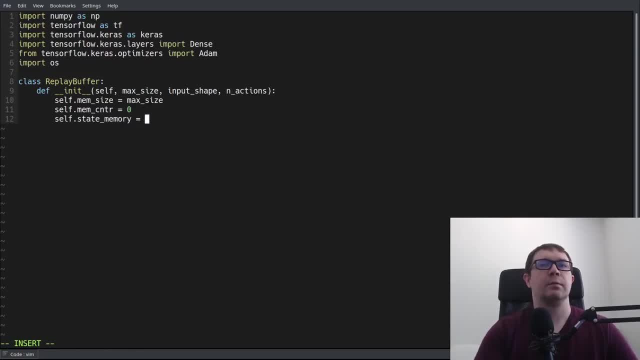 memory counter instantiated at zero. memory counter instantiated at zero. because our memory is finite, we'll need, because our memory is finite, we'll need, because our memory is finite, we'll need our state memory, which will initialize our state memory, which will initialize our state memory, which will initialize as zeros in the shape, mem size and star. 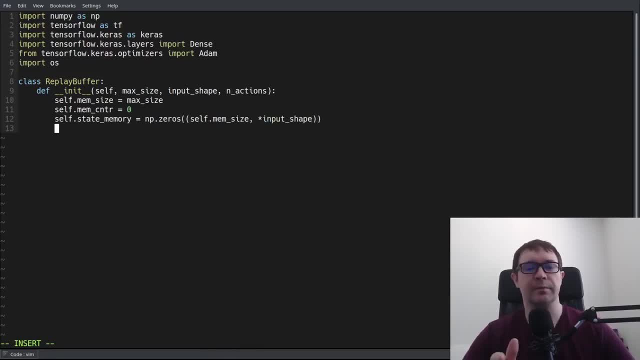 as zeros in the shape, mem, size and star as zeros in the shape, mem, size and star input shape. the star idiom just unpacks input shape. the star idiom just unpacks input shape. the star idiom just unpacks a, an array. in this case, whatever the 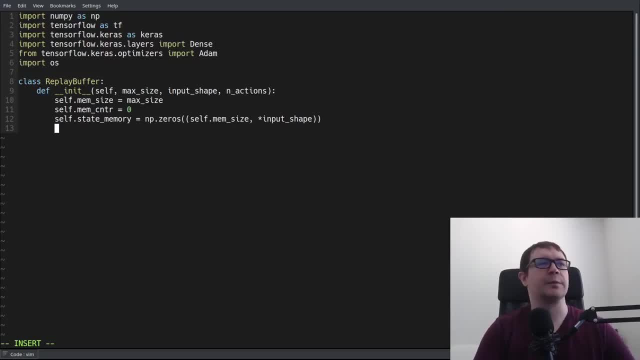 a an array in this case. whatever the a an array in this case. whatever the shape of our input, dimensionality is from shape of our input. dimensionality is from shape of our input. dimensionality is from our environment. we'll, of course, need a our environment. we'll of course need a. 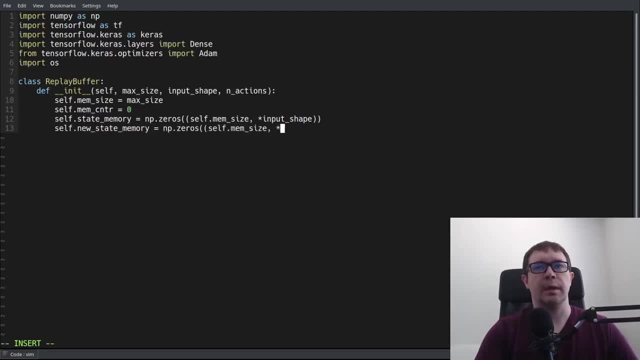 our environment. we'll, of course, need a new state memory. and that's the same new state memory. and that's the same new state memory and that's the same shape that keeps track of the new states. shape that keeps track of the new states. shape that keeps track of the new states that we are going to see an action. 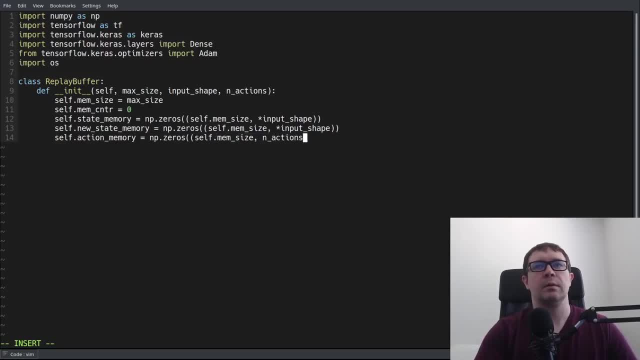 that we are going to see an action, that we are going to see an action, memory and remember of course again, memory and remember of course again memory and remember of course again. number of actions is number of number of actions is number of number of actions is number of components to or action reward memory in. 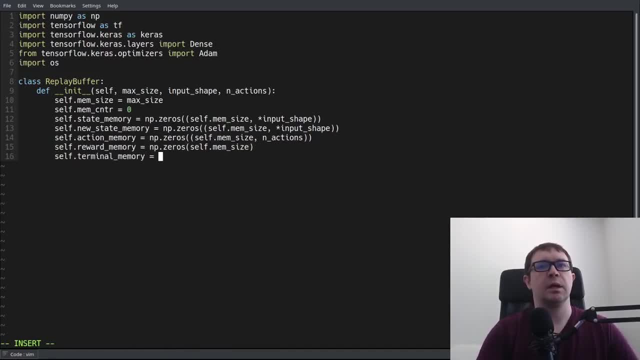 components to or action reward memory in components to or action reward memory in the shape of memory size and a terminal. the shape of memory size and a terminal. the shape of memory size and a terminal memory. we're going to use numpy, numpy, numpy bool as our data type. that'll keep. we're going to use numpy, numpy, numpy, numpy, bool as our data type that'll keep track of our terminal flags. the reason: track of our terminal flags. the reason: track of our terminal flags? the reason being that, the value of the terminal being that the value of the terminal, 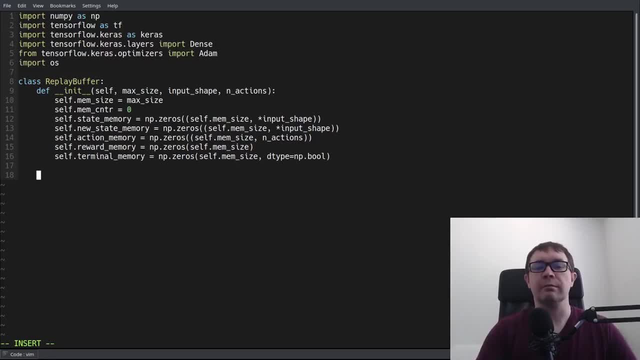 being that the value of the terminal state is always zero, and so we keep state is always zero, and so we keep state is always zero, and so we keep track of the done flags from our track of the done flags, from our track of the done flags from our environment to accommodate that. so let's 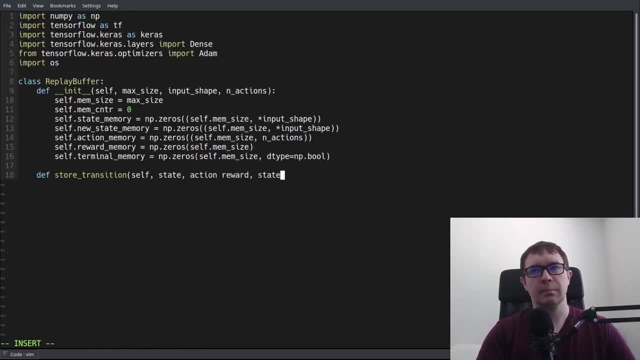 environment to accommodate that. so let's environment to accommodate that. so let's store a transition that takes the state store, a transition that takes the state store, a transition that takes the state observed. action taken- reward received. observed action taken- reward received. observed action taken- reward received. new state observed and terminal flag. 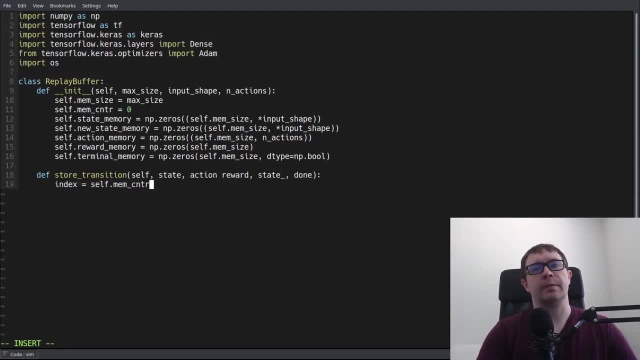 new state observed and terminal flag. new state observed and terminal flag received as input. we want to know what received as input. we want to know what received as input. we want to know what the first available memory position is. the first available memory position is, the first available memory position is, and that's memory counter modules, mem. 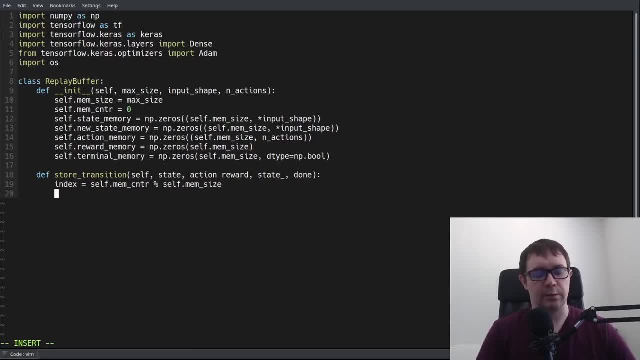 and that's memory counter modules, mem. and that's memory counter modules, mem. size: that is a property that it will size. that is a property that it will size. that is a property that it will overwrite earlier memories with newer, overwrite earlier memories with newer, overwrite earlier memories with newer memories, as soon as the memory fills up. 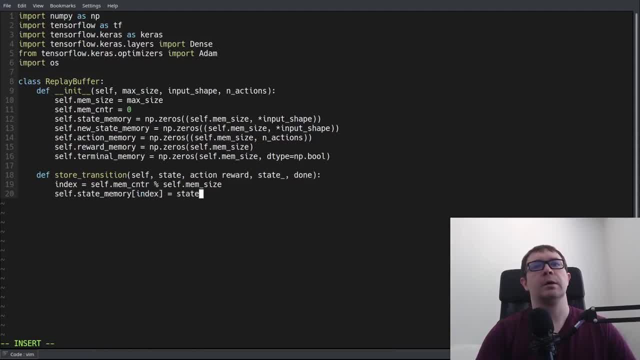 memories as soon as the memory fills up, memories as soon as the memory fills up, and then go ahead and save our and then go ahead and save our and then go ahead and save our. variables will state: underscore variables will state: underscore variables will state underscore: terminal memory and that's all of them. I. 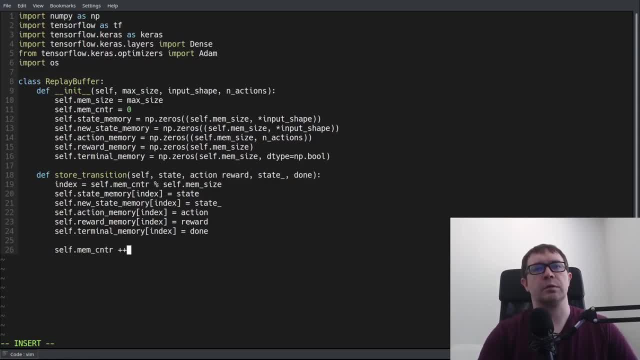 terminal memory and that's all of them. I terminal memory and that's all of them. I believe, and very important, we want to believe, and very important, we want to believe, and very important, we want to increment our memory counter by one next. increment our memory counter by one next. 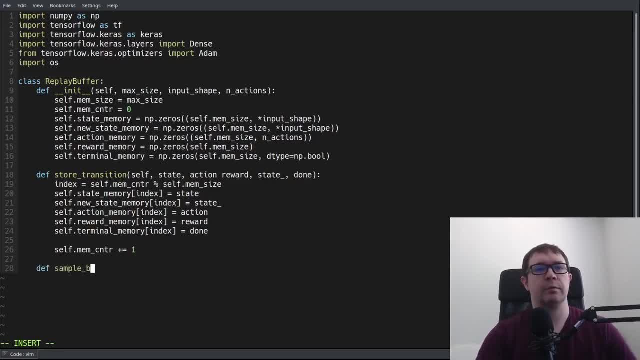 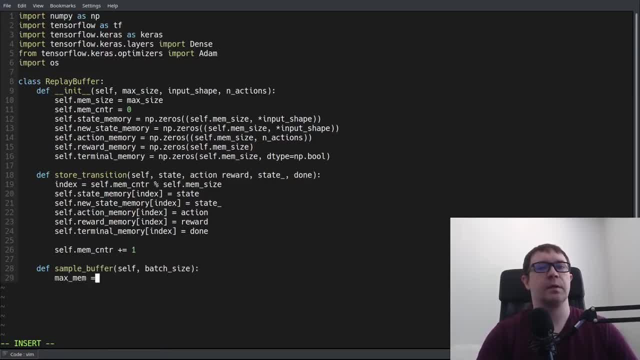 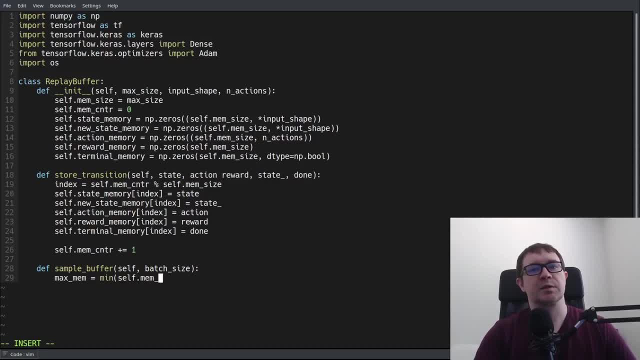 input. we want to know what the position input. we want to know what the position of our maximum field of memory is and of our maximum field of memory is and of our maximum field of memory is, and that's given by this minimum of mem. that's given by this minimum of mem. 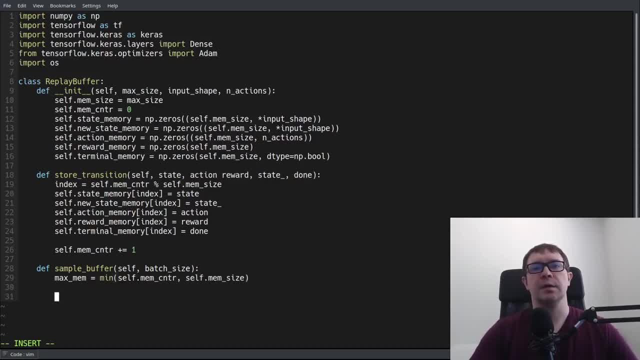 that's given by this minimum of mem counter and mem size. because we don't counter and mem size, because we don't counter and mem size, because we don't want to sample zeros, we initialize, want to sample zeros. we initialize, want to sample zeros, we initialize the memory with zero, so we just sample the. 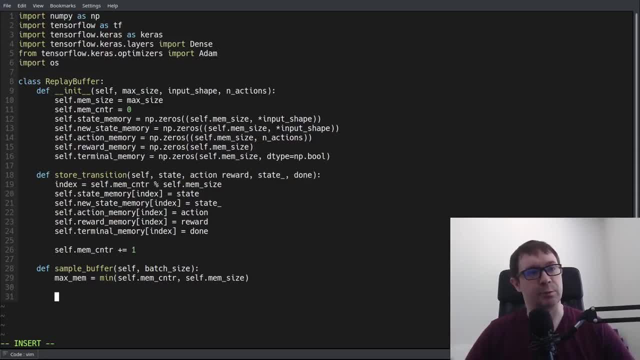 the memory with zero, so we just sample the the memory with zero, so we just sample the entire buffer. then we were probably entire buffer, then we were probably entire buffer, then we were probably going to end up sampling zeros until we going to end up sampling zeros until we 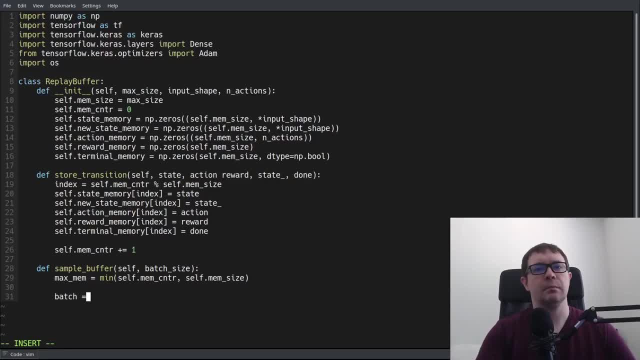 going to end up sampling zeros until we fill up that buffer which is totally fill up that buffer which is totally fill up, that buffer which is totally useless, useless, useless. so then the batch is going to be a. so then the batch is going to be a. so then the batch is going to be a random choice. 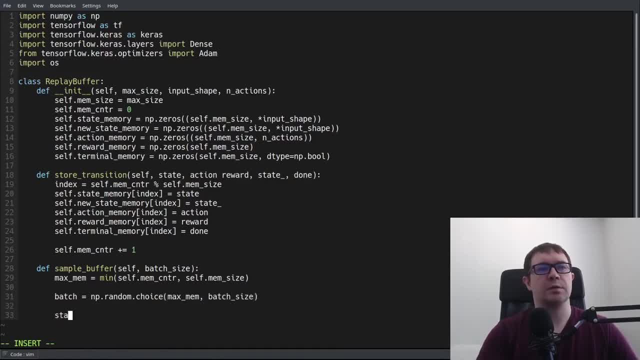 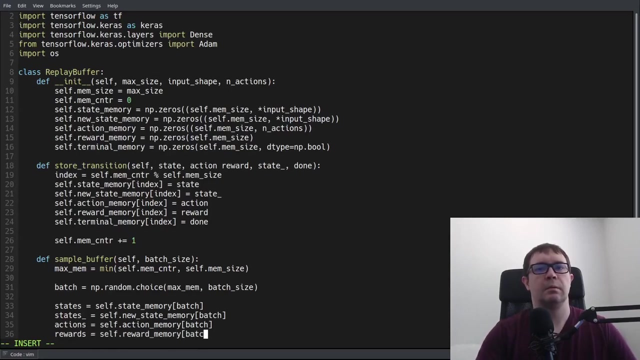 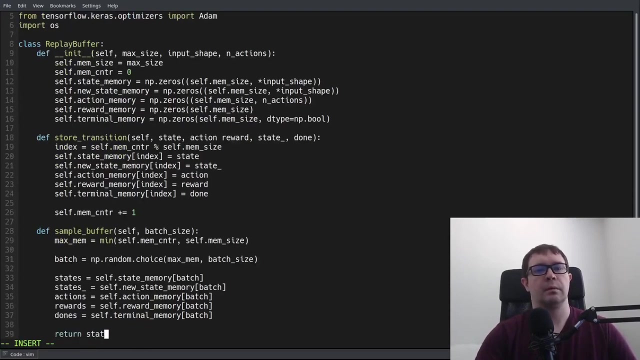 random choice. random choice: from zero to maximum in shape batch. from zero to maximum in shape batch. from zero to maximum in shape batch size. then go ahead and dereference. then go ahead and dereference, then go ahead and dereference our variables and and and duns. 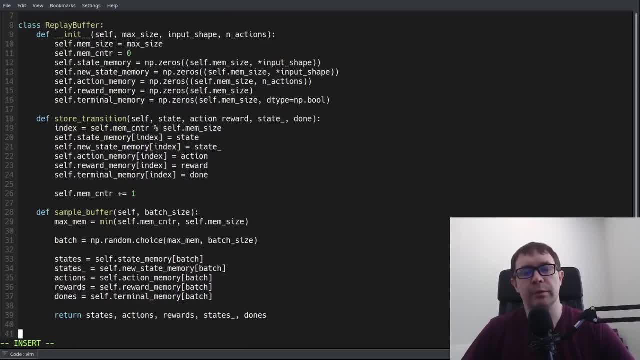 all right, that wraps up our replay. all right, that wraps up our replay. all right, that wraps up our replay. memory, that's very, very simple. uh, memory, that's very, very simple. uh, memory, that's very, very simple. uh, probably the most straightforward class, probably the most straightforward class. 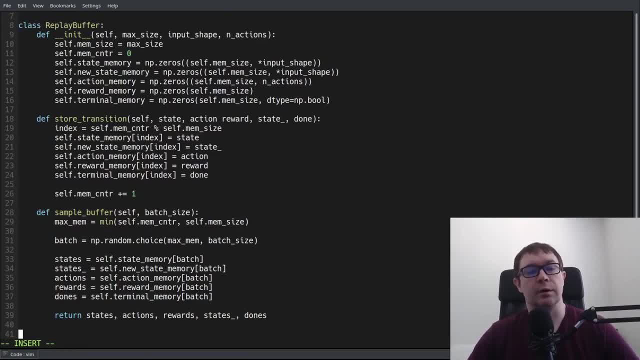 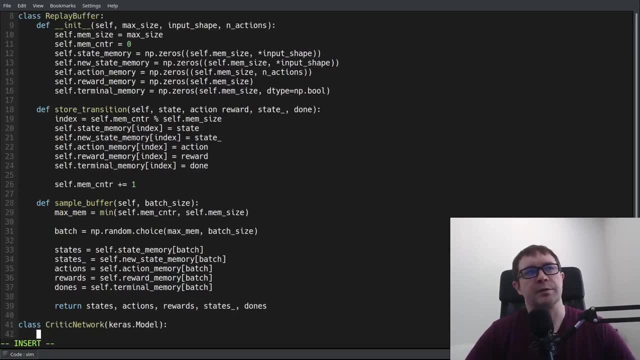 probably the most straightforward class in the entire project, in the entire project, in the entire project. next, we're going to move on to our next, we're going to move on to our next, we're going to move on to our critic network, critic network, critic network, and that will derive from charismodel. 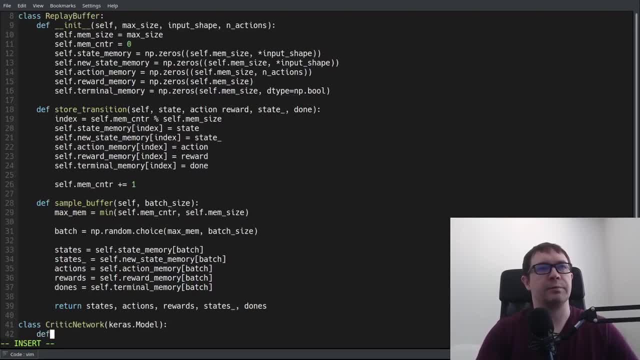 and that will derive from charismodel and that will derive from charismodel. so we get access to all of the. so we get access to all of the. so we get access to all of the properties of that particular base, properties of that particular base, properties of that particular base class. 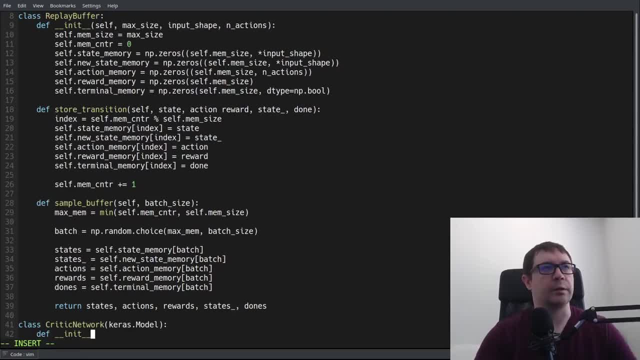 class class that'll help with using the gradient. that'll help with using the gradient. that'll help with using the gradient tape for learning, tape for learning, tape for learning later on. we're going to take some. we're going to take some. we're going to take some inputs for the number of dimensions for 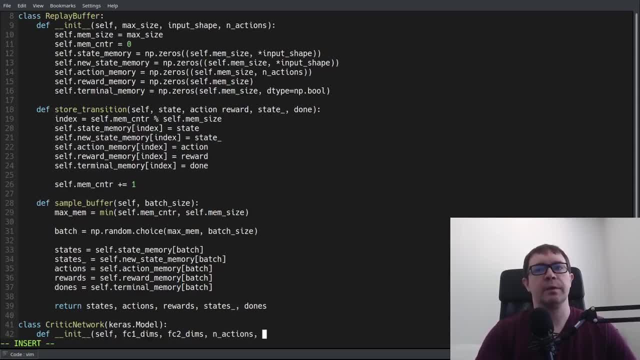 inputs for the number of dimensions, for inputs for the number of dimensions for the first and second. the first and second. the first and second. second fully connected layers. second fully connected layers. second fully connected layers. number of actions again. number of number of actions again. number of number of actions again. number of components: 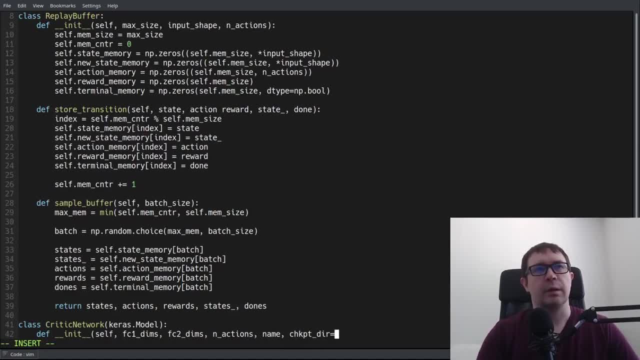 components, components, a name for the purpose of model, a name for the purpose of model, a name for the purpose of model, checkpointing, checkpointing, checkpointing and a checkpoint directory and a checkpoint directory and a checkpoint directory. we will have to do, we will have to do. 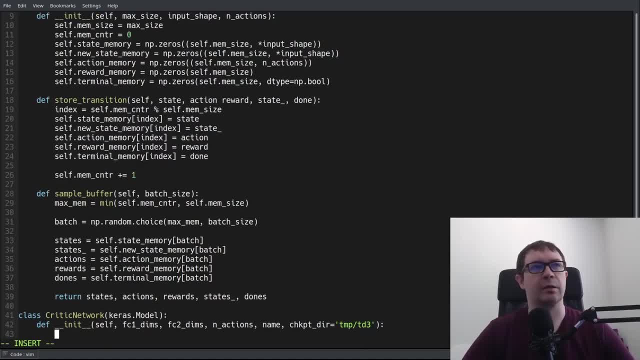 we will have to do a make directory on that before you, a make directory on that before you, a make directory on that before you begin, otherwise you will get an error. begin, otherwise you will get an error. begin, otherwise you will get an error and it will not. 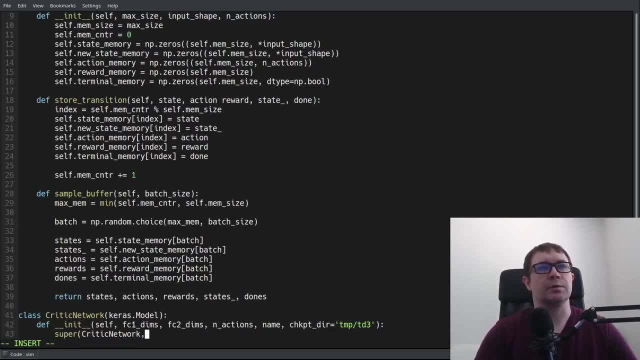 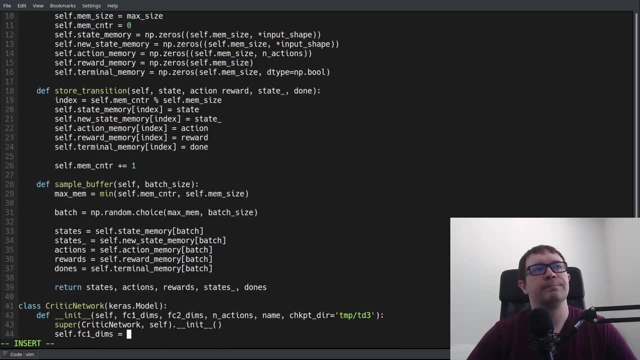 and it will not and it will not work. let's call our super constructor work. let's call our super constructor work. let's call our super constructor and start saving stuff. and start saving stuff. and start saving stuff. do i need to do that? do i need to do that? 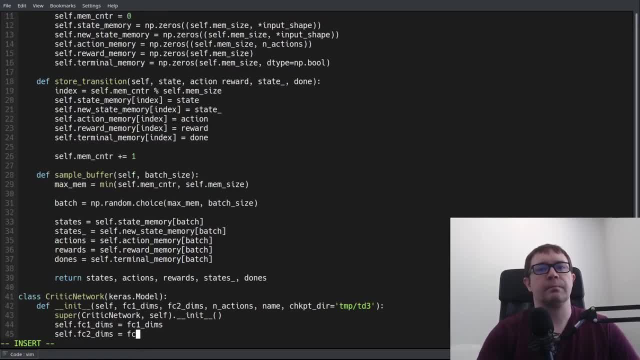 do i need to do that? yeah, why not? so the purpose of the name is the fact that the purpose of the name is the fact that the purpose of the name is the fact that, um, we're going to be saving target. um, we're going to be saving target. 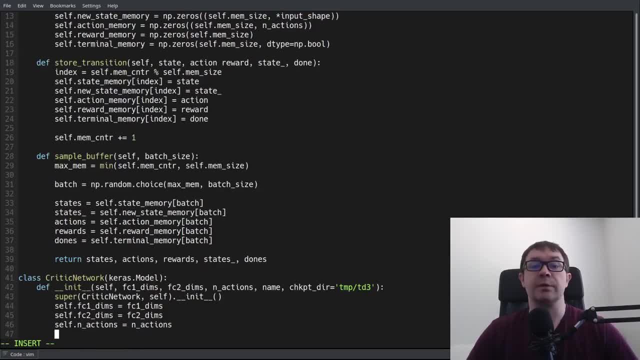 um, we're going to be saving target networks as well as networks, as well as networks as well as regular networks, and they're going to be regular networks and they're going to be regular networks and they're going to be two critics. so we want to be able to 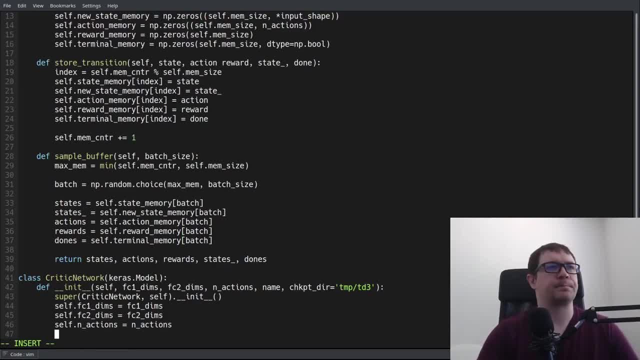 two critics, so we want to be able to two critics, so we want to be able to keep all of those straight. when we keep all of those straight, when we keep all of those straight when we handle model checkpointing, so we'll save our model name. so we'll save our model name. 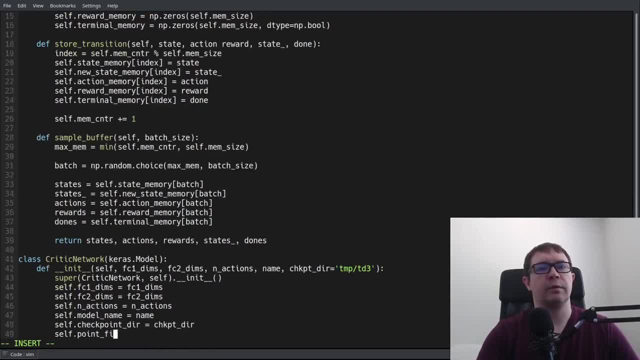 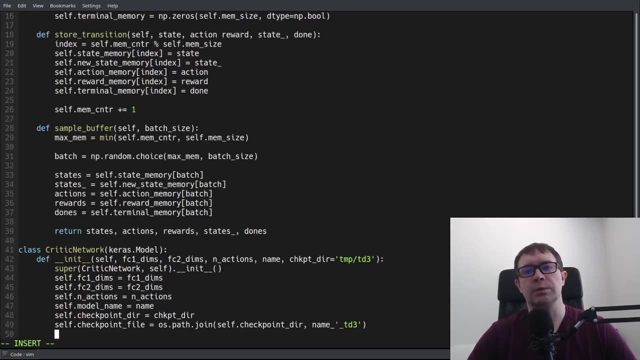 so we'll save our model name, checkpoint directory, checkpoint directory, checkpoint directory and the checkpoint file and i like to append the algorithm name and i like to append the algorithm name and i like to append the algorithm name to the checkpoint file so that, if i do, to the checkpoint file, so that, if i do, 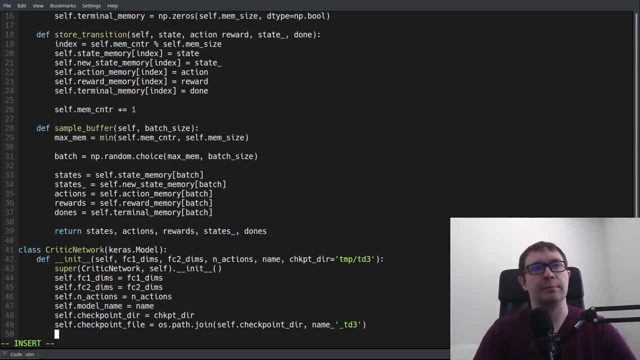 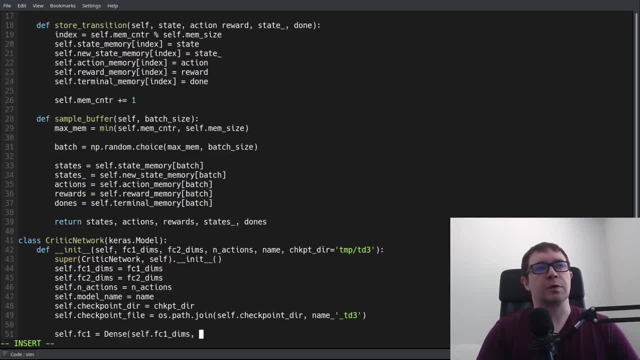 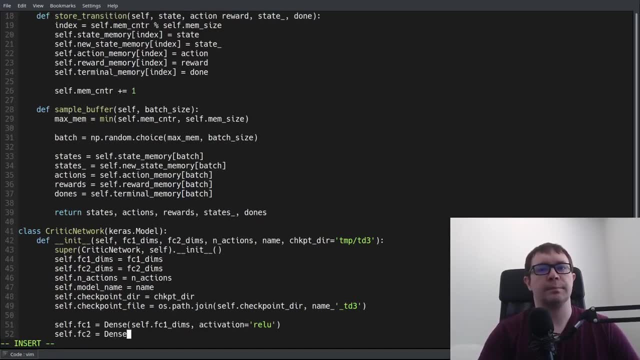 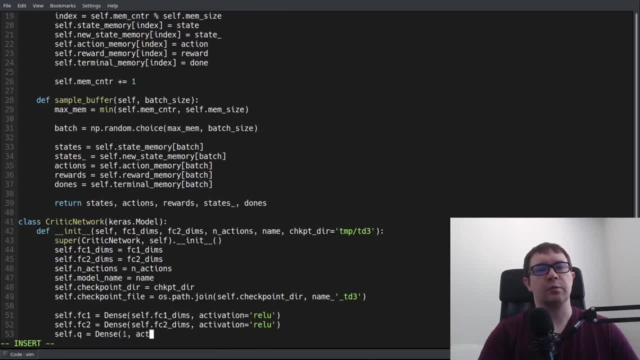 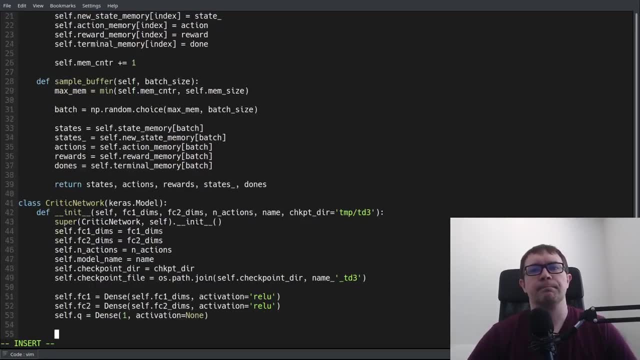 second dense layer with value activation, second dense layer with value activation and an output and an output, and an output that will be single valued with no. that will be single valued with no. that will be single valued with no activation. now keep in mind one interesting thing. now keep in mind one interesting thing. 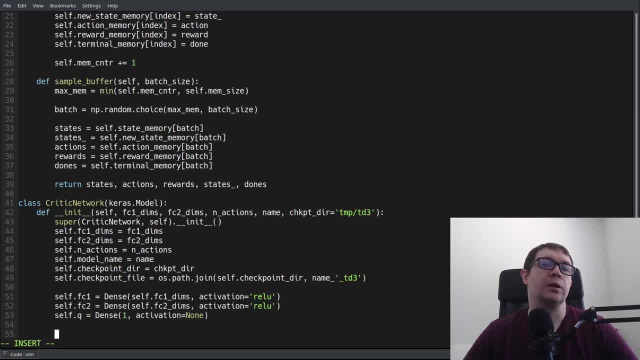 now keep in mind. one interesting thing about about about tensorflow 2 is that we don't have to tensorflow 2 is that we don't have to. tensorflow 2 is that we don't have to specify the number of input dimensions. it specify the number of input dimensions. it. 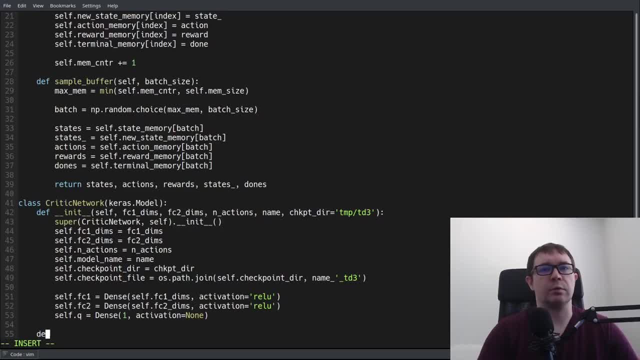 specify the number of input dimensions. it infers it from the inputs. that's a infers it from the inputs. that's a infers it from the inputs. that's a pretty nice feature. so now we define our pretty nice feature. so now we define our pretty nice feature. so now we define our feed forward. in this case, we call it. 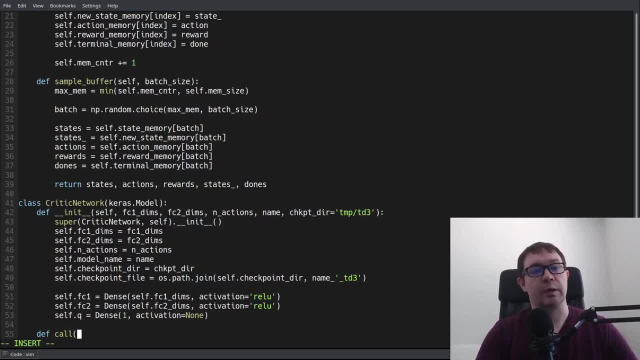 feed forward. in this case, we call it feed forward. in this case, we call it call that allow us to use the name of an call. that allow us to use the name of an call. that allow us to use the name of an object as a function call. basically need: 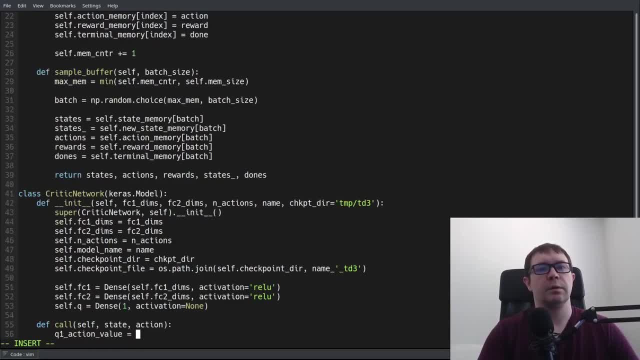 object as a function call. basically need object as a function call. basically need a state in action as input. we'll have a a state in action as input. we'll have a a state in action as input. we'll have a q1 action value and we will want to. 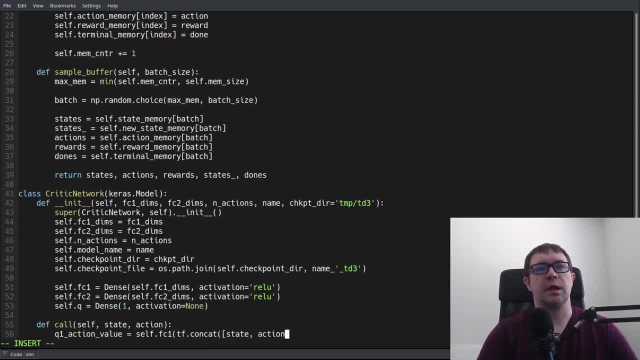 q1 action value and we will want to q1 action value and we will want to concatenate our state and action along, concatenate our state and action along, concatenate our state and action along the first axis, and we will feed that, the first axis, and we will feed that. 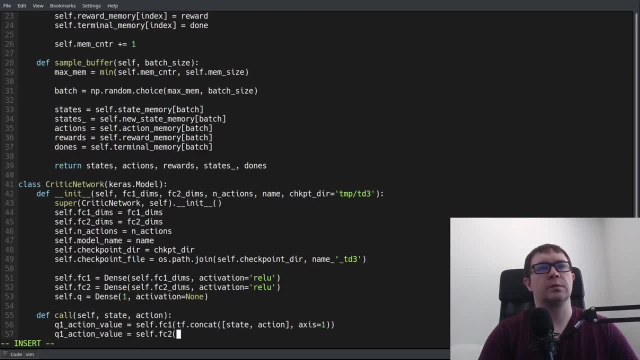 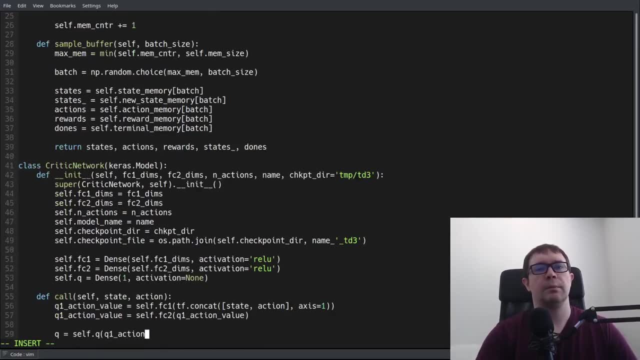 the first axis and we will feed that through FC to q1 action value and then through FC to q1 action value and then through FC to q1 action value and then pass it through the final layer action, pass it through the final layer action, pass it through the final layer action value and return. now, keep in mind, 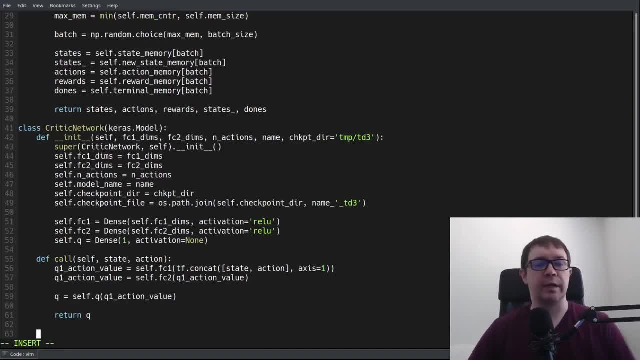 value and return now. keep in mind value and return now. keep in mind that the critic evaluates the value of that. the critic evaluates the value of that. the critic evaluates the value of both the action and state. so that's why, both the action and state. so that's why. 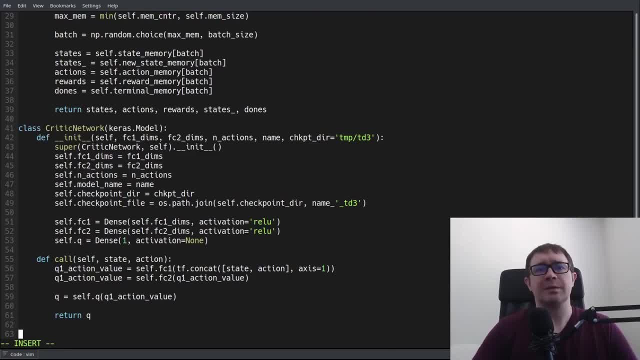 both the action and state. so that's why we have to concatenate the two values. we have to concatenate the two values. we have to concatenate the two values. that is it for our critic Network. very, that is it for our critic Network. very, that is it for our critic Network. very, very straightforward. next, we're gonna. 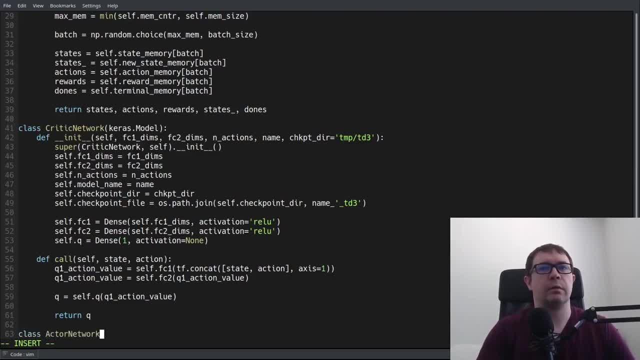 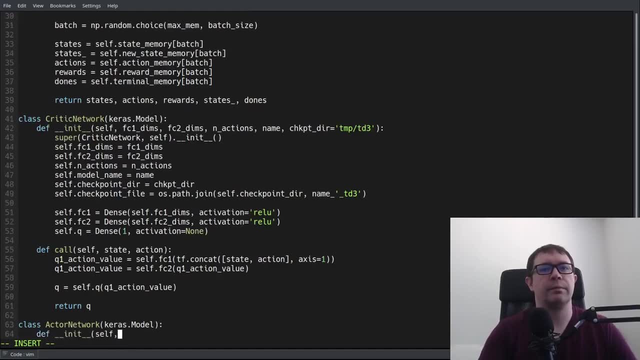 very straightforward. next, we're gonna very straightforward. next we're gonna handle our actor network. and that again, handle our actor network. and that again handle our actor network. and that again derives from Karis dot model. just the derives from Karis dot model, just the derives from Karis dot model, just the same as the critic network, our. 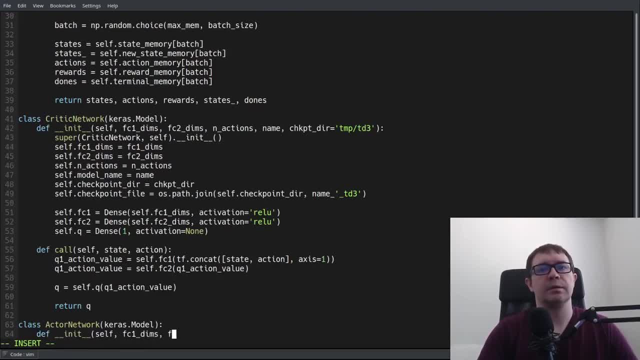 same as the critic network. our same as the critic network, our initializer takes dimensionality as initializer, takes dimensionality as initializer, takes dimensionality as input again as well. number of actions- input again as well. number of actions, input again as well. number of actions. and you know what did I? I'm sorry, I'm. 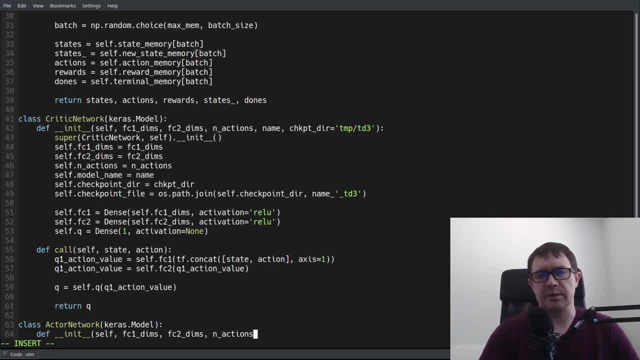 and you know what did I. I'm sorry I'm, and you know what did I? I'm sorry I'm checking something here. no, I did not for checking something here. no, I did not for checking something here. no, I did not for a second there. I thought I passed in. 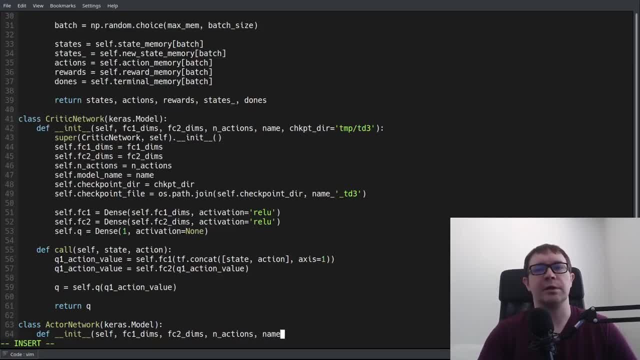 a second there. I thought I passed in a second there. I thought I passed in input shape to the critic network, that input shape to the critic network, that input shape to the critic network. that would have been totally unnecessary, would have been totally unnecessary, would have been totally unnecessary. checkpoint directory equals temp td3 we. 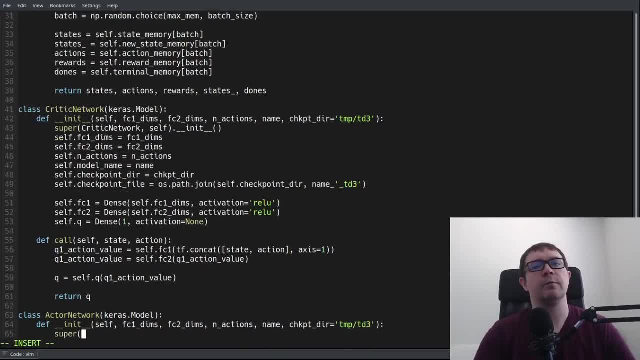 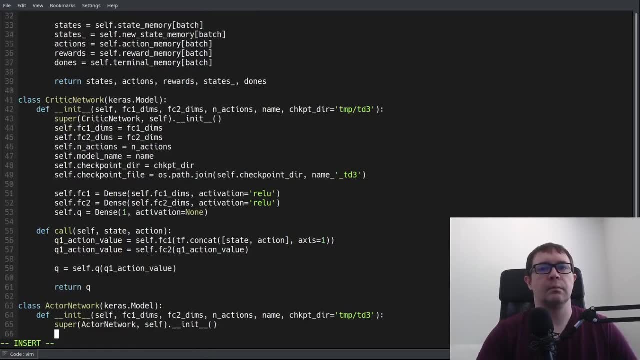 checkpoint directory equals temp td3. we checkpoint directory equals temp td3. we want all of the models to live in the want all of the models to live in the want all of the models to live in the same directory. very, very helpful, and then we can go ahead and start saving. 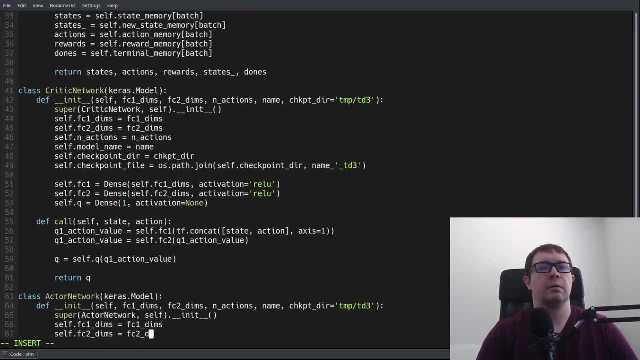 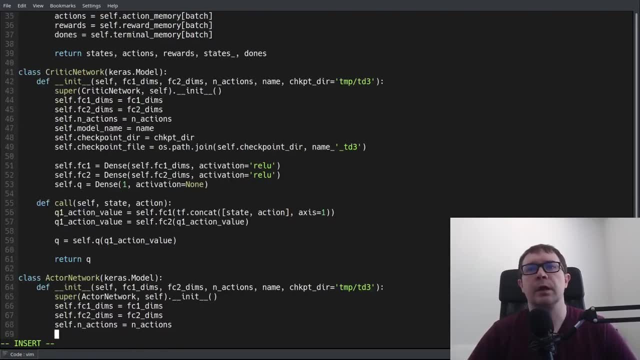 then we can go ahead and start saving. then we can go ahead and start saving stuff. I'm looking at this and as I look stuff, I'm looking at this and as I look stuff, I'm looking at this and as I look at the, what I'm doing here. so I like 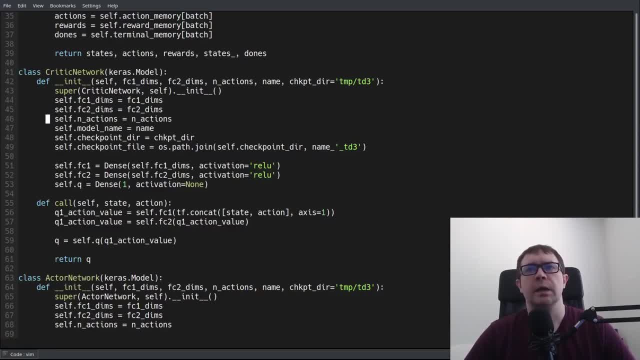 at the what I'm doing here, so I like at the what I'm doing here, so I like to modify stuff on the fly. I don't think I to modify stuff on the fly. I don't think I to modify stuff on the fly, I don't think I actually need this and actions here. so 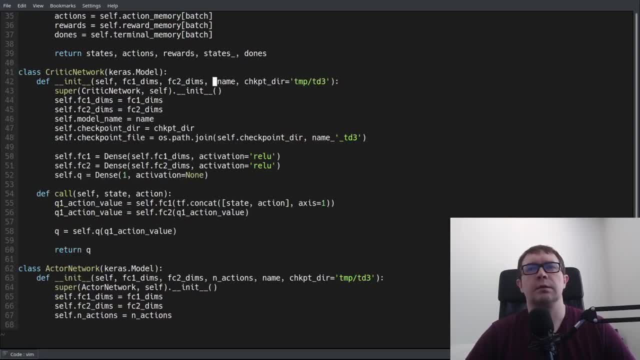 actually need this and actions here. so actually need this and actions here. so let's go ahead and delete that, just for. let's go ahead and delete that, just for. let's go ahead and delete that, just for the sake of cleanliness. we will need it, the sake of cleanliness, we will need it. 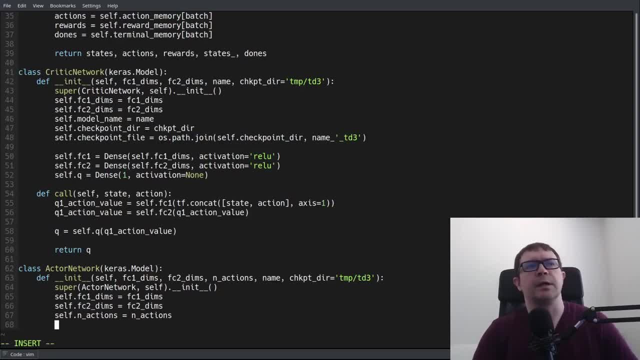 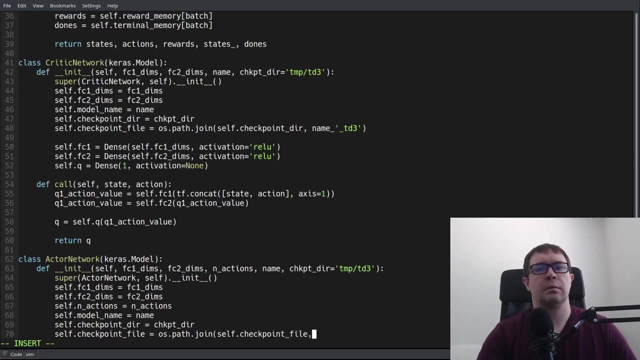 the sake of cleanliness, we will need it in the actor. of course, yeah, let's keep in the actor. of course. yeah, let's keep in the actor. of course, yeah, let's keep it nice and clean. model name it nice and clean. model name it nice and clean. model name checkpoint directory plus td3 and just. 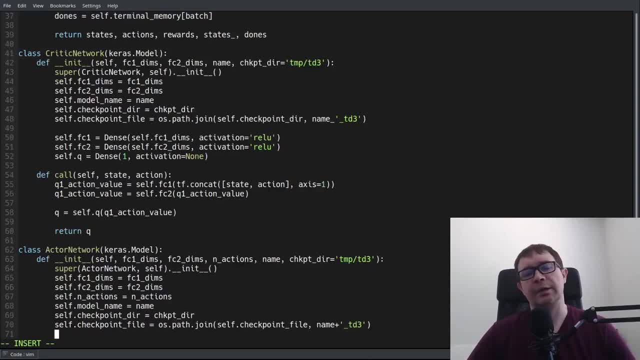 checkpoint directory plus td3 and just checkpoint directory plus td3. and just for clarity, that name will have stuff for clarity. that name will have stuff for clarity. that name will have stuff like target actor, target critic actor, or like target actor, target critic actor, or like target actor, target critic actor or critic. so we can keep all of those. 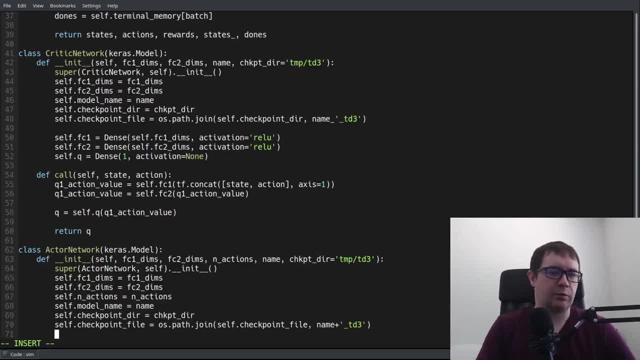 critic, so we can keep all of those critic, so we can keep all of those particular networks straight and of particular networks straight and of particular networks straight. and of course the two critics will be critic, course the two critics will be critic, course the two critics will be critic one or critic two, because we have some. 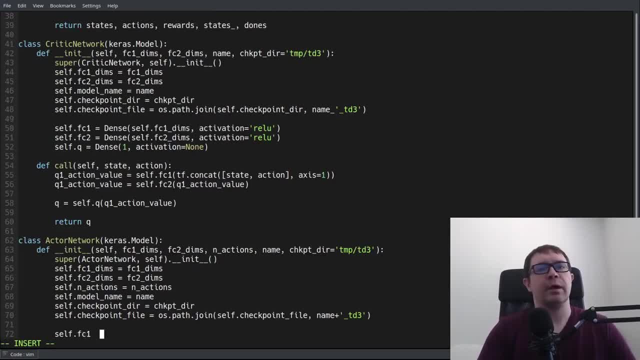 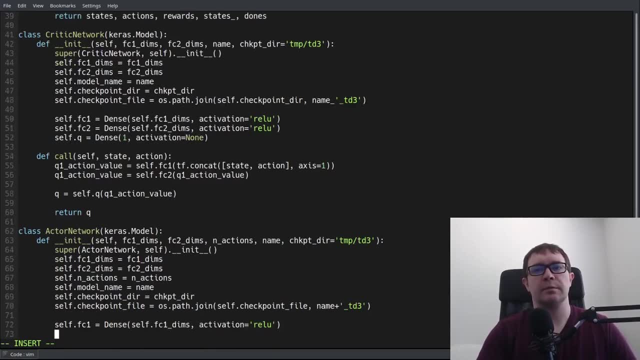 one or critic two because we have some one, or critic two because we have some very interesting naming conventions. so now, very interesting naming conventions. so now very interesting naming conventions. so now we'll have our deep neural network. we'll have our deep neural network, we'll have our deep neural network- again a simple dense layer with value. 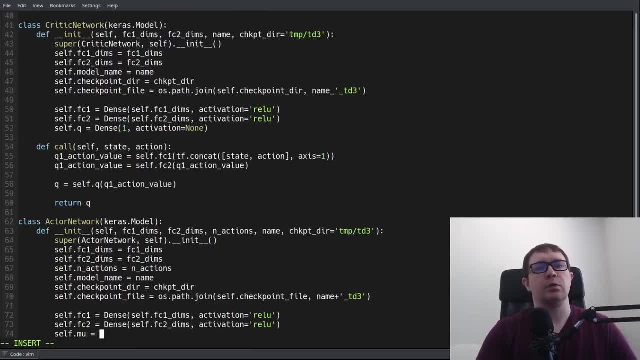 again a simple dense layer with value. again a simple dense layer with value. activations for the first two layers and activations for the first two layers, and activations for the first two layers, and then mu for our output, and that will then mu for our output, and that will. 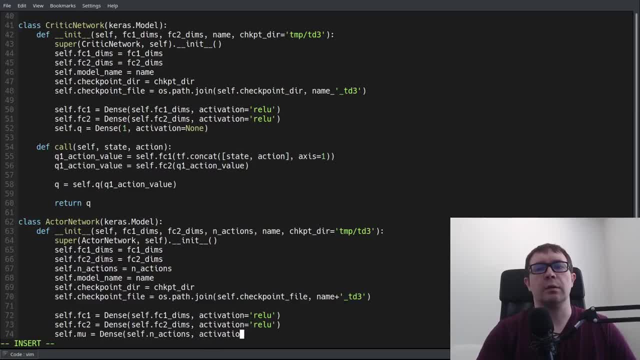 then mu for our output, and that will take an actions as our output, take an actions as our output, take an actions as our output. dimensionality with a tan hyperbolic dimensionality with a tan hyperbolic dimensionality with a tan hyperbolic activation, the tan hyperbolic is bound. activation: the tan hyperbolic is bound. activation: the tan hyperbolic is bound between minus 1 and plus 1. if you want between minus 1 and plus 1. if you want between minus 1 and plus 1. if you want to take into account. to take into account. to take into account boundaries of actions that are beyond plus boundaries of actions that are beyond plus boundaries of actions that are beyond plus or minus 1. you can multiply this or minus 1. you can multiply this or minus 1. you can multiply this output by the maximum balance for your. 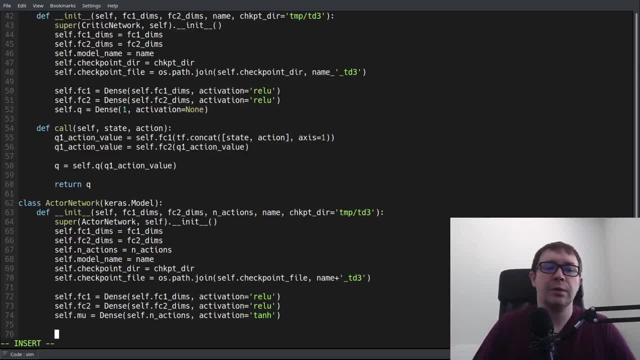 output by the maximum balance for your output, by the maximum balance for your environment. so some environments, all the environment. so some environments, all the environment, so some environments. all the max action of plus or minus 2? which of max action of plus or minus 2? which of 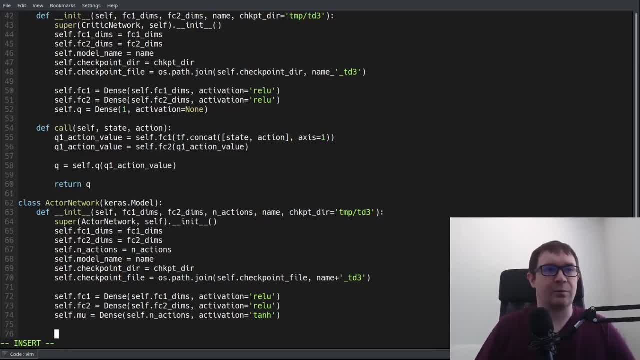 max action of plus or minus 2, which, of course, plus or minus 1 is oftentimes course. plus or minus 1 is oftentimes course plus or minus 1 is oftentimes less than you know. 2, so you have to take. less than you know 2, so you have to take. 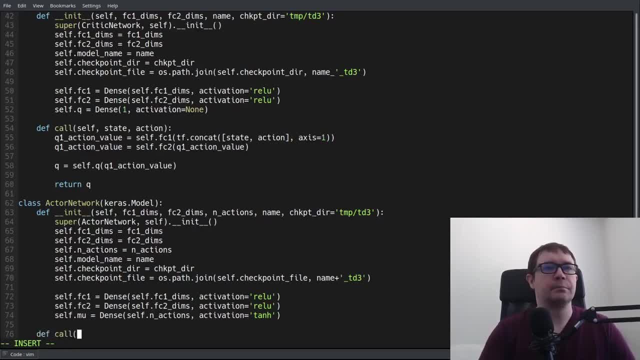 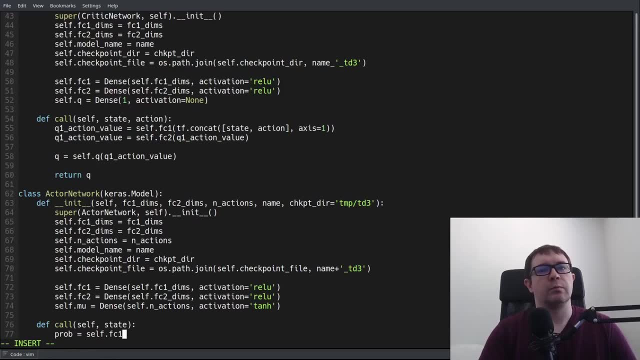 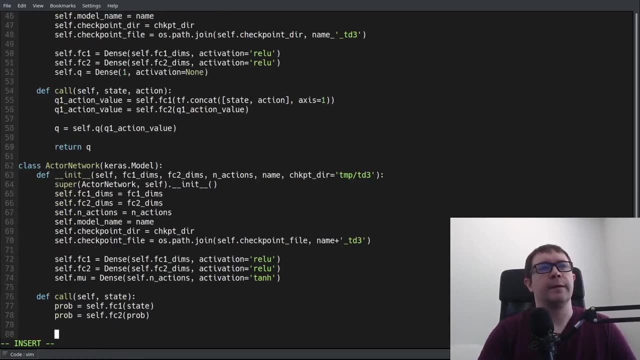 less than you know. 2, so you have to take that into account, depending on the, that into account, depending on the that into account, depending on the environment. so again, we need a call state through the first fully connected state, through the first fully connected state, through the first fully connected layer, second fully connected layer and 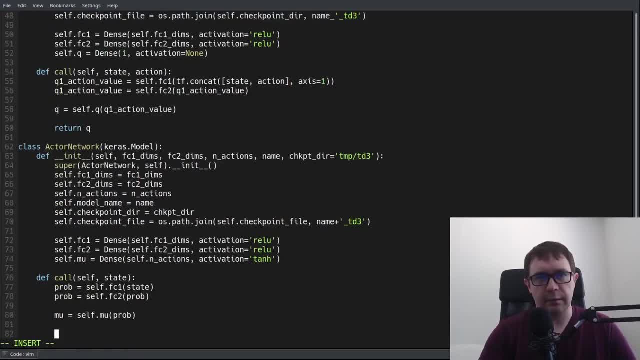 layer second fully connected layer and layer second fully connected layer and pass that through the final layer and pass that through the final layer and pass that through the final layer and return it. so that is it for our actor, return it. so that is it for our actor. 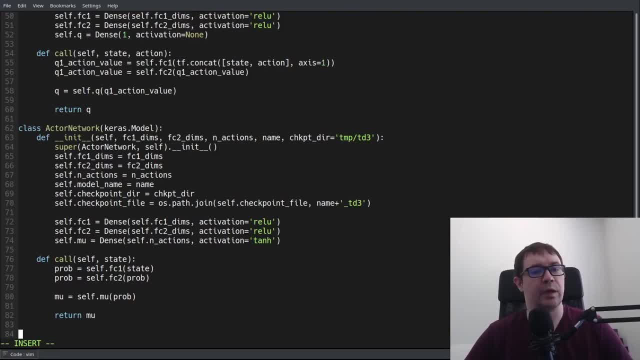 return it. so that is it for our actor network. next we need an agent class, that network. next we need an agent class that network. next we need an agent class that I, everything together and to handle all I, everything together, and to handle all I, everything together and to handle all of the really interesting functionality. 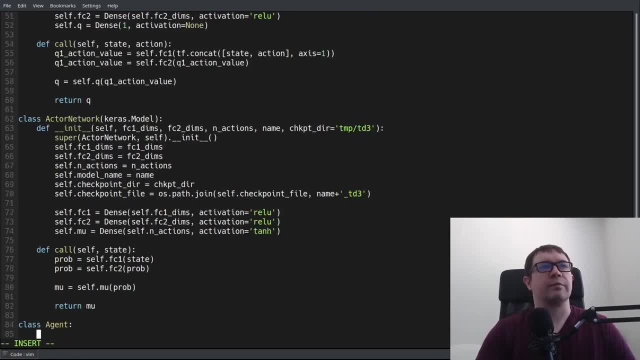 of the really interesting functionality, of the really interesting functionality. so our agent doesn't derive from. so our agent doesn't derive from. so our agent doesn't derive from anything but our anything. but our agent doesn't derive from anything. but our agent doesn't derive from our super constructor, excuse me, our 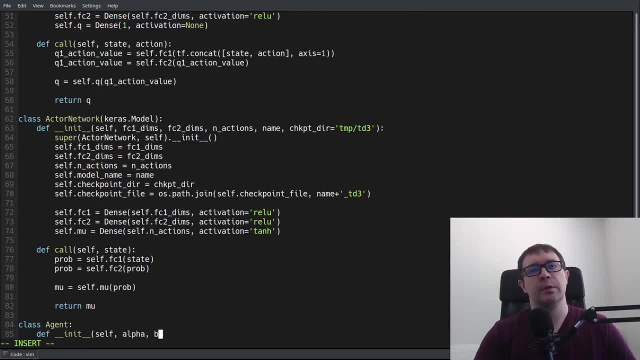 our super constructor, excuse me, our, our super constructor, excuse me, our constructor is going to take a whole slew. constructor is going to take a whole slew. constructor is going to take a whole slew of inputs. so we need a couple of inputs. so we need a couple of inputs. so we need a couple different learning rates. reason being: you. 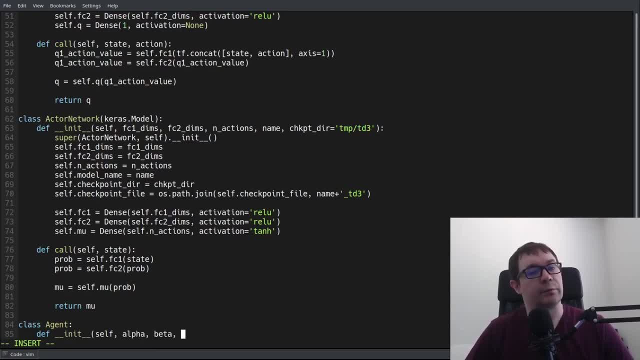 different learning rates. reason being: you different learning rates. reason being: you want to accommodate the capacity for want to accommodate the capacity for want to accommodate the capacity for different learning rates for your actor, different learning rates for your actor, different learning rates for your actor and critic networks. sometimes they learn. 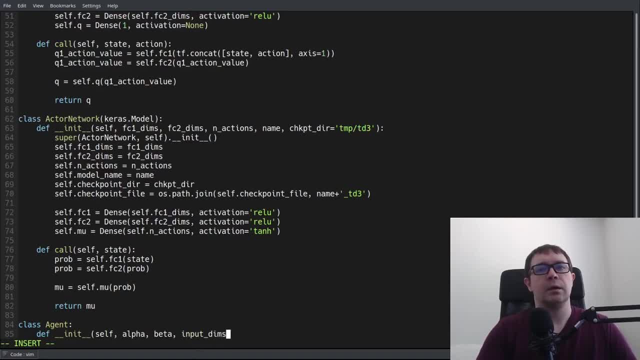 and critic networks: sometimes they learn and critic networks: sometimes they learn best with different learning rates input: best with different learning rates input. best with different learning rates input dims: you'll need that for your memory dims. you'll need that for your memory dims. you'll need that for your memory. tau for your soft update rule, your. 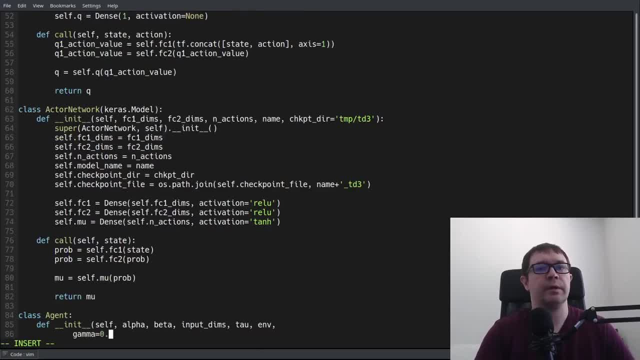 tau for your soft update rule. your tau for your soft update rule. your environment for a number of important environment. for a number of important environment, for a number of important variables from the environment. default variables from the environment. default variables from the environment. default gamma: 0.99. the update, active update. 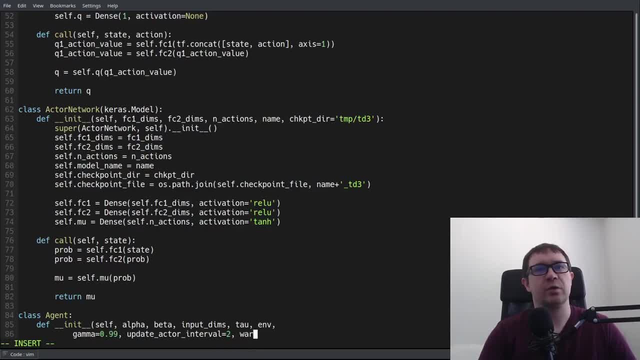 gamma 0.99. the update active update: gamma 0.99. the update active update actor interval. will default it to every actor interval. will default it to every actor interval. will default it to every other iteration. a warm-up of a thousand. other iteration: a warm-up of a thousand. 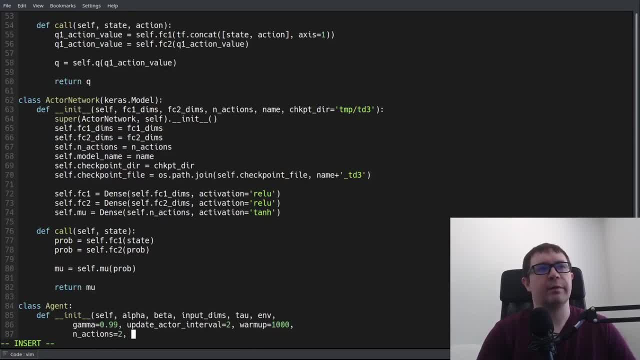 other iteration, a warm-up of a thousand steps. just a default value for inactions steps. just a default value for inactions steps. just a default value for inactions. max size of a million transitions. max size of a million transitions. max size of a million transitions. and. 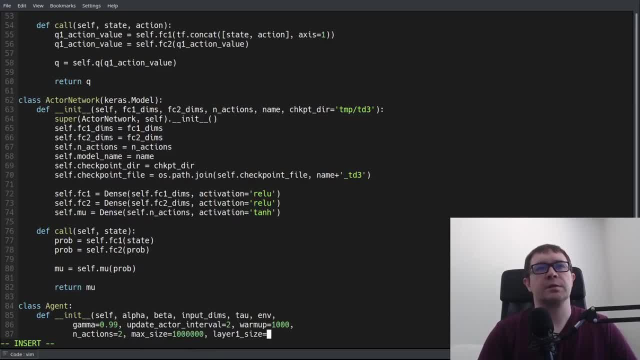 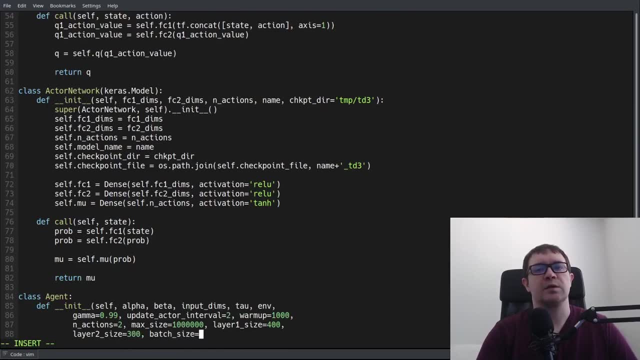 and and layer. one size 400 layer. two size layer. one size 400 layer. two size layer. one size 400 layer. two size: that's our FC one and two dims. that's our FC one and two dims. that's our FC one and two dims respectively. a batch size default of 300. 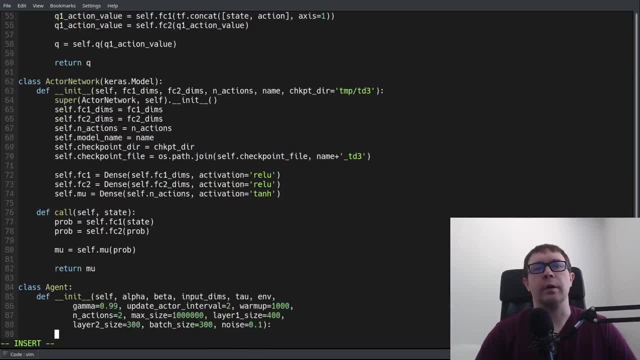 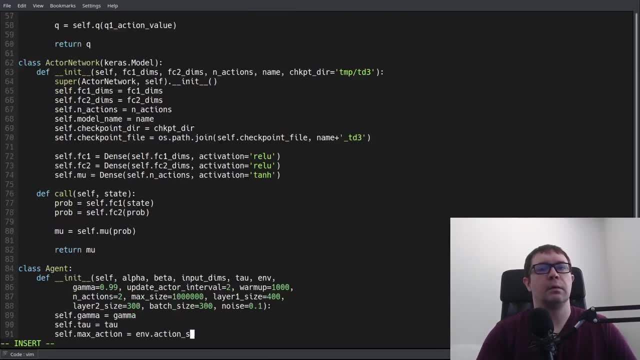 respectively a batch size default of 300. respectively a batch size default of 300 and a noise of 0.1. let's go ahead, and and a noise of 0.1. let's go ahead, and and a noise of 0.1. let's go ahead and start saving stuff, since we will be. start saving stuff. since we will be start saving stuff, since we will be adding in noise, we're gonna have to adding in noise. we're gonna have to adding in noise. we're gonna have to perform clamping on our actions to make, perform clamping on our actions to make. 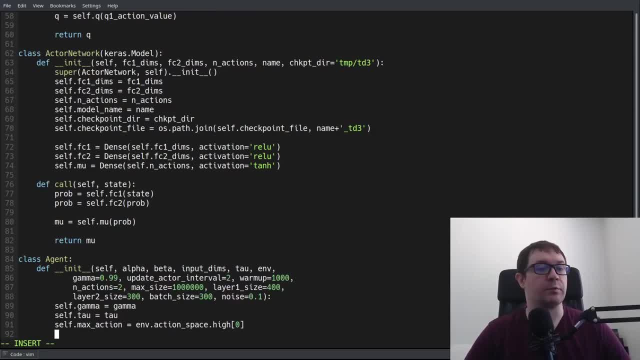 perform, clamping on our actions to make sure that the actions now the action, sure that the actions now the action, sure that the actions, now the action, plus the noise don't fall outside of, plus the noise don't fall outside of, plus the noise don't fall outside of the allowable bounds of the environment. 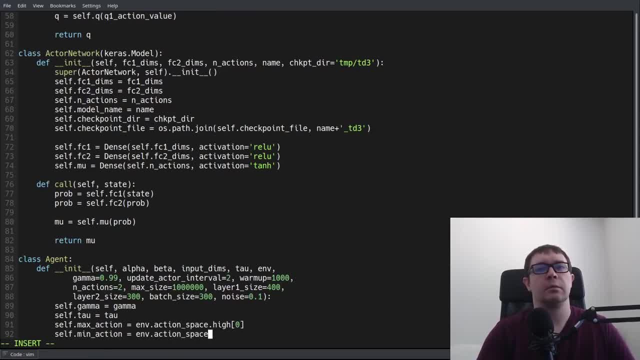 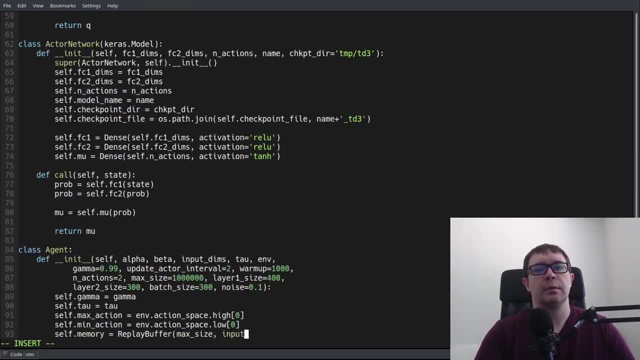 the allowable bounds of the environment. the allowable bounds of the environment or below. we'll need our memory. that's a or below. we'll need our memory. that's a or below. we'll need our memory. that's a replay buffer, then we need batch size. replay buffer, then we need batch size. 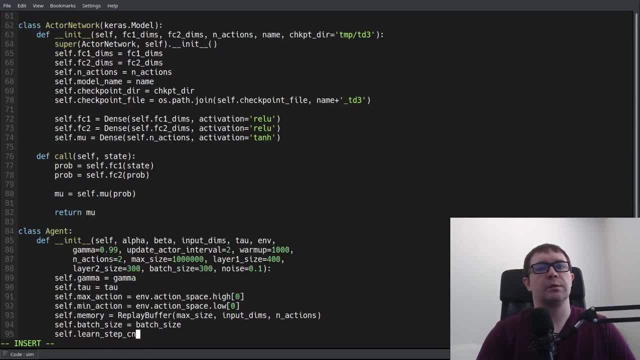 replay buffer. then we need batch size. we'll need a learn step counter. that we'll need a learn step counter. that we'll need a learn step counter that we'll need that because we're doing the. we'll need that because we're doing the. we'll need that because we're doing the delayed part of td3. we're going to delay. 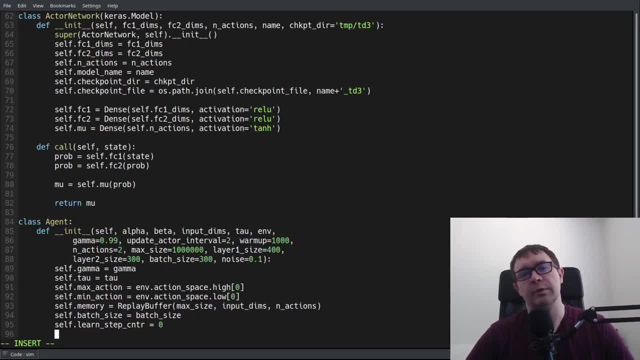 delayed part of td3. we're going to delay delayed part of td3. we're going to delay the updates of the actor network, the updates of the actor network, the updates of the actor network, every to every two different iterations, every to every two different iterations, every to every two different iterations of the update of the critic network to 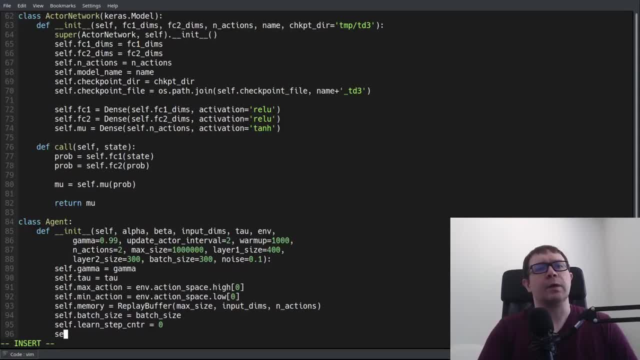 of the update of the critic network to of the update of the critic network to give the critic network time to converge, give the critic network time to converge, give the critic network time to converge, then we have um, then we have um, then we have um. you know, i'm looking at my cheat sheet. 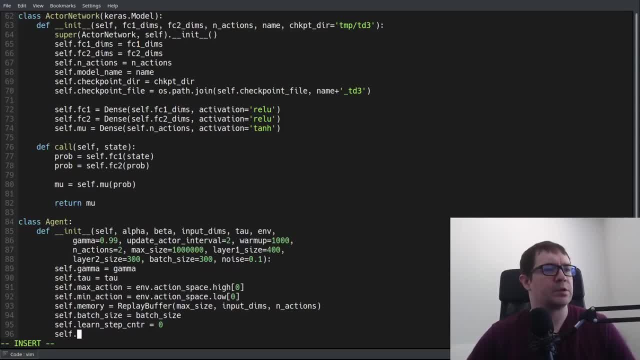 you know, i'm looking at my cheat sheet. you know, i'm looking at my cheat sheet here. oh, a time step here. oh, a time step here. oh, a time step. why do i have a time step? excuse me one. why do i have a time step? excuse me one. 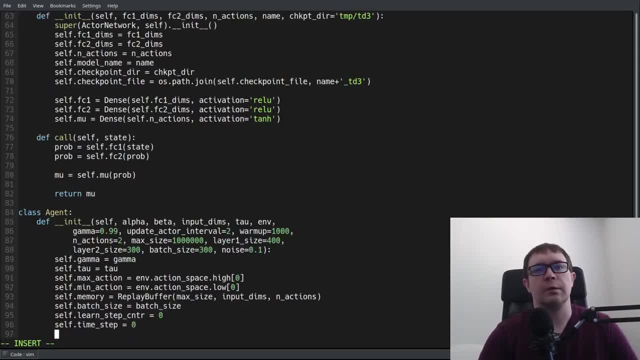 why do i have a time step, excuse me, one moment now. i believe the time step is moment now. i believe the time step is moment now. i believe the time step is for the uh, for the uh, for the uh. warm-up procedure, warm-up procedure, warm-up procedure. we shall double check that later, if not. 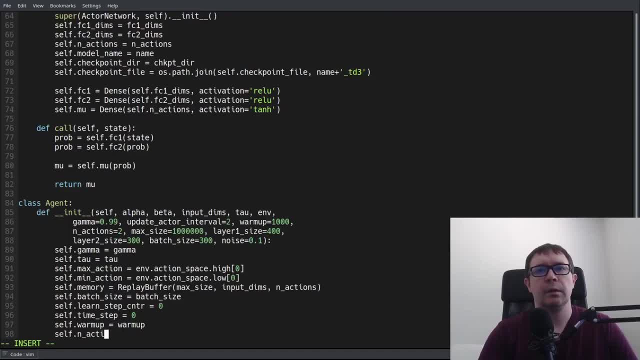 we shall double check that later. if not, we shall double check that later. if not, i'll come back and delete it in the. i'll come back and delete it in the. i'll come back and delete it in the github, github, github. and we don't want to forget number of. 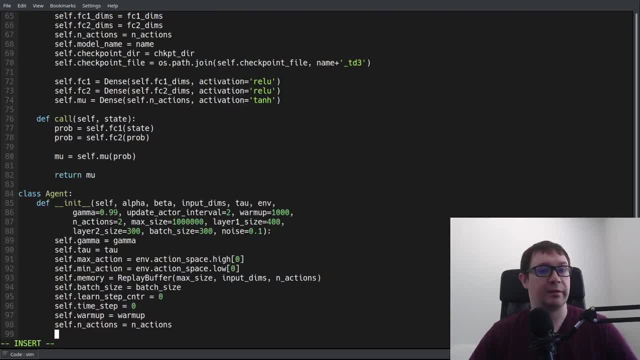 and we don't want to forget number of and we don't want to forget number of actions. sorry, i write this code. you know actions. sorry, i write this code. you know actions. sorry, i write this code. you know, sometimes well in advance of doing the, sometimes well in advance of doing the. 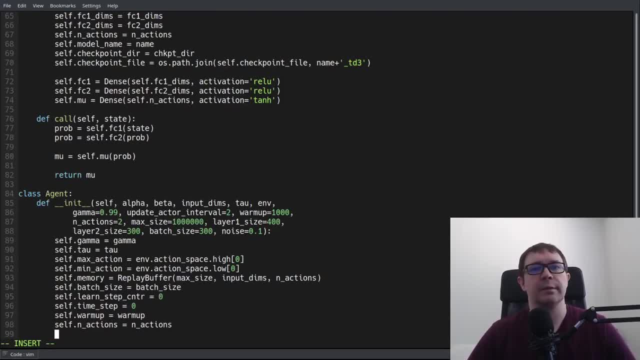 sometimes well in advance of doing the video, video, video, because i get distracted by other stuff. because i get distracted by other stuff. because i get distracted by other stuff, so when i come back to it, i don't always. so when i come back to it, i don't always. 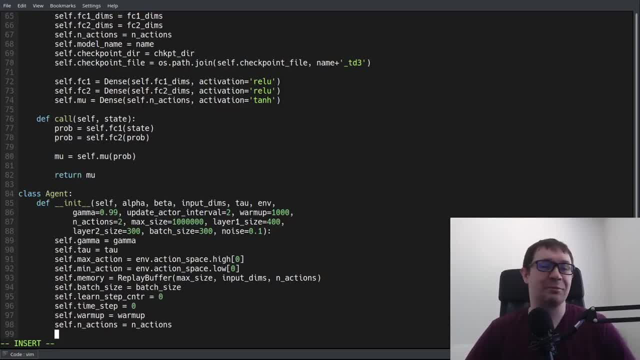 so when i come back to it, i don't always know, know, know what i was thinking. that is the benefit what i was thinking, that is the benefit, what i was thinking, that is the benefit of comments which i don't really do for, of comments which i don't really do for. 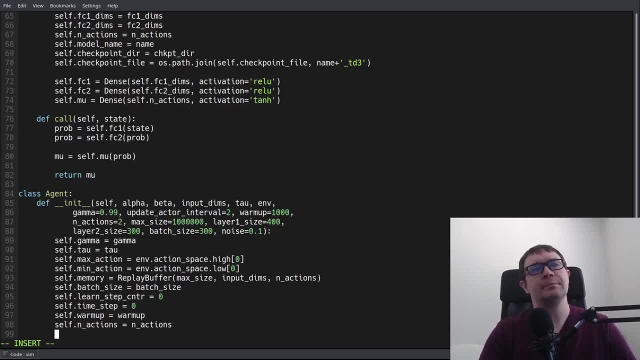 of comments, which i don't really do for this stuff, this stuff, this stuff. sue me, i probably should sue me. i probably should sue me, i probably should. we do need our update. we do need our update. we do need our update. actor: actor, actor: iteration, iteration, iteration, and that is update. 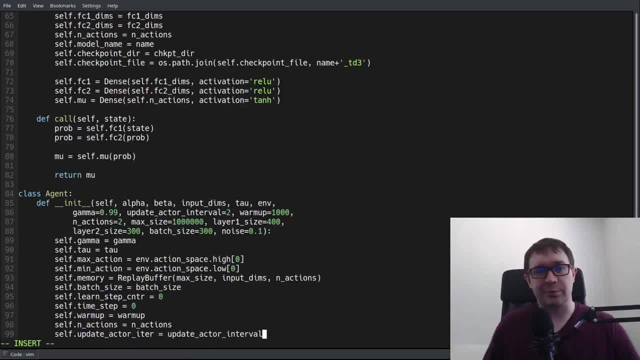 and that is update and that is update actor interval. excuse me, let me close my actor interval. excuse me, let me close my actor interval. excuse me, let me close my door. my toddler is rampaging door, my toddler is rampaging door, my toddler is rampaging. and next we can go ahead and start. 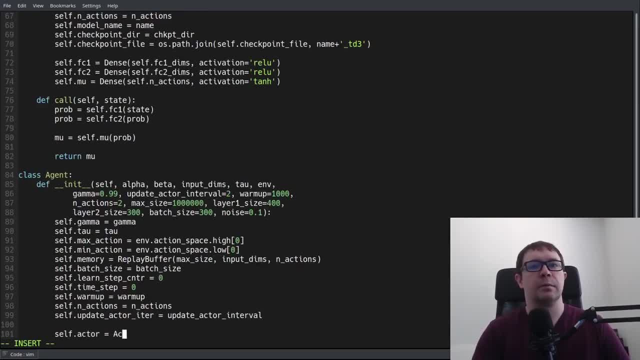 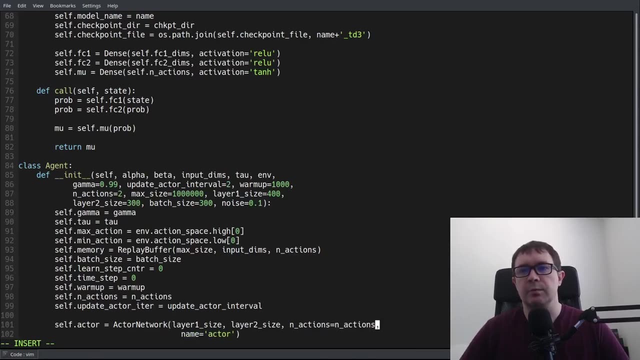 and next we can go ahead and start, and next we can go ahead and start defining our actors and critics, and, and, and so the name will just be actor. so the name will just be actor. so the name will just be actor, because we are quite creative, because we are quite creative. 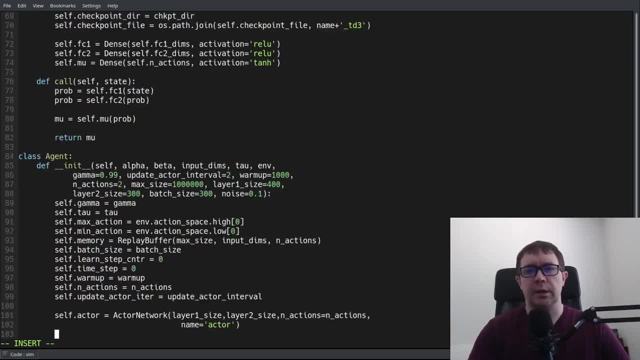 because we are quite creative to maintain compliance with the pet bait, to maintain compliance with the pet bait, to maintain compliance with the pet bait style. god, let's go ahead and delete a style. god, let's go ahead and delete a style. god, let's go ahead and delete a couple spaces. 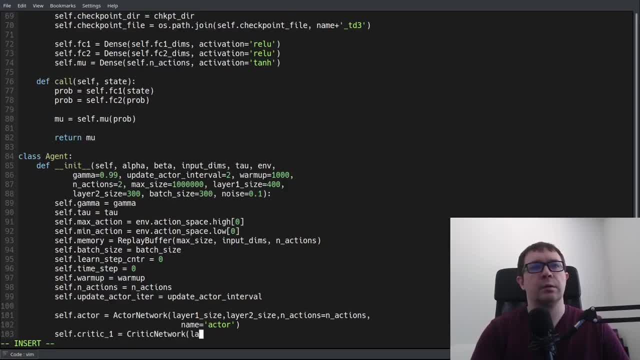 couple spaces, couple spaces. critic. one is a critic, network critic. one is a critic network critic, one is a critic: network: you're one size, layer, two size. you're one size, layer, two size. you're one size, layer, two size and we don't need and we don't need. 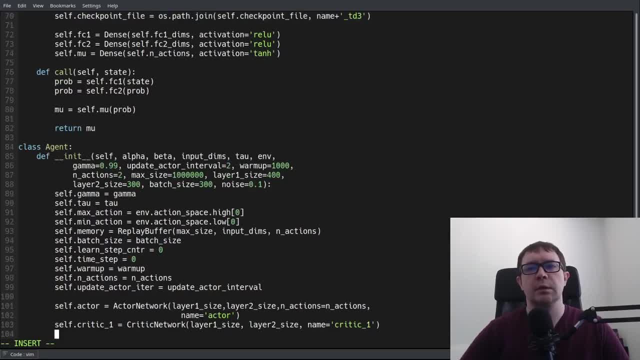 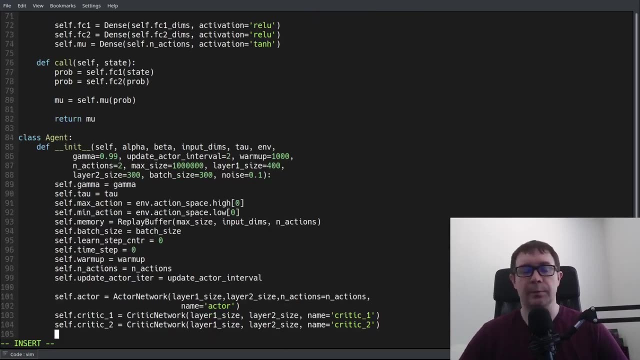 and we don't need um number of actions there because i um number of actions there, because i um number of actions there, because i deleted it, deleted it, deleted it. so its name will be critic one, likewise for critic two and again. the purpose of this is to 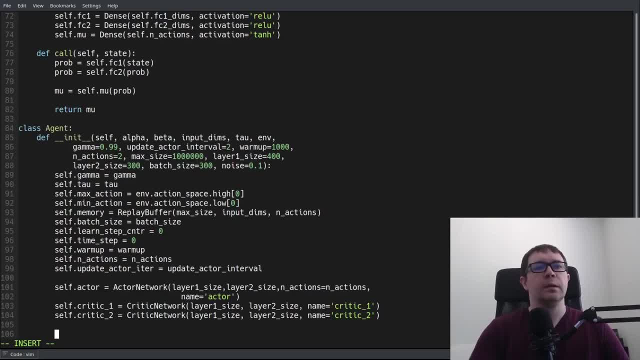 and again. the purpose of this is to and again. the purpose of this is to handle the double q learning update, handle the double q learning update, handle the double q learning update. rule, rule, rule. next, we will need a target actor layer. two size, layer, two size, layer, two size. let me go ahead and delete. 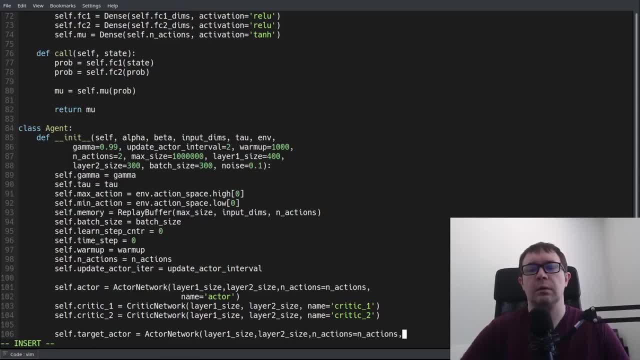 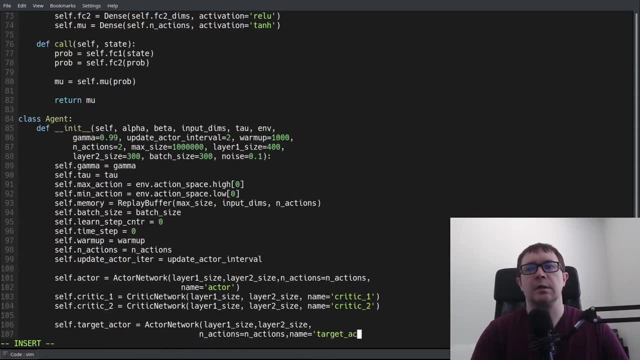 let me go ahead and delete. let me go ahead and delete spaces. oh you know what. oh you know what. oh you know what. silly style guides. and finally a name of silly style guides. and finally a name of silly style guides. and finally a name of target actor. 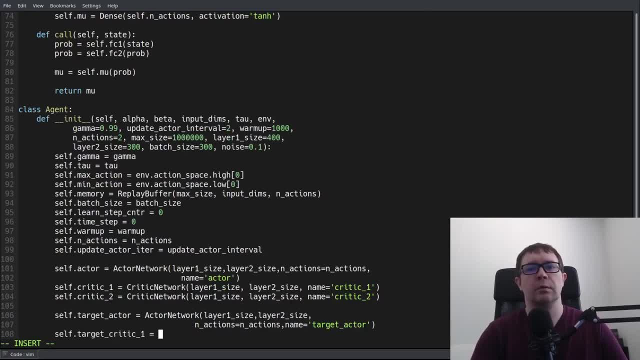 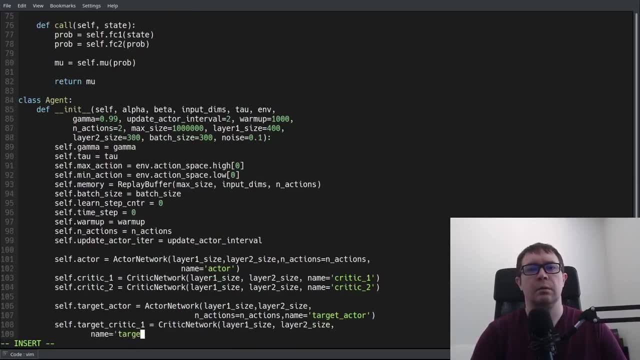 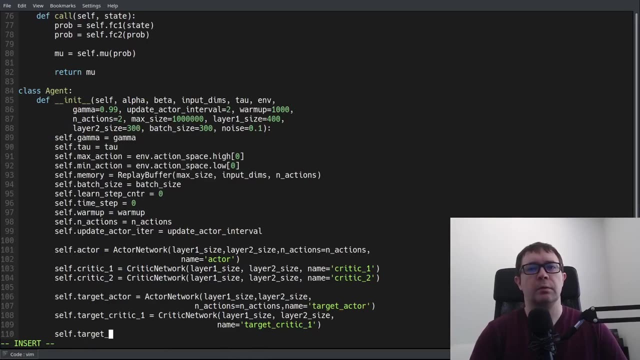 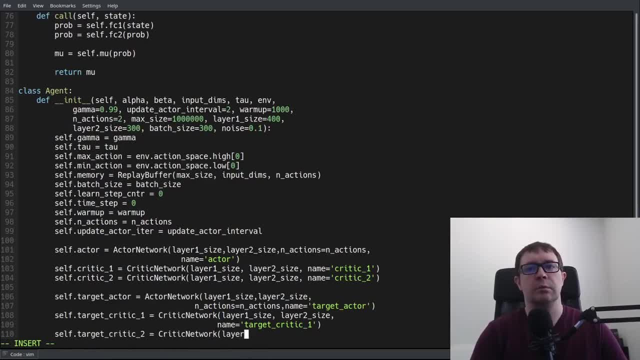 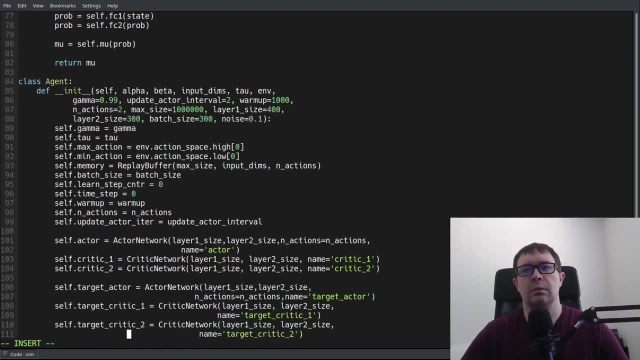 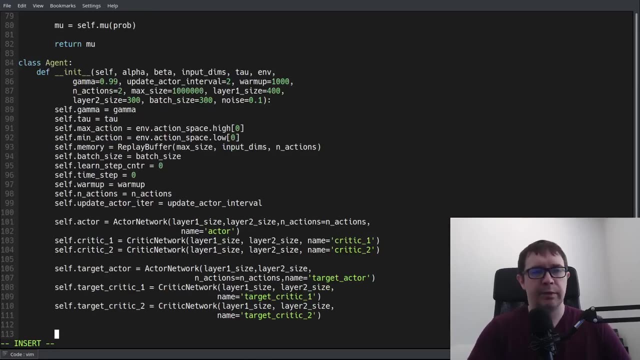 critic one, similarly critic net target, critic two: that is it for our networks. next we have to compile them, because this is a tensorflow 2 and that is where our learning rates come into play. so we will use our atom optimizer with the learning rate defined by alpha for our critic, our 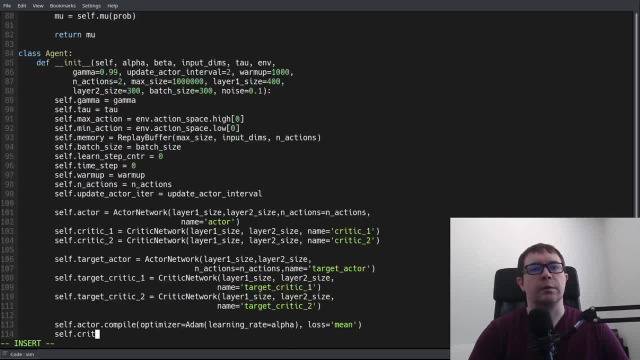 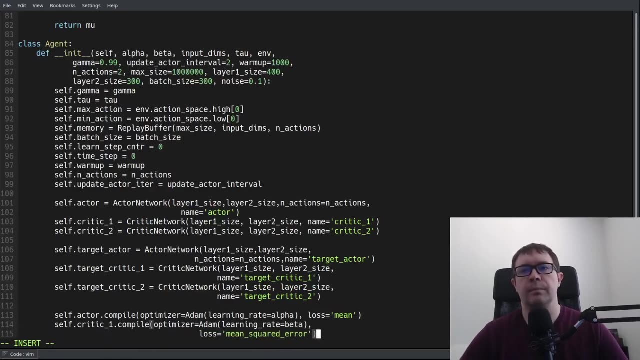 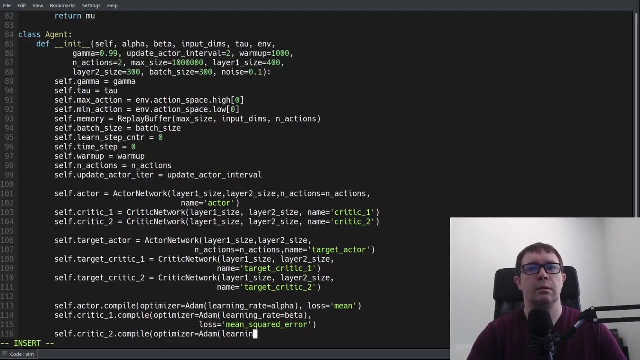 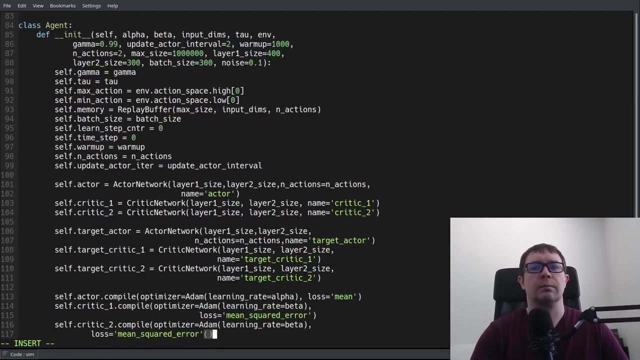 loss would just be a mean and our critic: one learning rate of beta, a loss of mean, squared error and critic to have to do the same thing. your equals beta. do I need- yes, I do, I do need to print the C's there: mean, squared error, and then we 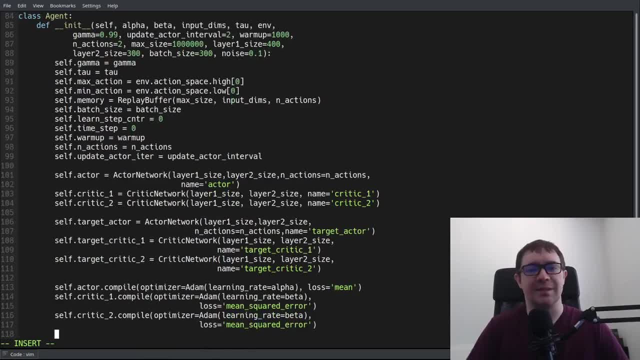 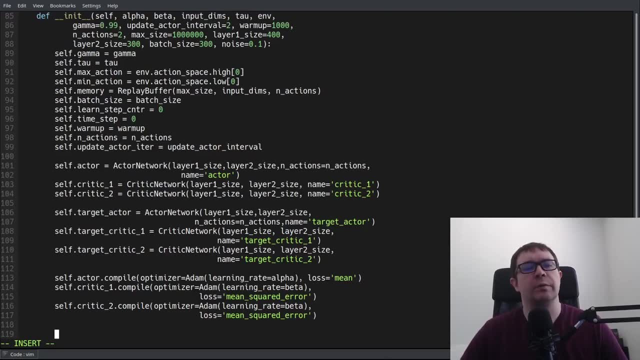 will handle our target networks, nest, target networks, nest next. that is it, tongue twister. so we have to compile the target networks just by convention with tensorflow 2. we're not going to be performing any stochastic gradient descent or atom in this case, on those particular networks. we're gonna be. 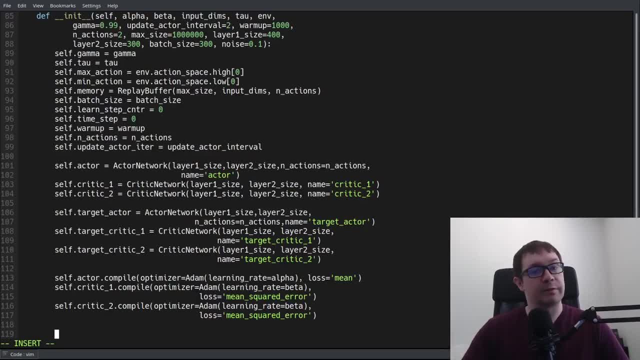 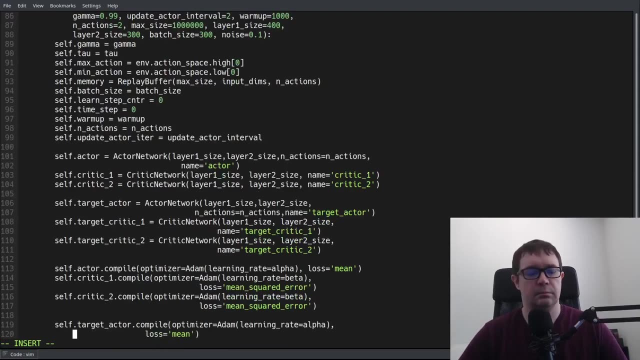 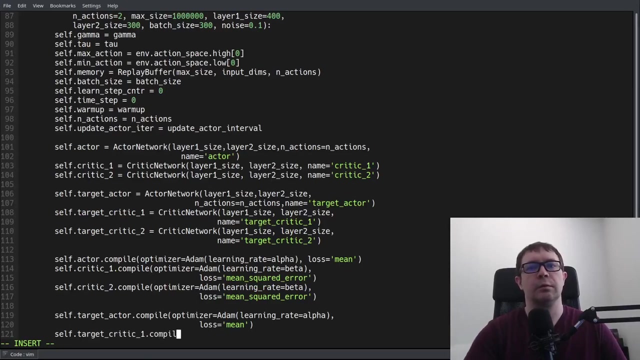 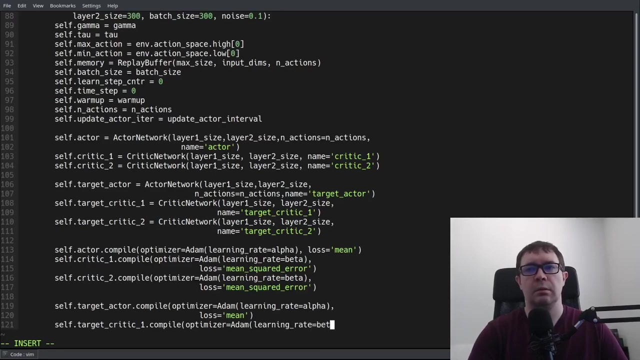 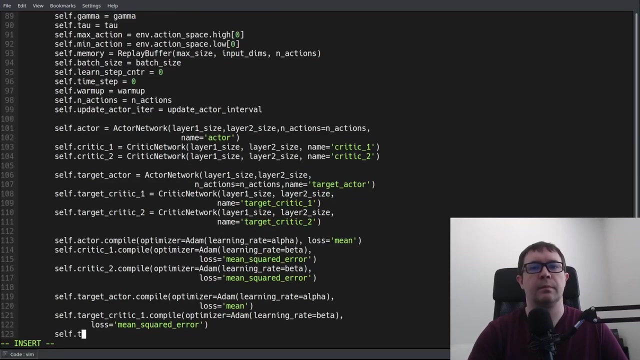 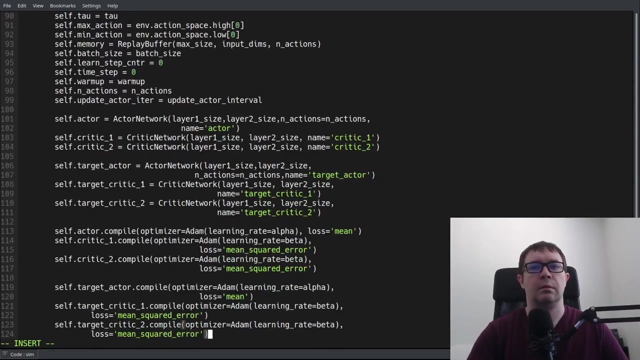 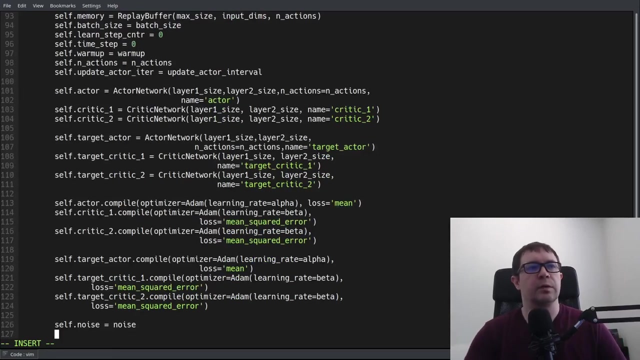 doing the soft network updates, but we still have to compile them nevertheless. that is just by convention. alpha loss equals mean target critic one, you, you. ok, so that is all of our networks. so if that noise we'll keep track of as well. ok, so that is all of our networks. so if that noise we'll keep track of as well. 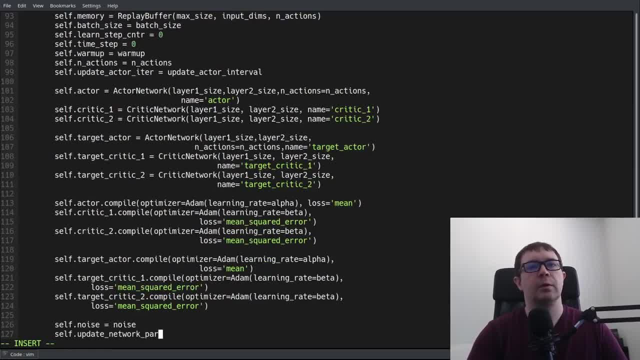 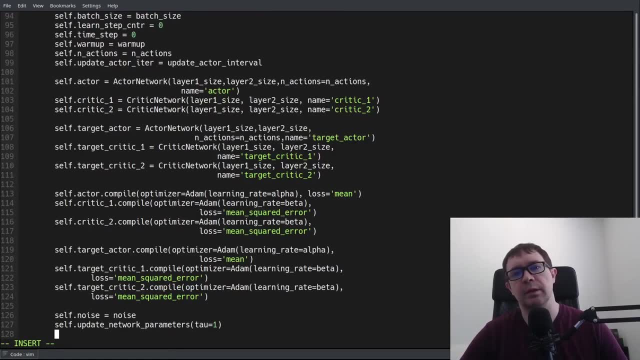 well, Update network parameters with the default value of tau equals one. I do that because on the first step of the update, we have to set the values of our target networks equal to the starting values of the online networks, And so we pass in a value of tau equals one to perform an exact 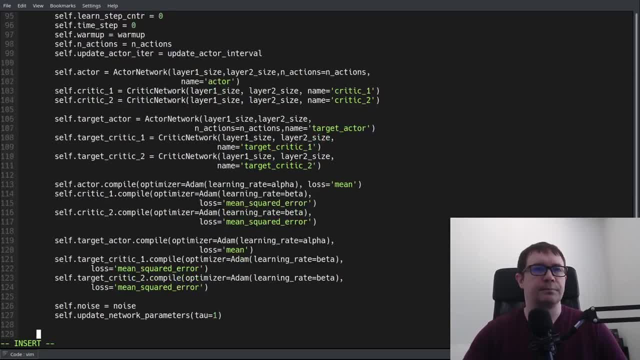 update or a hard update instead of a soft update. We'll handle that function toward the end. For now, I want to get to the choose action, remember and learn functionality, because that's where all the really interesting stuff is. So let's go ahead and choose an action based upon an observation. 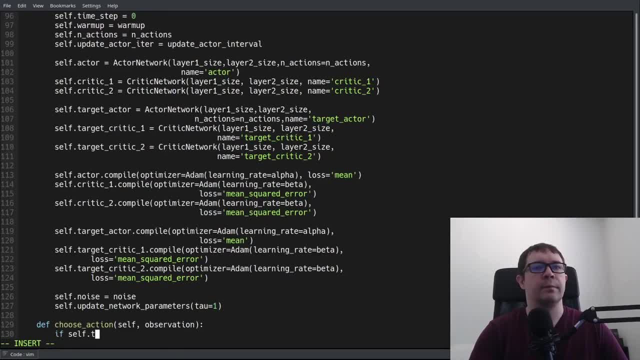 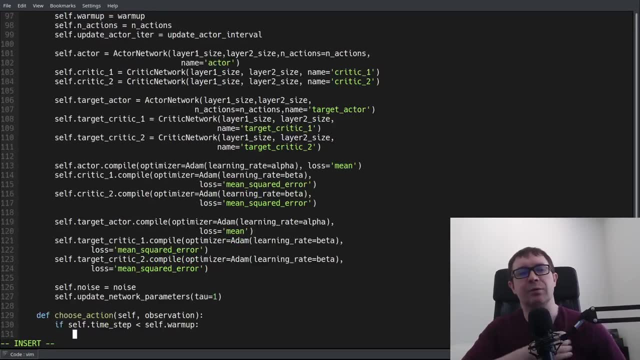 of the current state of the environment as input. So if our time step is less than our warm-up period, yeah, that's why we need the time step to handle the warm-up, as I suspected. Glad I didn't delete that We're going to select an action at. 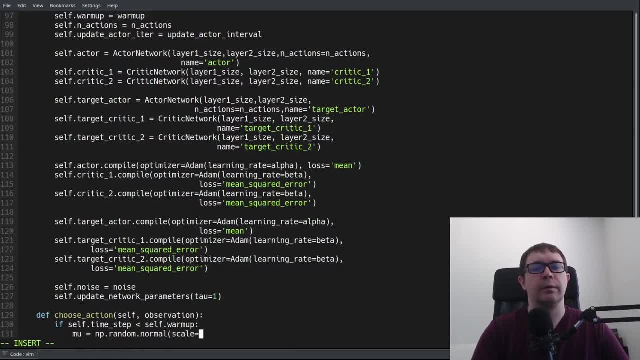 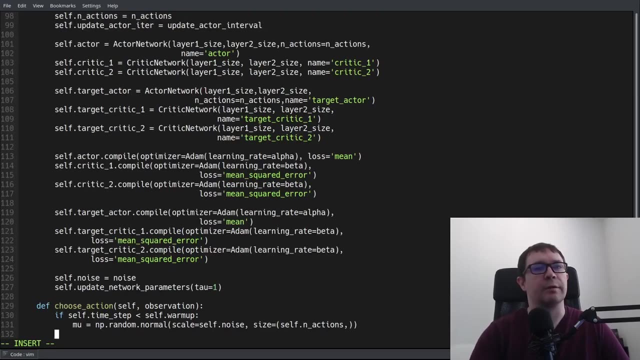 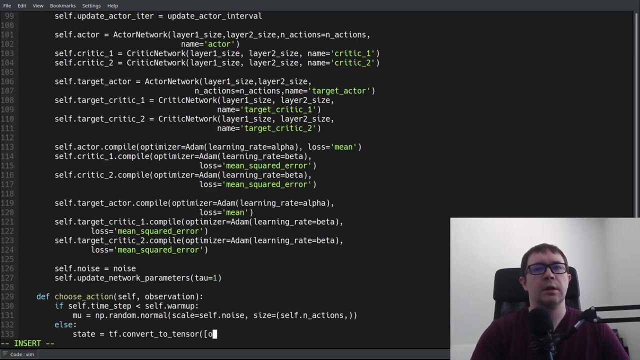 random, With just a normal distribution, with a scale defined by our noise parameter in the shape of number of actions comma. so we get a batch there, Sorry, an array of scalers. Otherwise we want to go ahead and convert our state to a tensor and add on a batch dimension. That's just the way that the inputs 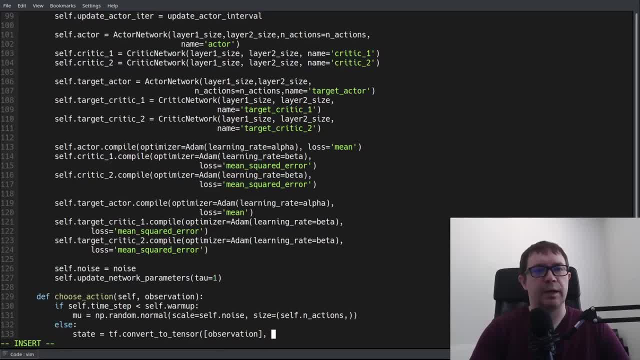 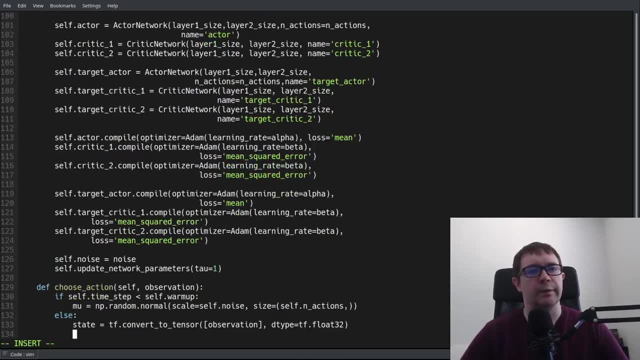 are expected to be fed into the deep. So if we want to add an action to a underlying neural network, we have to add that batch dimensionality, And I have tffloat 32 here. it must be due to some sort of precision thing that makes. 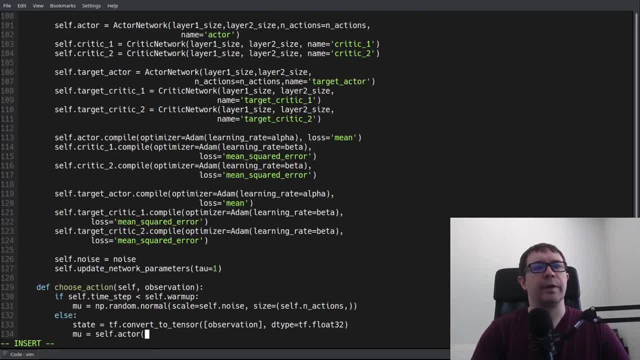 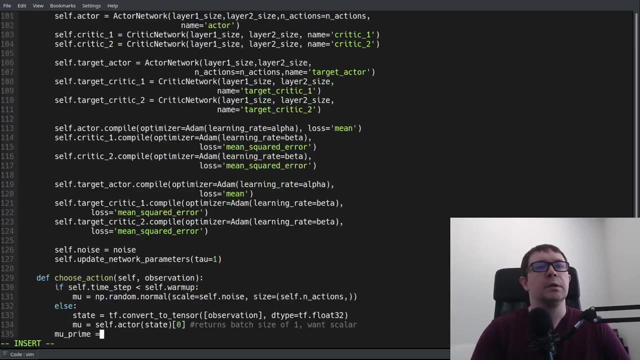 TensorFlow happy. So then we want to pass our state through our actor network and receive our mu, and we're doing that because it returns batch size of 1, want scaler? Then we'll say: mu prime, which is where we handle the noise, equals mu plus npn. 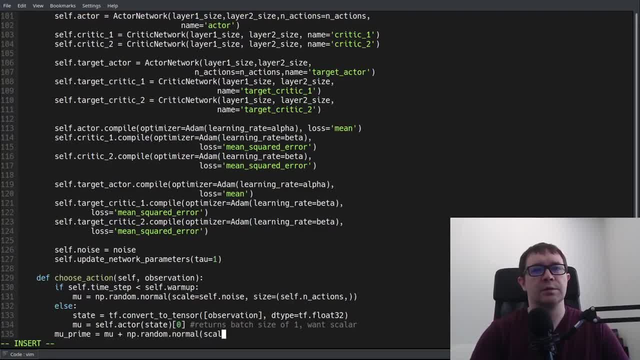 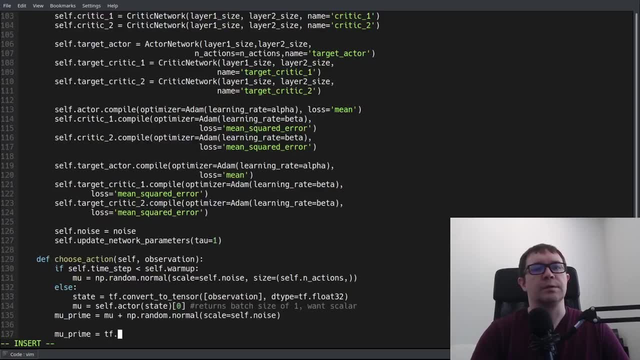 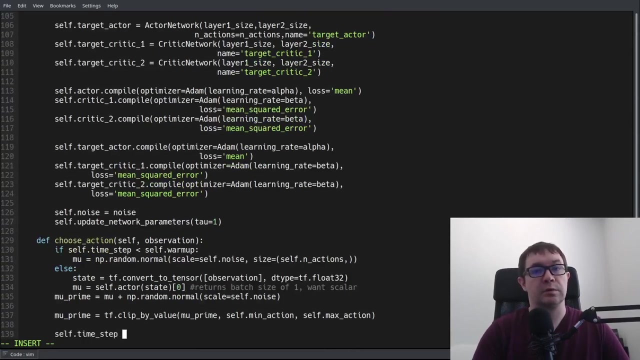 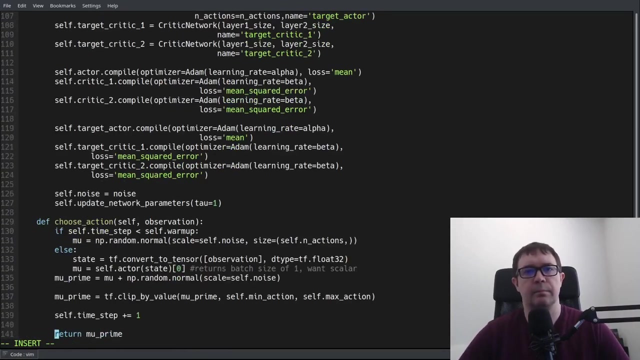 be random. normal scale equals self dot noise and mu prime is TF clip by value, because again that noise could take us outside the bounds of our environment. so we'll plant mu prime between min action and max action, increase our time step by one- very important- and we want to return mu prime. okay, that's it, for I choose action now. 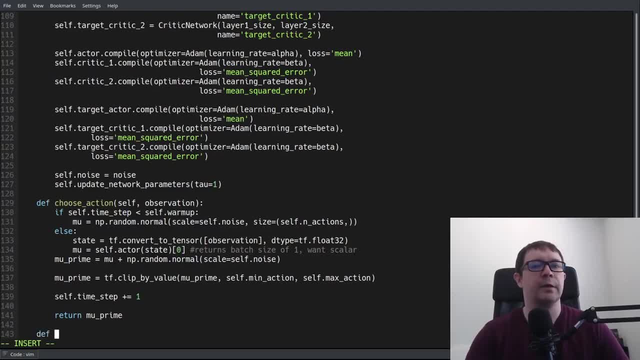 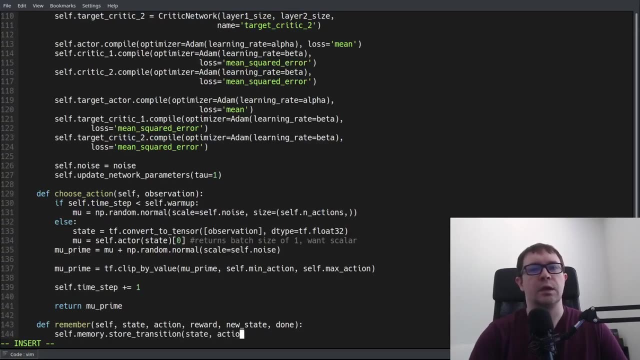 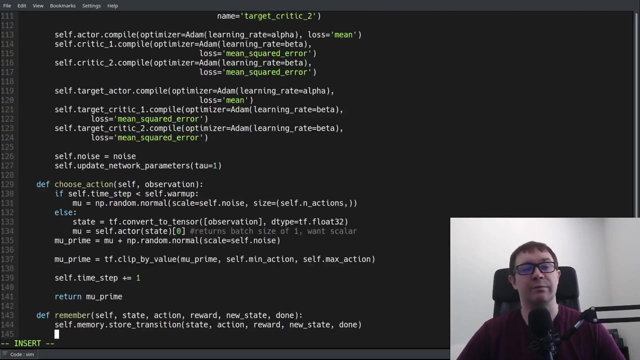 let's handle the simple interface function to remember a transition. so remember state action reward, new state done. and we'll say memory dot store transition, state action reward, new state done. and that's just because we have to interface with the memory in some way. we don't want to have the agent class calling you, don't want to have the agent class interacting. 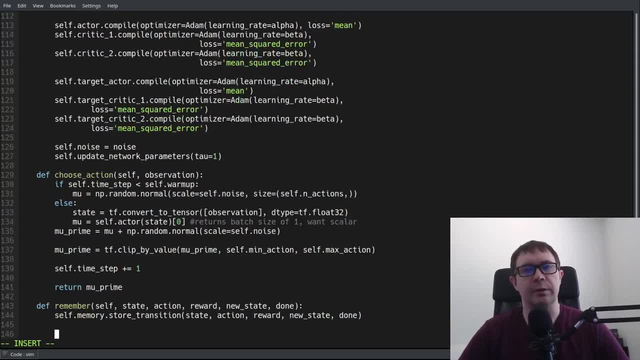 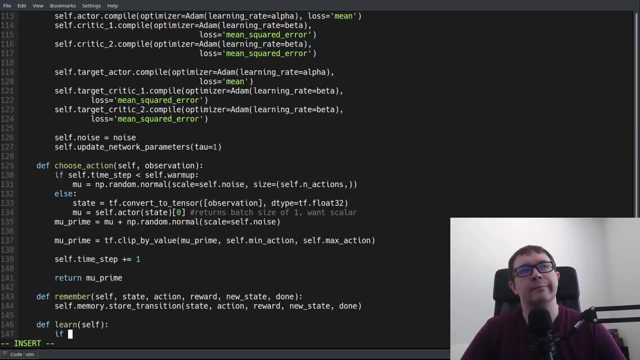 with private variables from your memory. that would be poor software design. so next we handle the most interesting function in the whole program, which is the learn function. and the very first thing we want to do is say, hey, if we haven't filled up at least back size of memory, we probably don't want to be learning. so we'll save self dot. 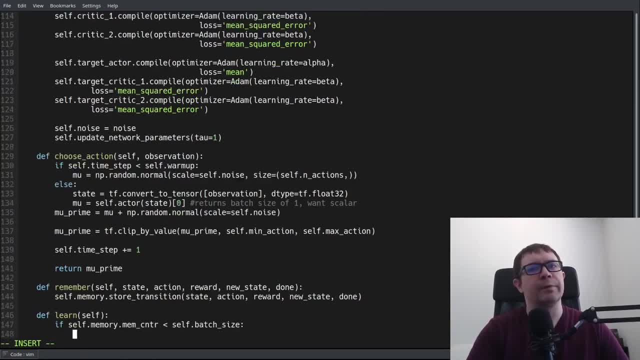 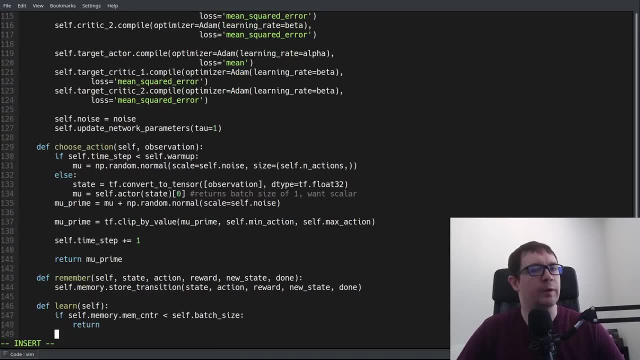 memorymemcounter plus in batch size. now, if it's not, if it's not greater than the batch size or equal, to go ahead and return now, since we're doing a warm-up. that won't be the case, because the batch size is just a few hundred, the warm-up is a thousand. so by the time we get through the 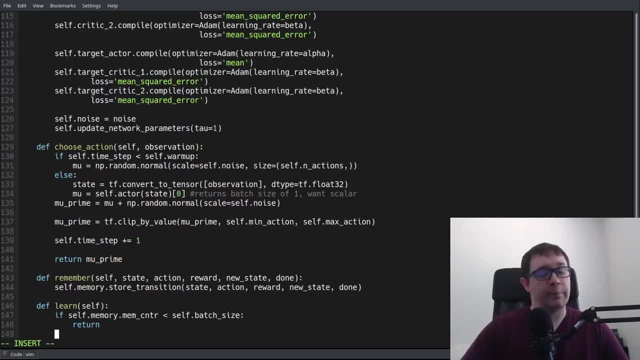 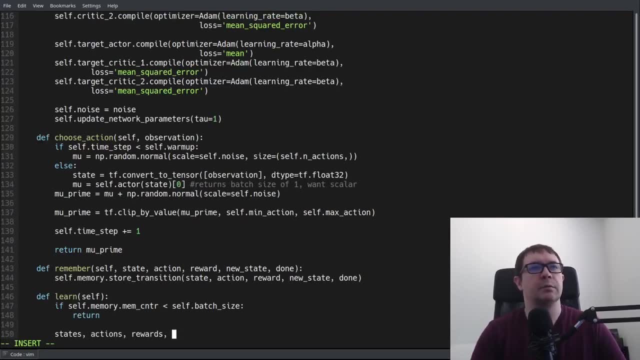 warm-up, then we're already well into filling up a batch size of memories. but if you decided not to do a warm-up, then that would be a very crazy problem. so we'll go ahead, and let's go ahead. if don't warm-up, then that would be important. so we'll start by sampling our memory self. 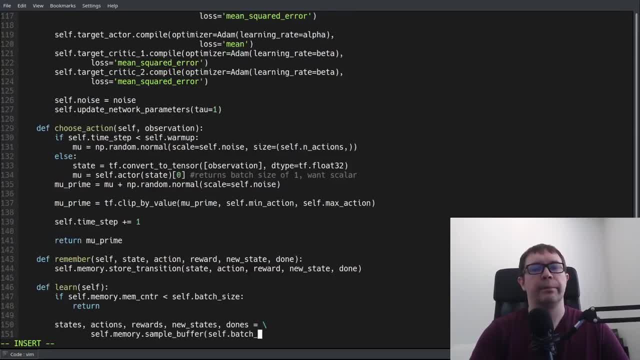 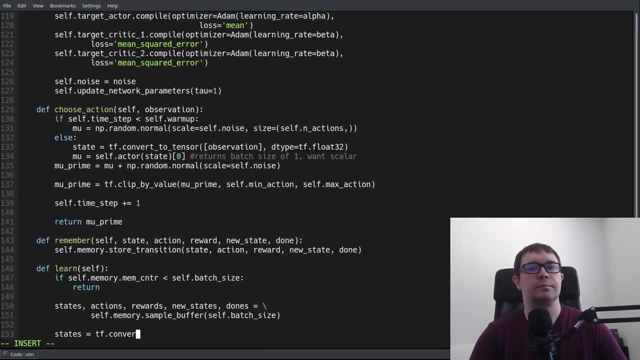 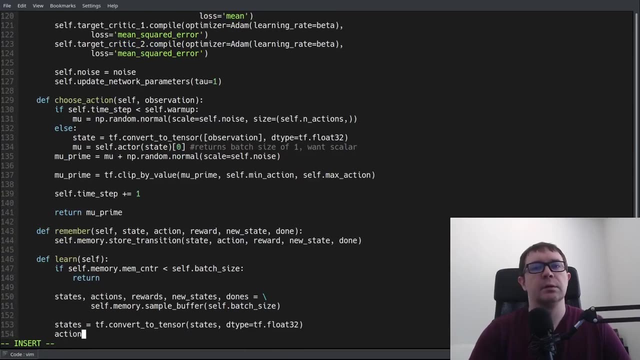 memory sample buffer pass in our batch size and then we want to convert all of those to tensorflow tensors and I have to be very pedantic with data types here. I think there could be issues if you do not, as I recall, I think it barks at you. 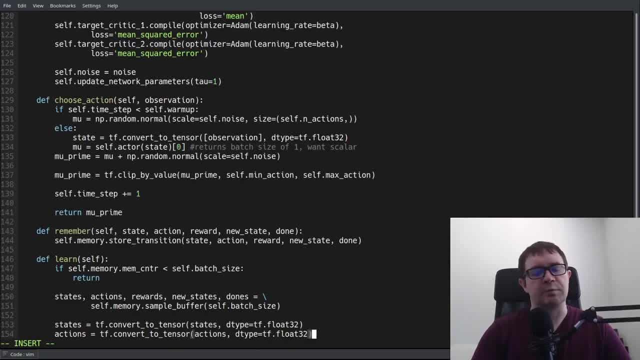 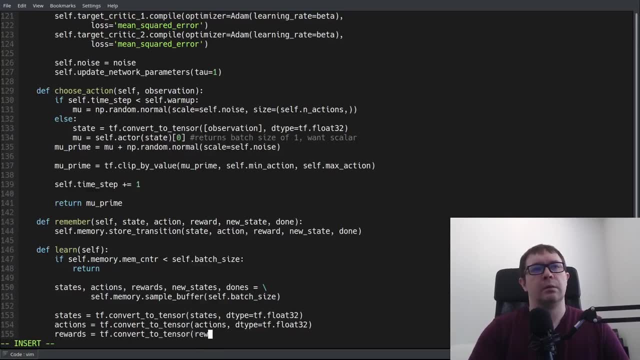 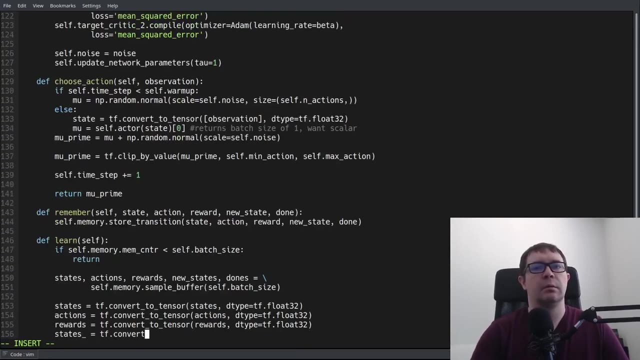 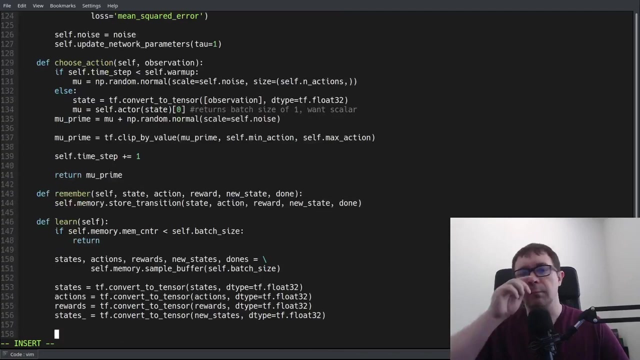 about data types because it expects certain types of floating-point variables in some places and other types elsewhere. and we don't have to convert the duns to a tensor because we're not sticking that in the deep neural network, we're just using that as a multiplicative factor. so 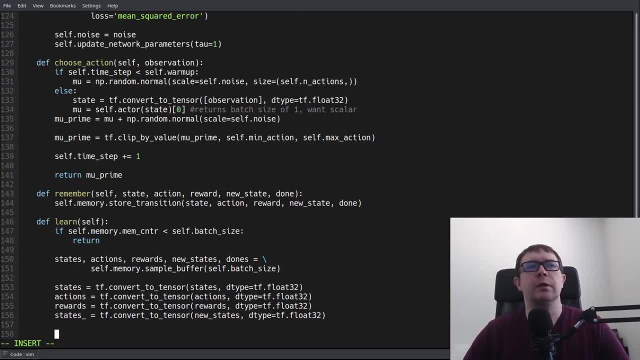 we can leave it as a numpy array. now we're gonna handle our update to the critic network, because we do that every time step, and then we'll handle the update to our actor network. so we'll say, with TF gradient tape, you know, I have persistent equals zero, so we're gonna do that every time step, and then we'll handle the update to our actor network. so we'll say, with TF gradient tape, you know, I have persistent equals. 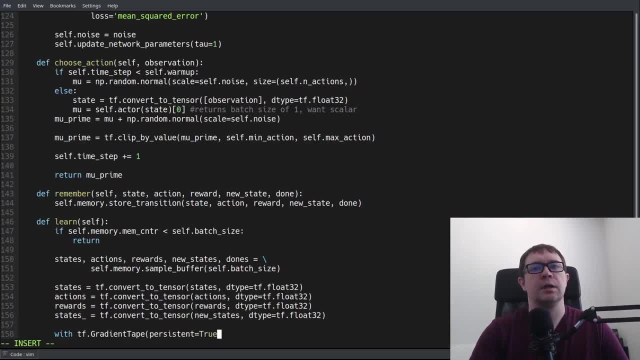 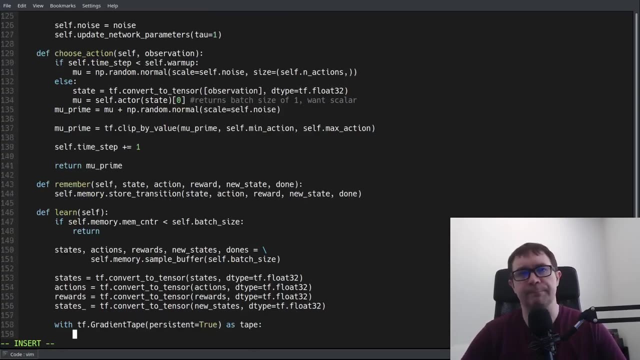 true, oh, because I have two different networks. yeah, so you need two different. if you're using two different updates for one, excuse me. if you're using two different, apply gradients for a single tape. then you need to pass in the persistent equals: true variable parameter, excuse me, or argument? 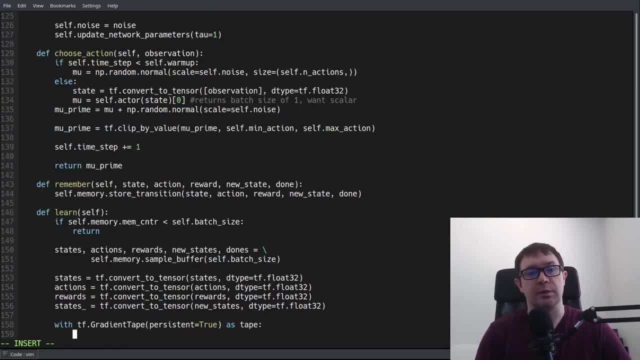 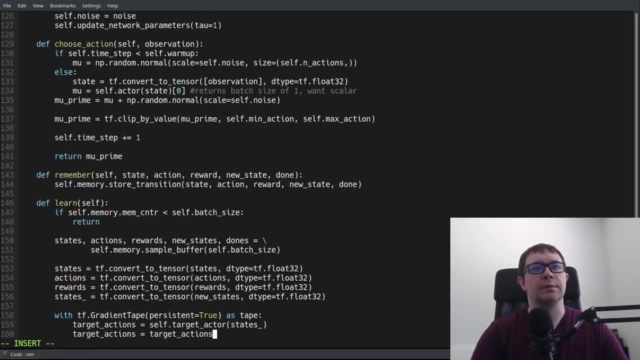 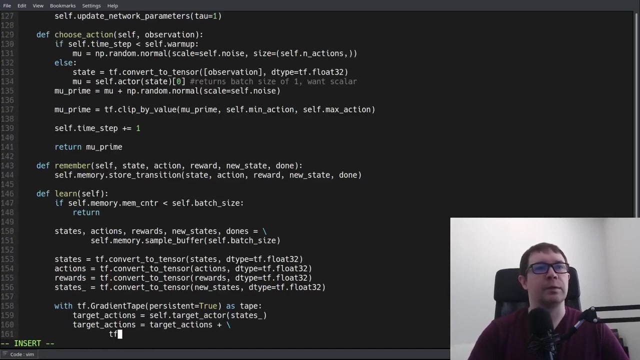 otherwise you don't need that persistent equals. true, you just have, say, a single network that you're performing an update on. so we want the actions according to our target actor for the new states, and then we're going to go ahead and add on a noise parameter to that, that we're going to clip between the range of minus point. 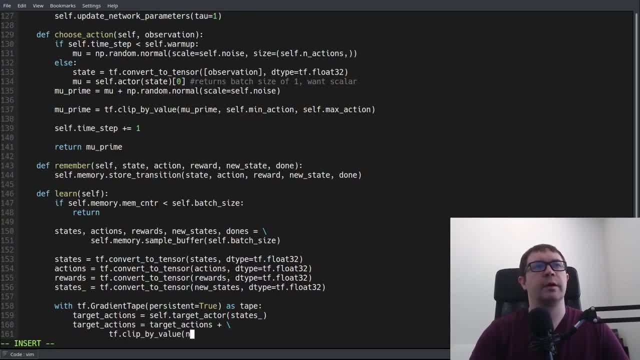 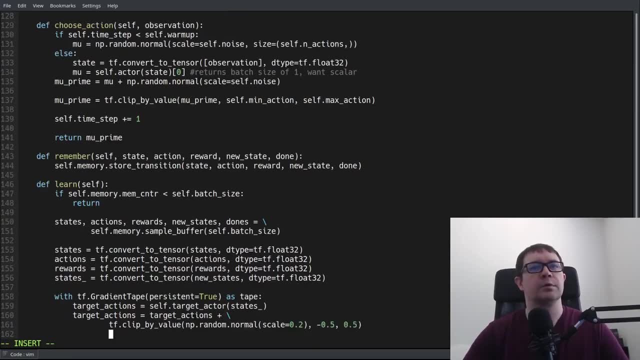 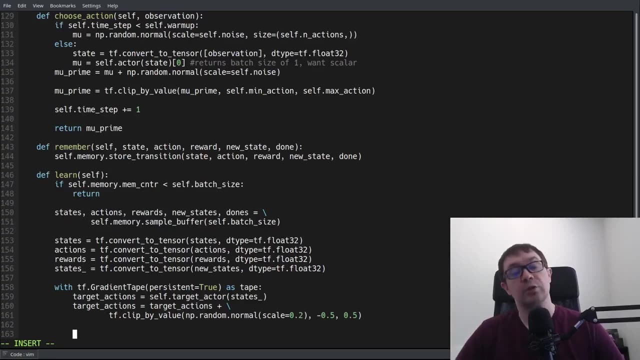 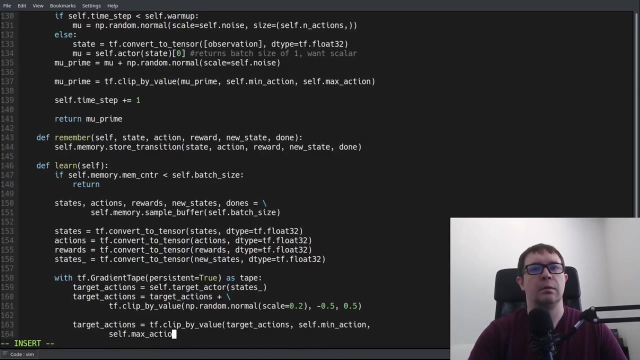 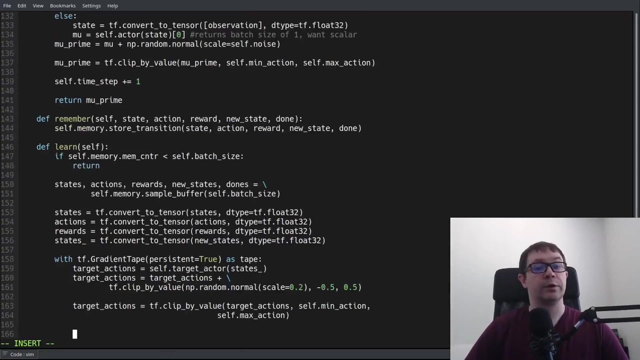 five and positive 0.5. so clip by value NP, random normal 0.2 minus 0.5, 0.5. and then we're going to go ahead and clip that again, because again the addition of that noise could take the action outside of the bounds of our environment, and then we are free to go. 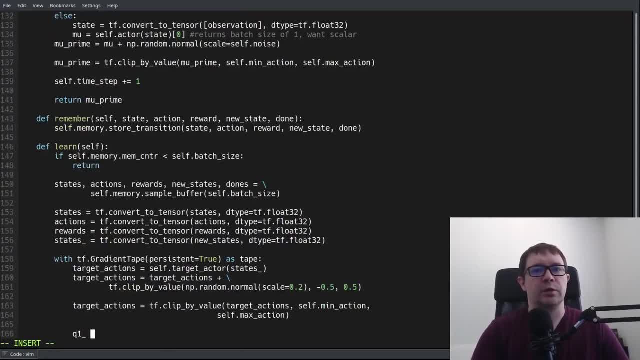 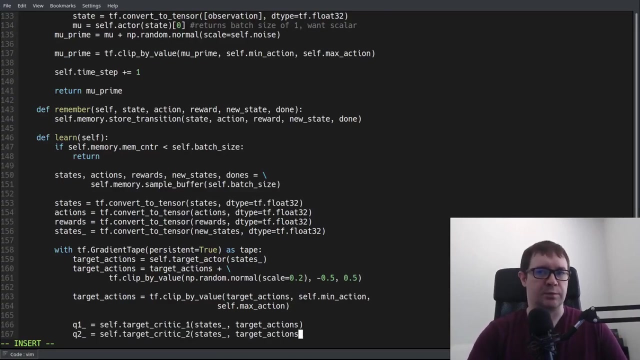 ahead and start calculating our critic values. so q1 underscore- the critic value according to the first target critic- is the feed forward of the new states and target actions through the first target critic. q2 underscore is very similar. it's just the evaluation of the new states and target actions according to. 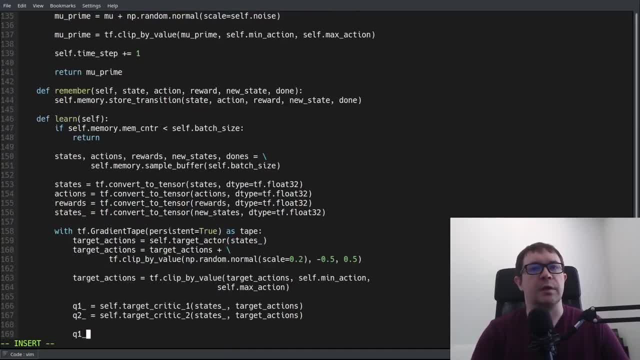 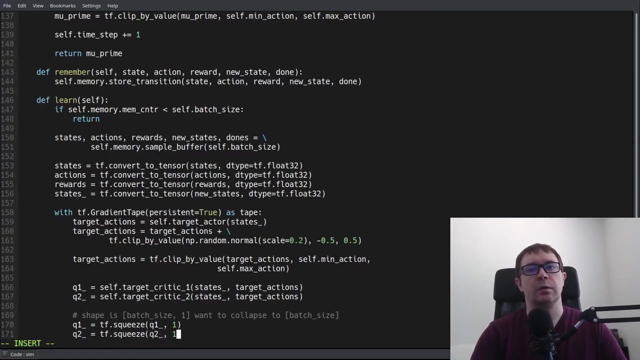 the second critic. now again, we're going to have to go ahead and squeeze that output, and the reason is is that our shape is batch size by one want to collapse to batch size, and we have to do that for q2 as well- excuse me, q2 underscore. and then we're going to need the, the value of the. 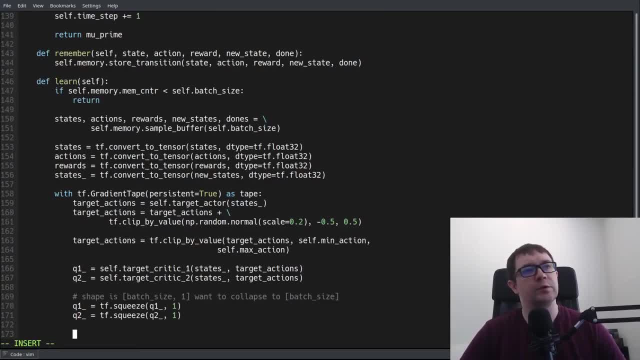 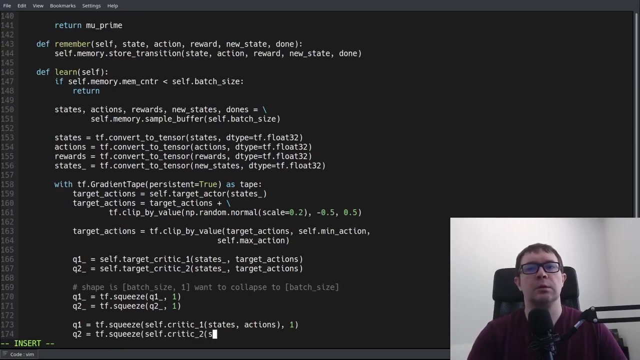 states and actions the agent actually took, according to the regular critic one- excuse me, one- and two networks. so we'll call those q1 and we'll just go ahead and squeeze those right away. critic one: states actions squeezed along the first dimension. critic two states, actions one. and then we're going to say that our critic value. 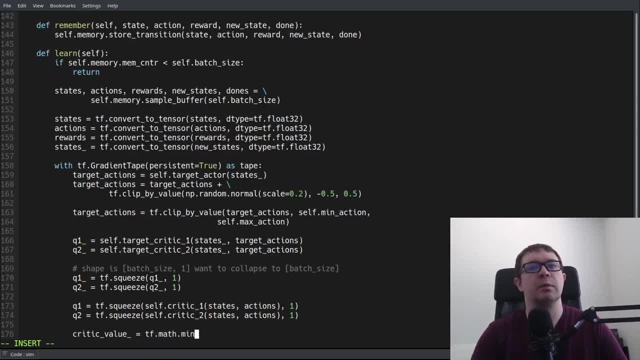 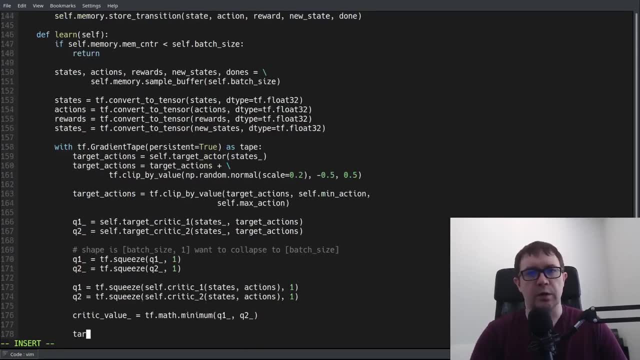 is the minimum of q1 underscore, two underscore. so we will put the value of this now and find out what's the minimum of the target value for the new states is the minimum of q1 underscore, q2 underscore, and then we're going to need our target value, the Y from our paper rewards plus gamma times critic. 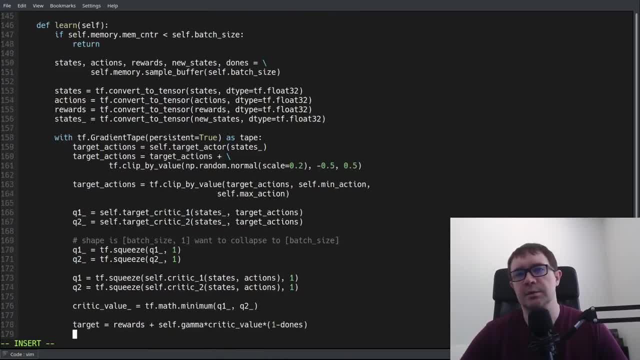 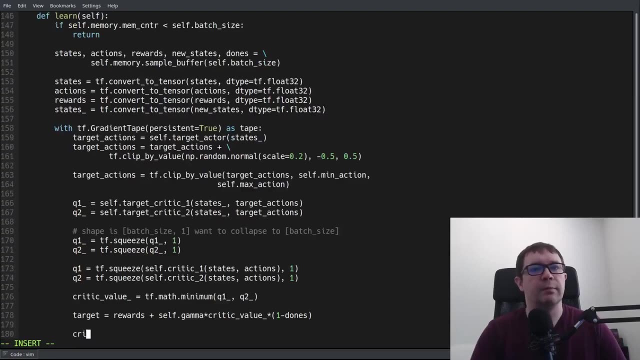 value times one minus done. that will set the value of the second term here. gamma times critic value. there should be an underscore, they're sorry to zero. everywhere the done flag is true And then we have our losses. So critic one loss, Karis. losses dot mean squared error between the target and q1.. 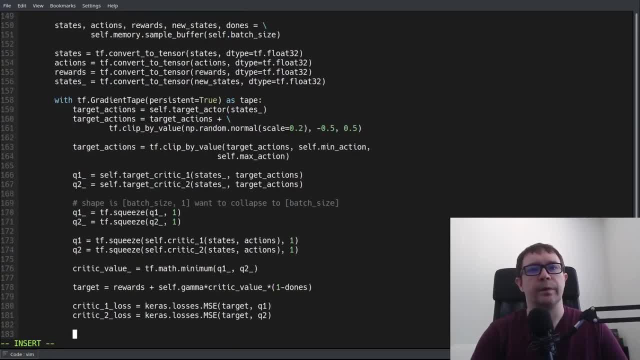 Mean, squared error, target and q2.. So that is it for the calculation of the critic losses. Now we have to handle the calculation of the gradients. Now we don't have to do anything special for that, the tensorflow package handles that for us. So tape dot gradient gradient. 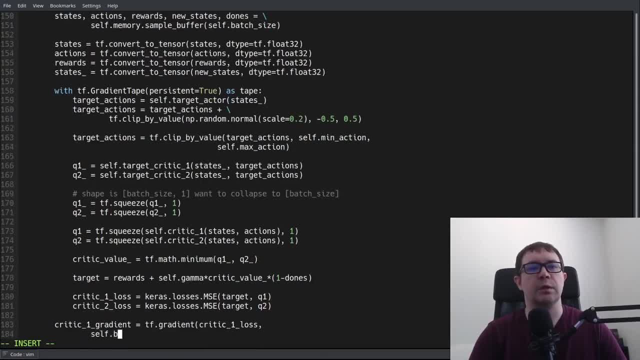 critic: one loss with respect to the critic. one: trainable variables. So that should be dot, not an underscore. I make that mistake frequently. Critic: one critic underscore, one dot. trainable variables- Yeah, that is right. And then we need the critic to grant. 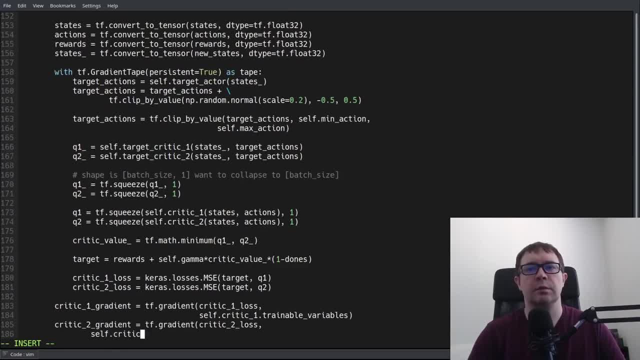 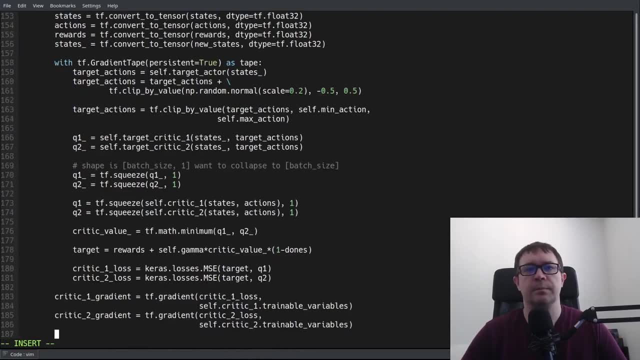 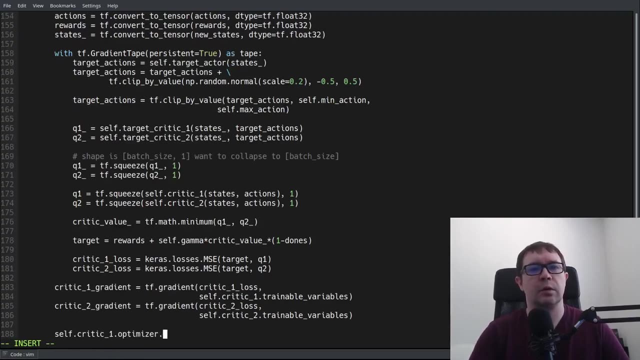 critic to loss, So dot. critic to trainable variables- Same deal. Then we need to go ahead and apply those gradients. So calling our optimizer, dot apply gradients function And that expects a zip as input. we're going to zip the critic, one gradient. 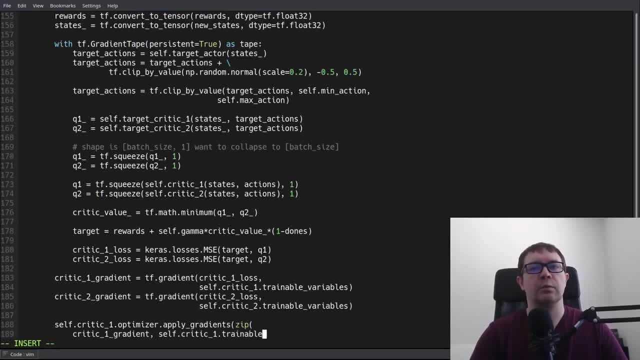 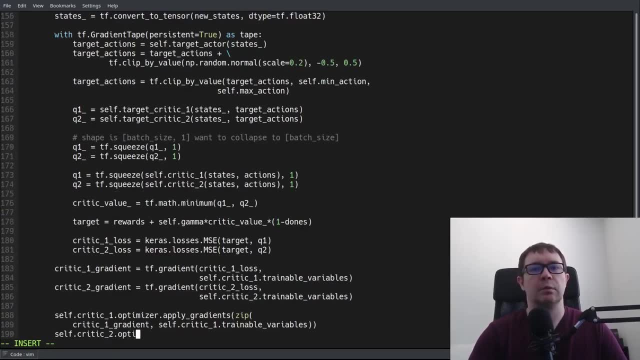 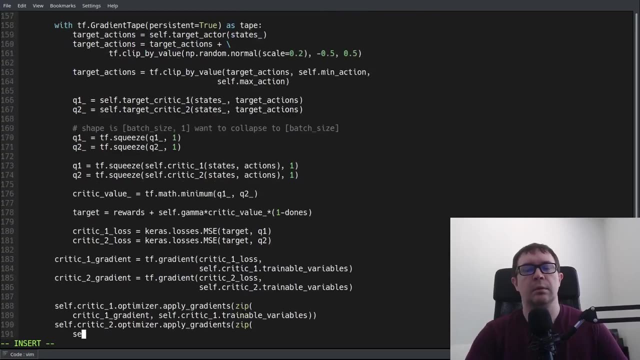 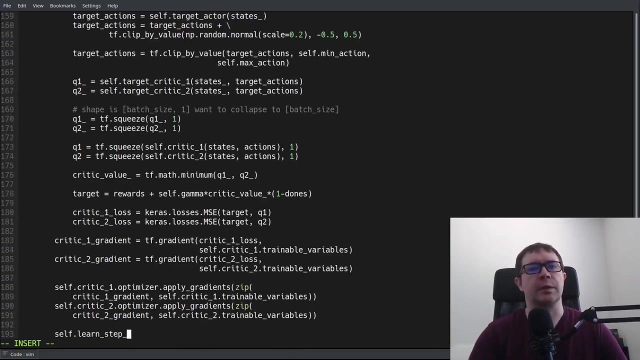 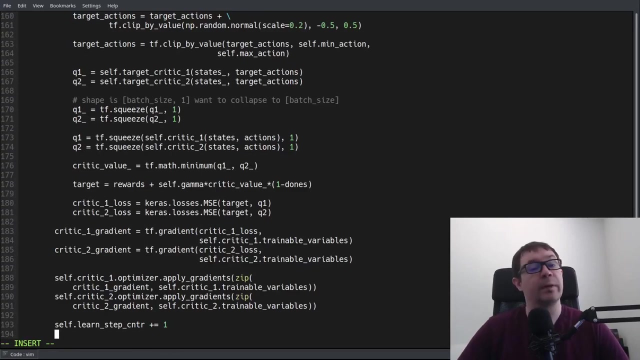 And the self critic one trainable variables. Same thing for critic to optimize for two gradient Okay. and then we want to increment our learn step counter, because that gets incremented every time we update our critic networks. and then we have to address the question of is it time to update our actor network? so we'll say if that learn step counter. 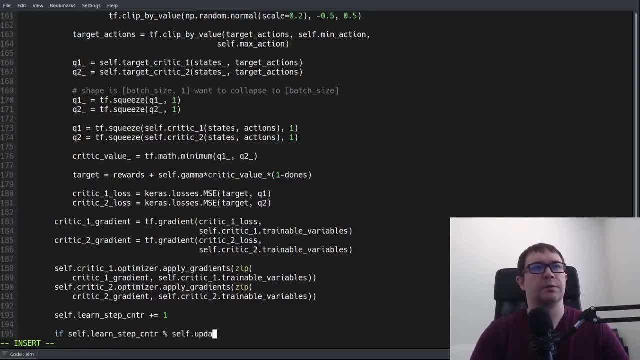 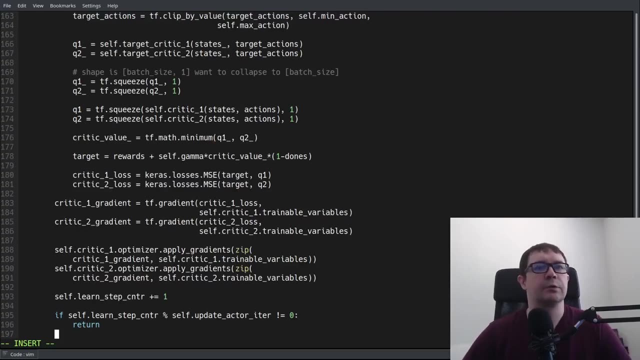 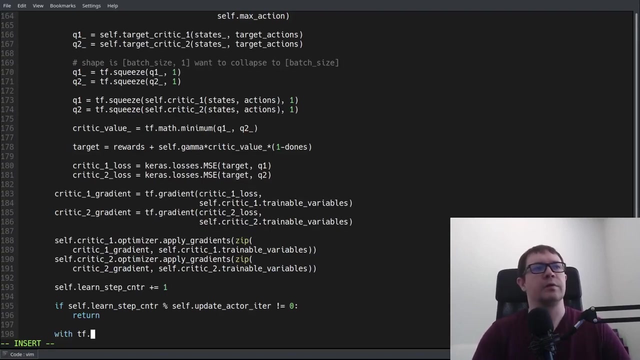 modulus selfupdate actor interval. iter- sorry, is not equal to zero, then return. so if it's not every n steps, then go ahead and return, and if we haven't returned, then we're going to go ahead and calculate the loss for our actor network. so a tf gradient tape as tape, and here, since we're just 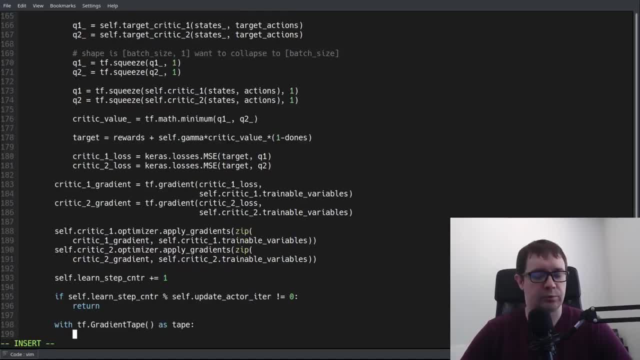 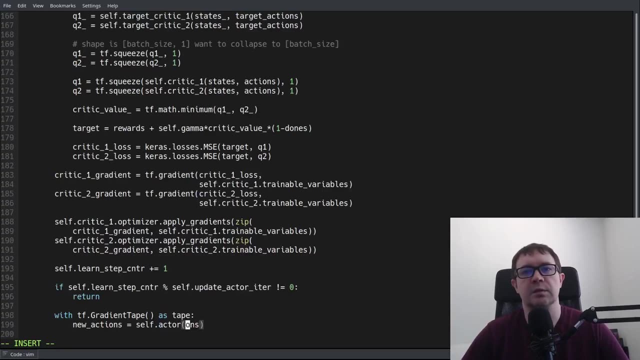 dealing with one loss. we don't have to call the persistent equals true. we don't have to pass in the persistent equals true argument. so let's our new actions are the actions chosen by the current argument parameters or actor network for the current set of states, the states the agent saw along the way. 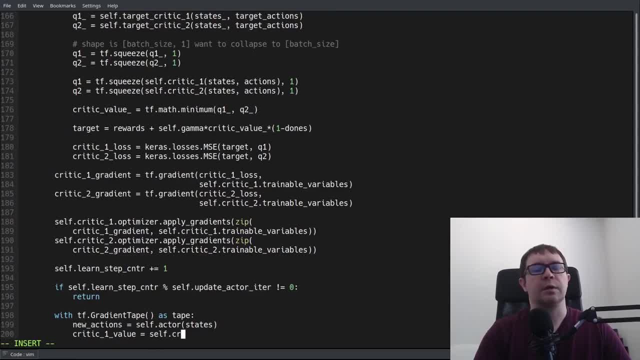 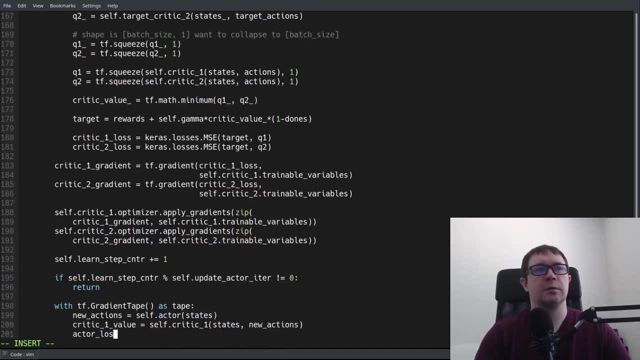 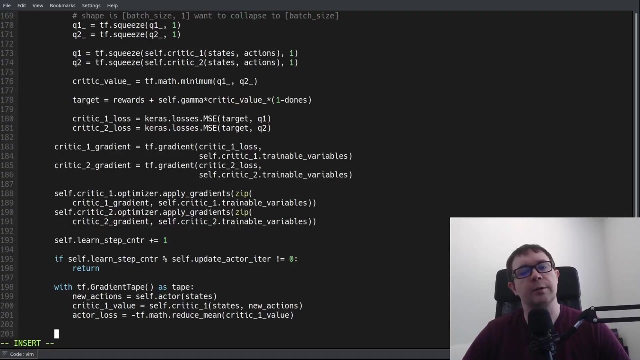 the critic one value is selfcritic, one of those states and new actions and then our actor loss goes negative. tf math reduce mean critic one value, and this may look a little strange to you, but this is how we're going to handle the gradient of the output of one network with respect to the parameters. 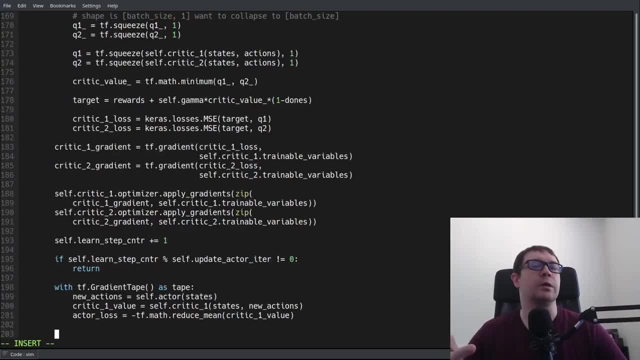 of a network. it's kind of like how you apply the chain rule to the, to the loss of the output of the critic network with respect to the parameters of your target actor, your actor network. sorry, i hope that makes sense. so then we do the same thing where we calculate our green gradient tape. 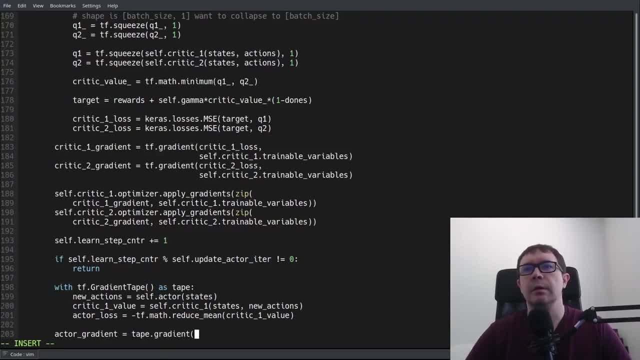 dot gradient. uh sorry, tape dot gradient did i call? let me make sure i didn't make a mistake. i did make a mistake up here, sorry. so this should be tape dot gradient, not tf. that is one less error to worry about when we get to running the program. 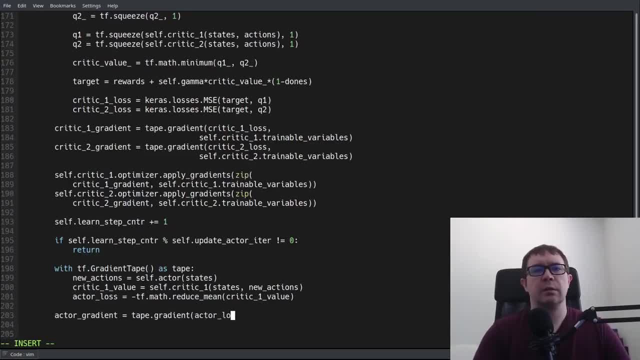 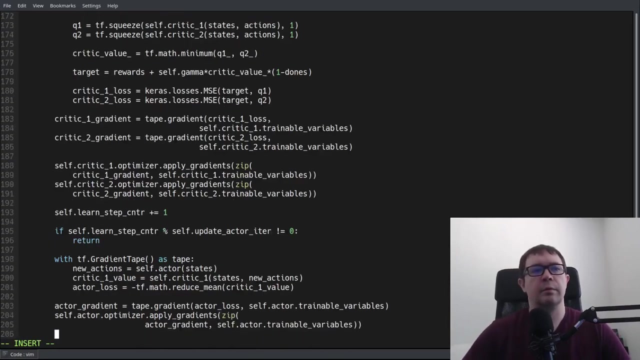 sorry about that. so tape dot: gradient, actor loss, actor trainable variables. i'm going to step our optimizer by applying our gradients again. that takes a zip as input: actor gradient, selfactor, trainable variables. okay, so then, finally, at the end of the learning function, we want to update our network parameters. 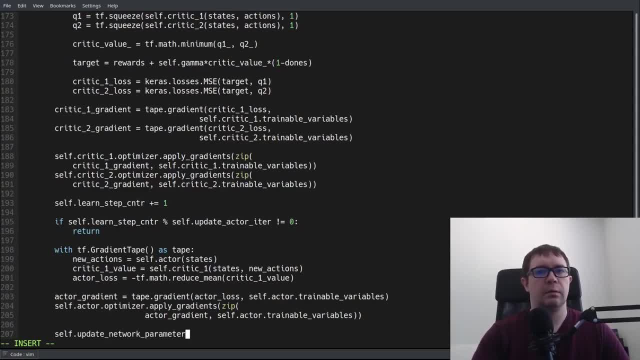 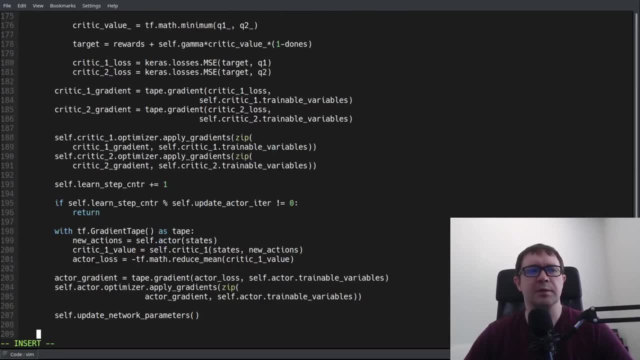 as an order. so let's see, here we've got our learning algorithm okay. so that really handles all of the learning algorithm for our agent. all that's left now is to update our network parameters and then handle the model saving. so just a few functions left and then. 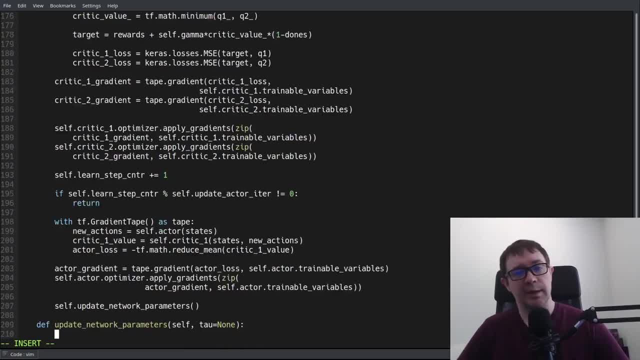 we can go right our main loop and see how it does so. network parameters. value of tau for none. remember that at the top of our- rather the end of our- initializer we pass in tau equals one. to handle a hard update. every other time we're going to pass in a none. so we'll say: if tau is none, then tau equals self. 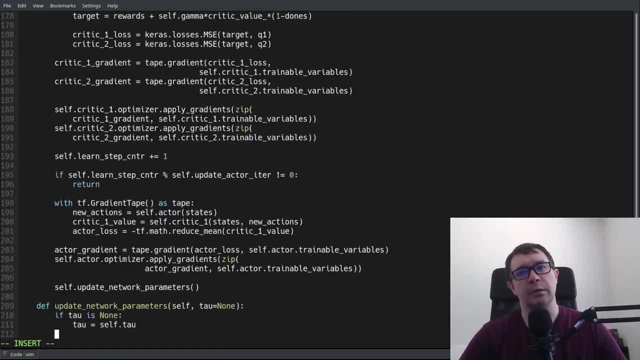 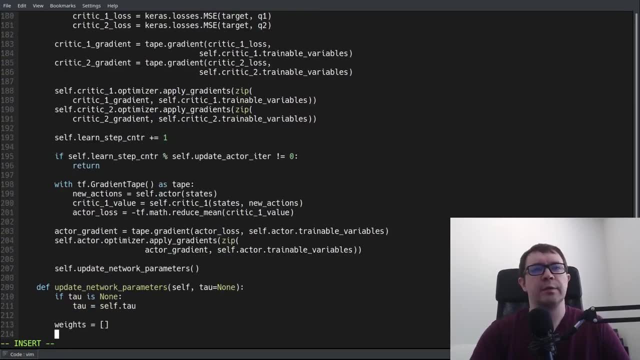 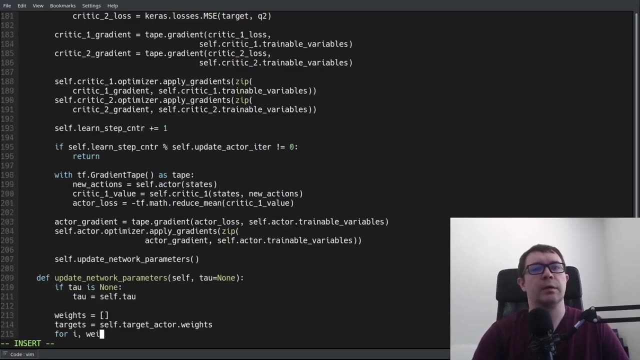 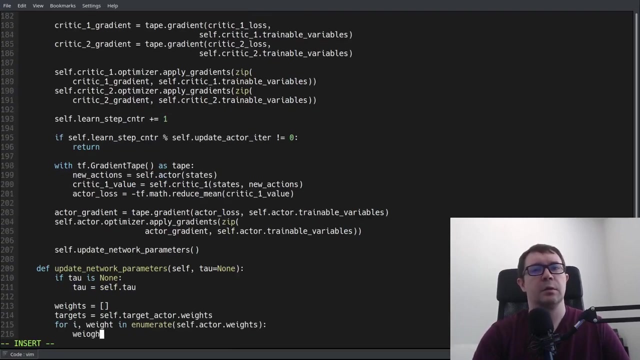 dot tau. so every time other than the first time we call this, we're going to use the stored value for tau. so weights equal and MD list targets equals self dot, target actor dot weights. for I wait in enumerate self actor weights: Bates dot. append weight times: tau plus targets, sub I. 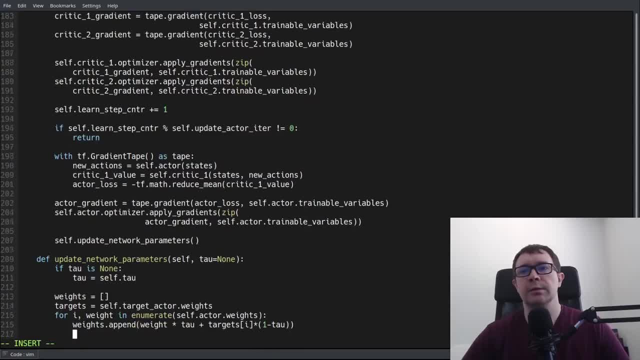 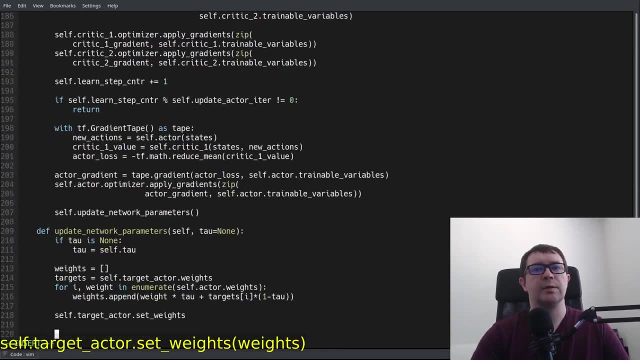 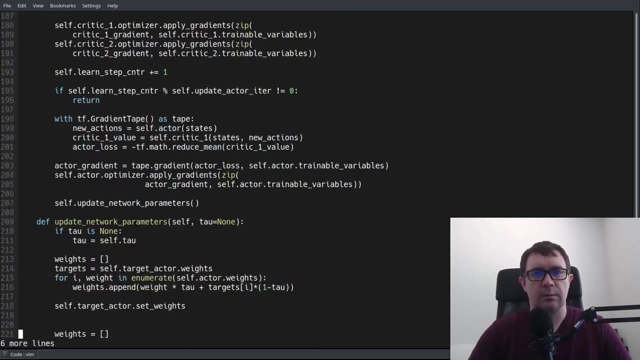 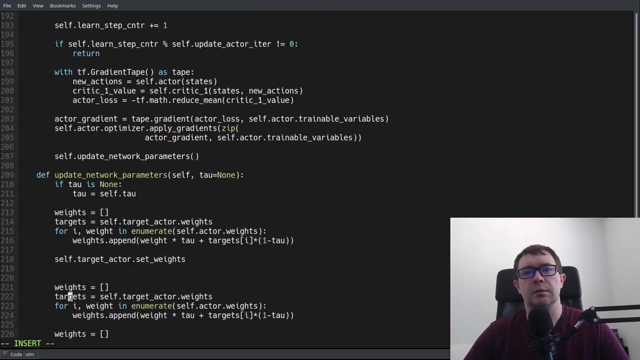 times one minus tau. there we go. and then self dot, target actor dot, set weights. and I am going to yank this and paste and paste again and then say: target critic one selfcritic1 weights, set weights. sorry, I forgot to set the actual value of the weights. 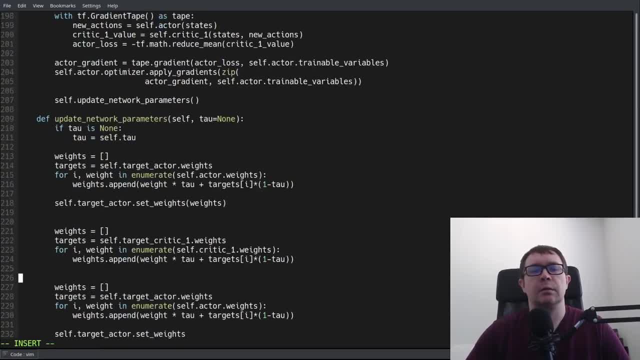 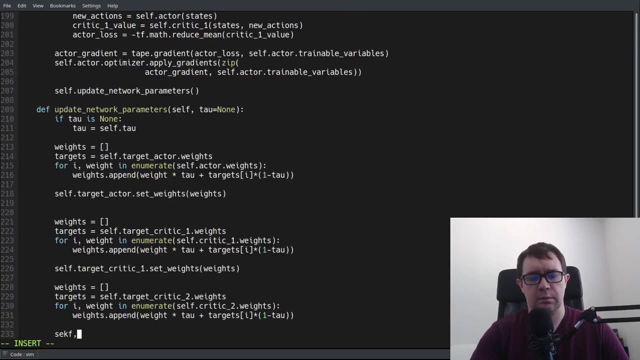 how sloppy of me. and then say: selftargetcritic1 set weights, weights, and then we have target critic2, enumerate critic2 weights, weightsappend, and then selftargetcritic2.setweights, and that handles our update rule for our two networks. 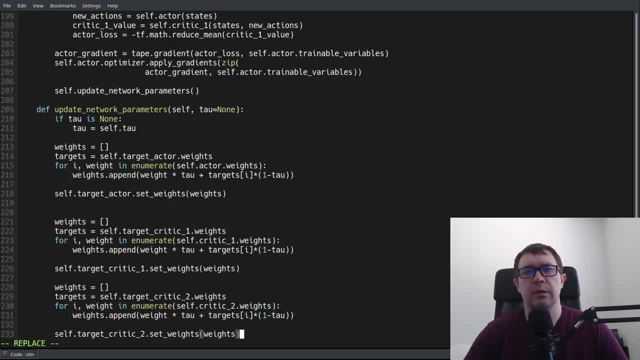 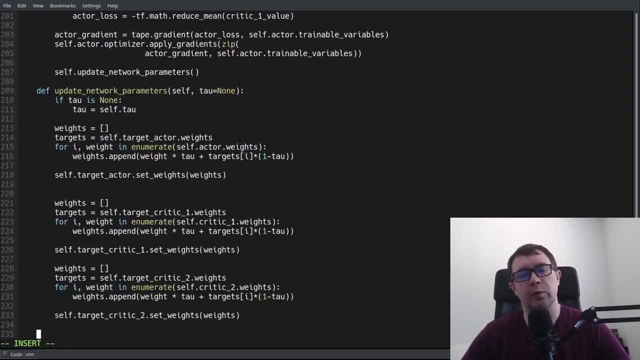 Sorry, my numlock key is off there. Okay, so if it isn't clear what's going on here, we are iterating over the weights of our actor and critic1, critic2 networks, then we're doing the calculation for the soft update. 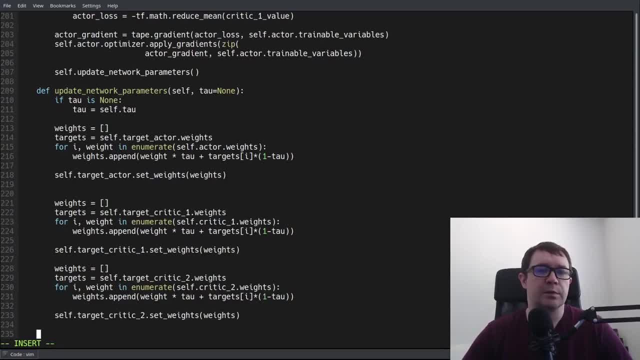 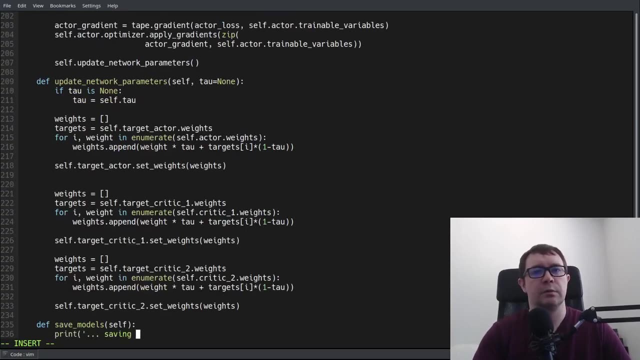 rule, saving that in a temporary list and uploading that list to the target actor or target critic1 or critic2 networks. Now we can handle the save model functionality. This is the easiest part of the whole project. So print saving models. just a little debug statement to let us know something is going on. save weights. 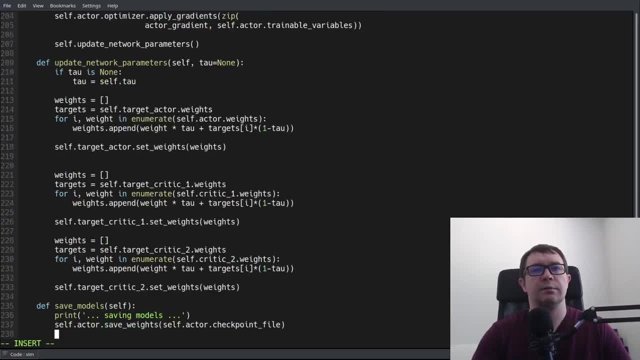 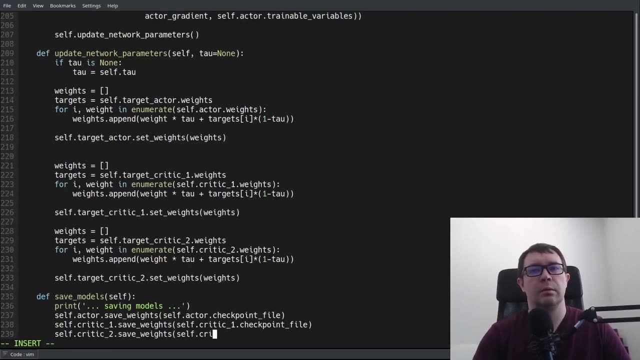 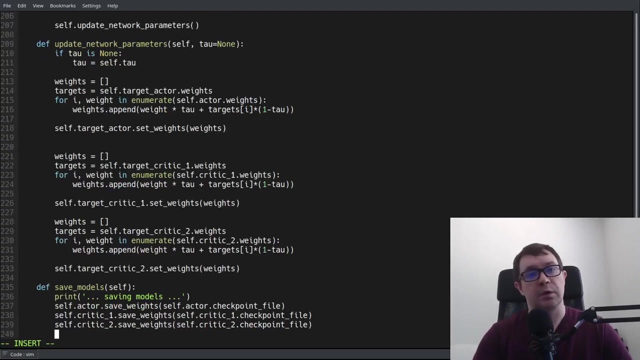 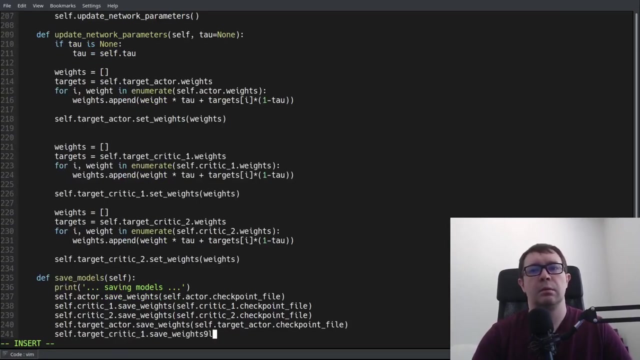 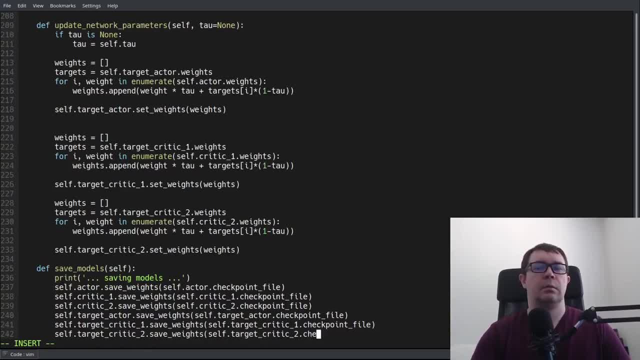 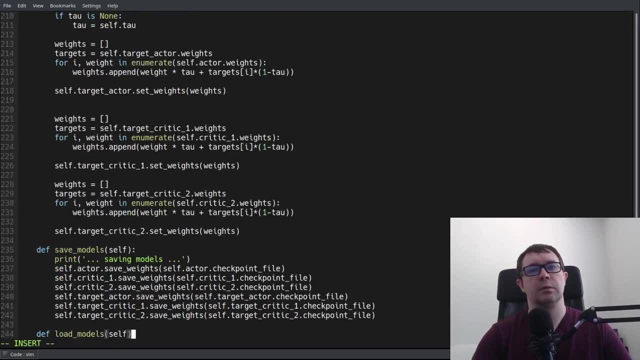 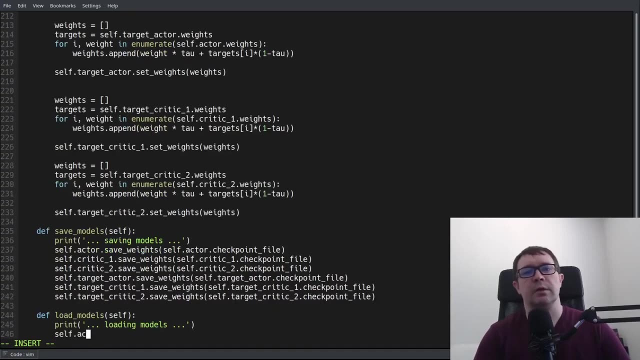 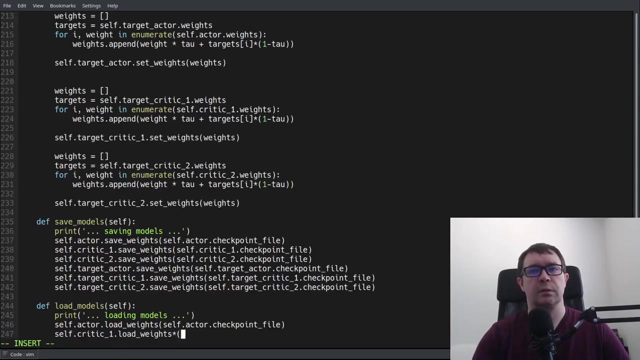 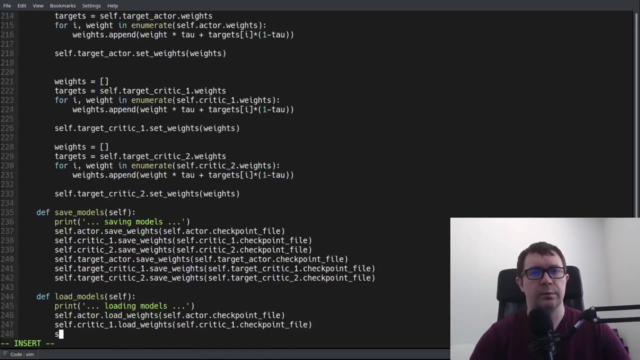 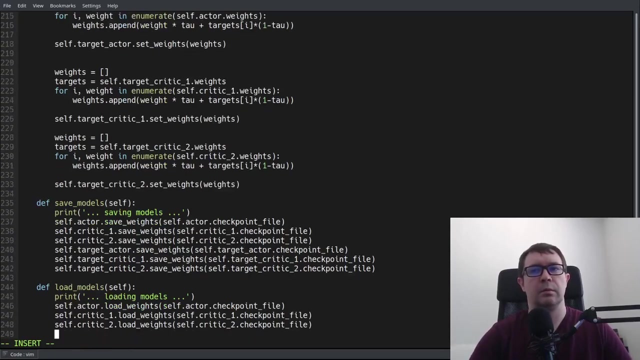 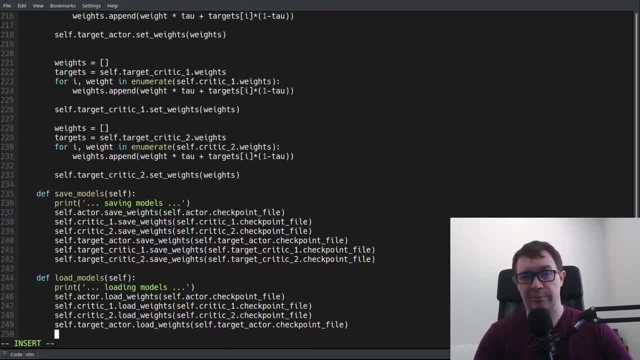 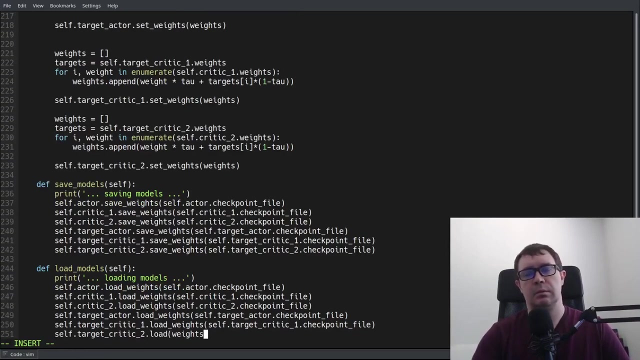 I should have chosen shorter variable names to save my wrists a little bit of work here, but hindsight is always. 20, 20, I guess target predict one checkpoint file. okay, so that is it for the main code for our td3 algorithm. now we get to handle the main loop. so 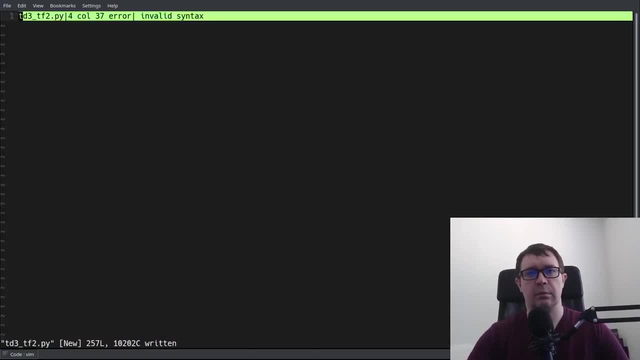 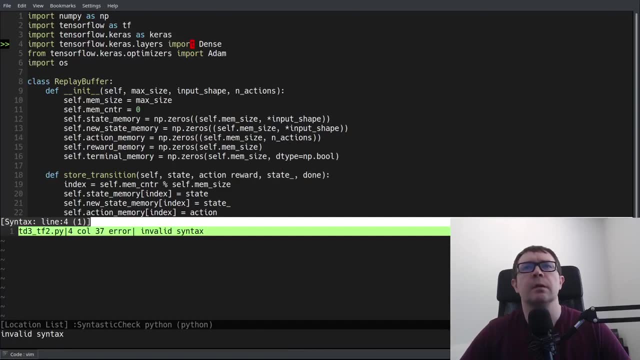 let's go ahead and code that up now, of course, before we can. I have an invalid syntax right here at the very beginning: tensorflow: dot, keras, dot layers. oh, sorry, that's because it's a from import dense. I'll have to notate that in the video. and I have another issue here: deaf store transition- where is it? 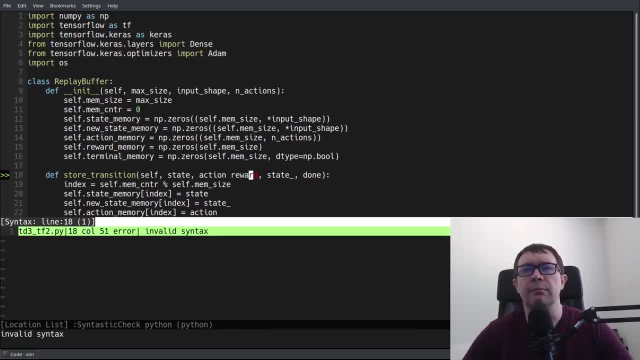 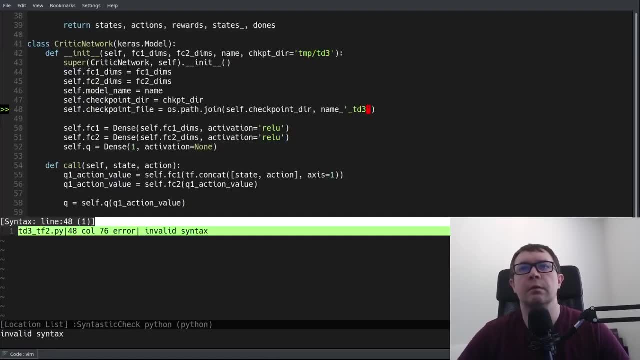 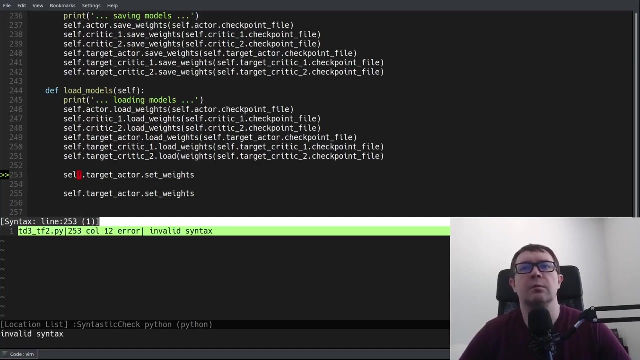 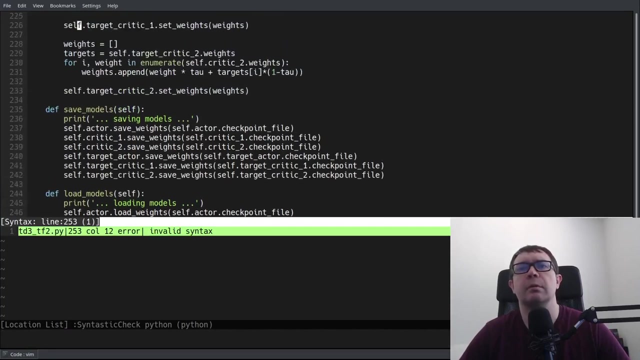 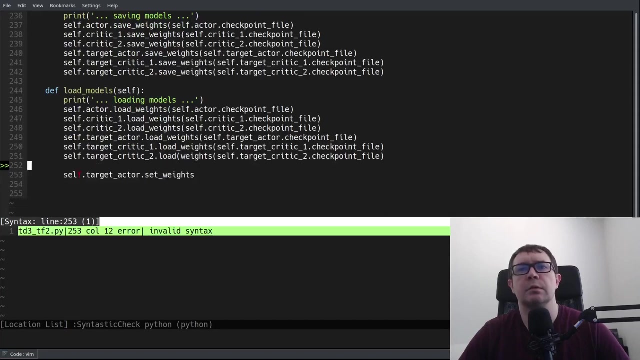 unhappy. I am missing a comma, of course. and I have another issue: OS path join name equal you. yeah, my wrists are non-functional today. self dot, target actor, dot set weights. oh, why did that happen? interesting, did I type those at the end and have a stroke or something? don't remember it very. 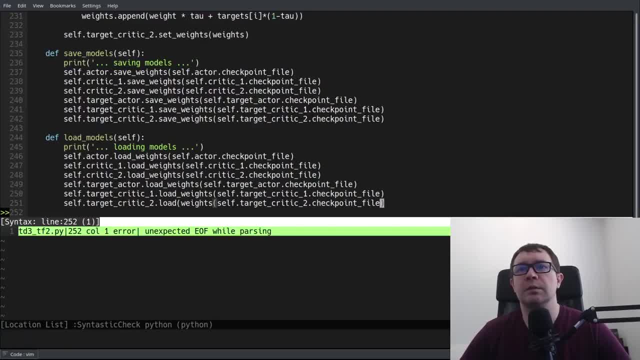 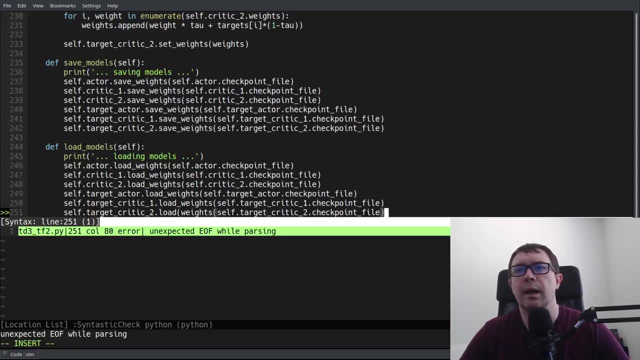 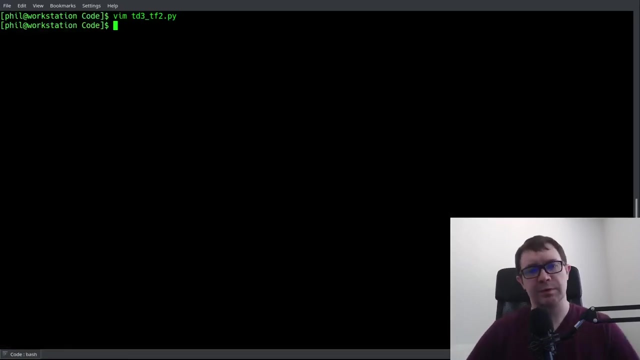 strange, okay, unexpected, and a file on my density somewhere. I because I have right there. all right, finally, good grief, that's a whole lot of typos. now some people suggest that I upgrade. repent Kontos too. I've improved, supposed to go open it on. all right, finally, good grief, that's a whole lot of typos. now some people suggest that I upgradeノ. 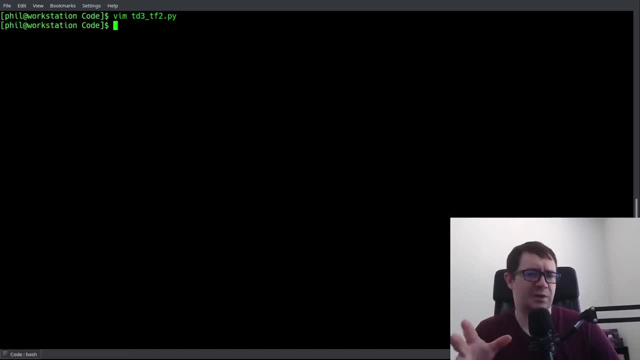 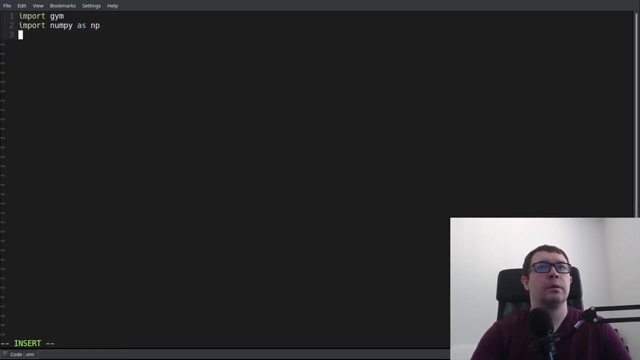 suggest that i upgrade my vim and to actually catch that stuff on the fly. and you're absolutely right, i'm going to do that when i finally force myself to do it. let's go ahead in the meantime and write our main loop. so we want to import jim numpy. we'll need our agent. 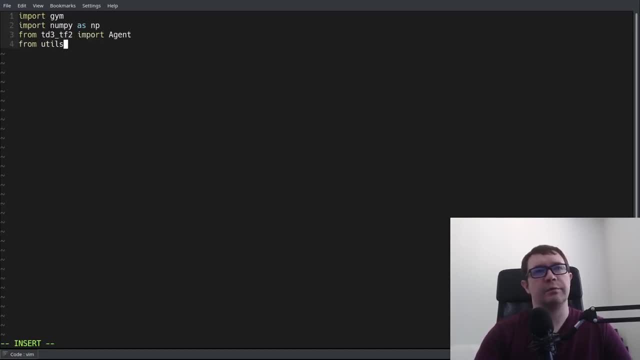 and we'll need our utility file. uh, plot learning curve. you can do a git clone on my github to get that. it's just a matplotlib pi plot with some labeled axes, uh, where we're taking an average of the previous 100 games running. um, i don't include that in all my videos, i just kind of. 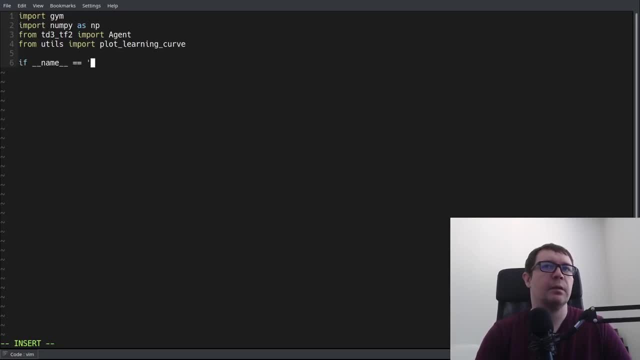 reference my github. you can just do a plot if you wish. um, you can just do a plot if you wish. you can just do a plot if you wish. name equals main jimmake. we're going to be doing the bipedal walker v2 and we're going to call our agent. 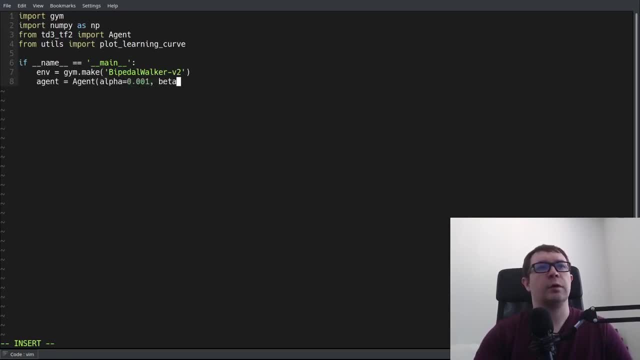 constructor: alpha 0.01, a beta of 0.001. our input dimensions will be determined by our environment, so we don't have to hard code anything. a tau of 0.001, 0.005, pass in our environment. batch size: i have a hundred here. 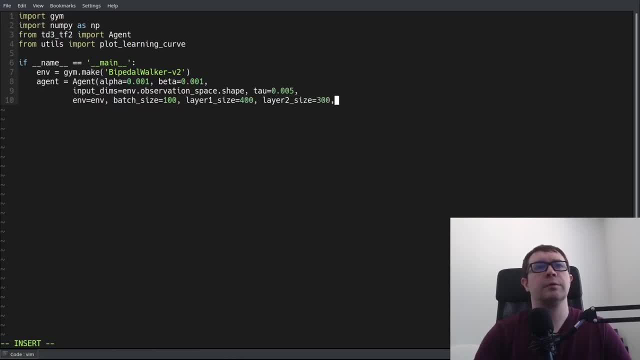 equals 400, 300 and an action is determined again by our environment. we'll let this bad boy play a thousand games and we'll call our file name plots plus walker underscore. now, keep in mind, you have to do a make-der plots and make dirt temp slash gd3 to correctly execute the code, because it'll expect that those 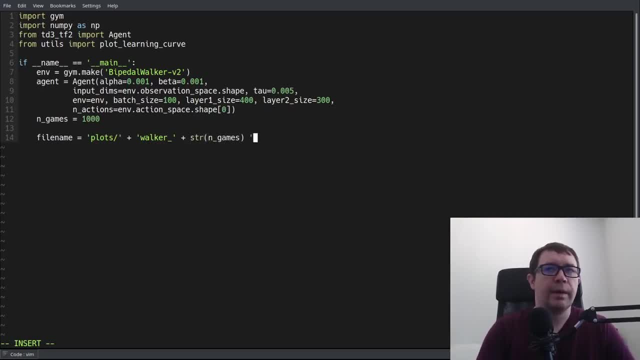 directories exist. pass a number of games as a variable for your file name. that way, if you run it over and over again with different numbers of games, it won't override the same plot. you can also include things like learning rates as part of your variable name for your file names. i recommend doing that if possible, and i'm just more interested in doing some data analysis. obviously, if you want an application more suburban management can zombify that data function and you can see that as a lot of data phenomena and the relationships of repo editor are the most useful factors in it. so say, perhaps fd war is not mustard fighting out with становится acting out of value algorithm, which is an interesting 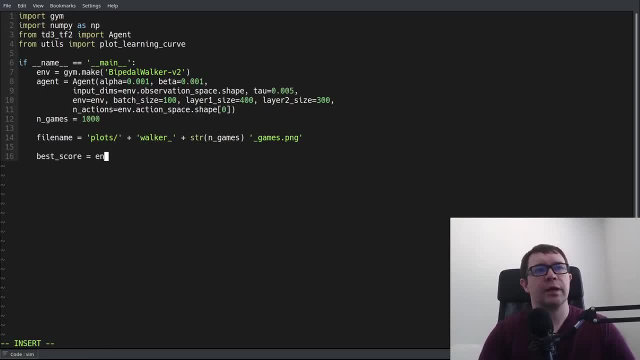 I'm just not doing it here. So we need to keep track of our best score. It's the minimum score of our environment And the reason is we want to save our best models. Keep track of your score history. If you want to load models, now is the appropriate time to do that. Actually, you know. 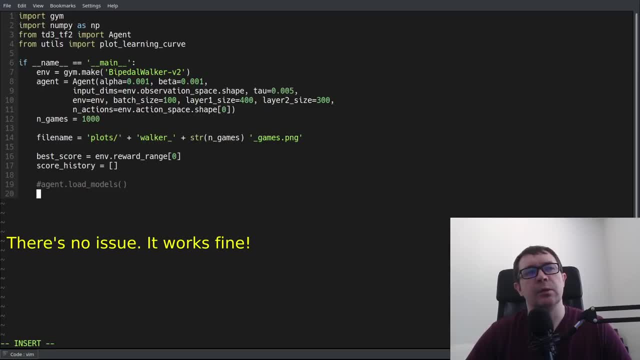 what We may need. there may be an issue where we have to actually instantiate our network with some variables to load the models. Open up an issue on my GitHub if that's the case and I will write the correct code. I won't bother with the video. I'll leave that as an exercise for the 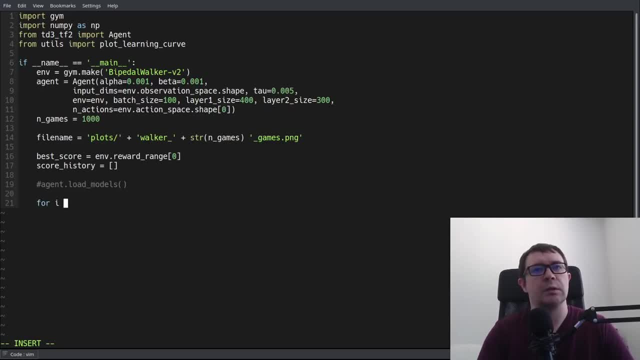 viewer. But if it turns out to be a problem, raise an issue and I can fix that. Not a huge deal. Let's go ahead and play our game. Start by resetting the environment at the top of every episode. Reset the done flag and zero. 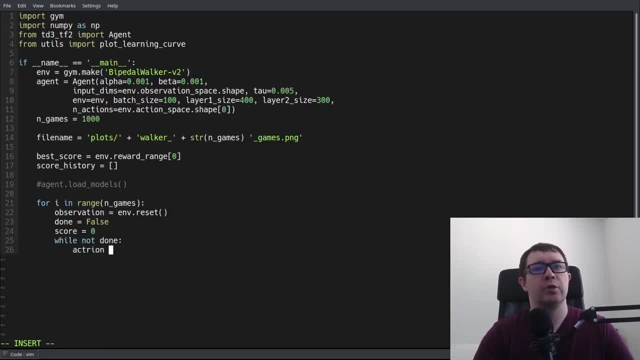 And let's play our episode While not done. Action Eagles agent dot. choose action based on the observation. Let's take that action. Get the new state reward done and debug info from our environment. Call our learn function, Keep track of our score and set the current state to the new state. Very important If you don't do. 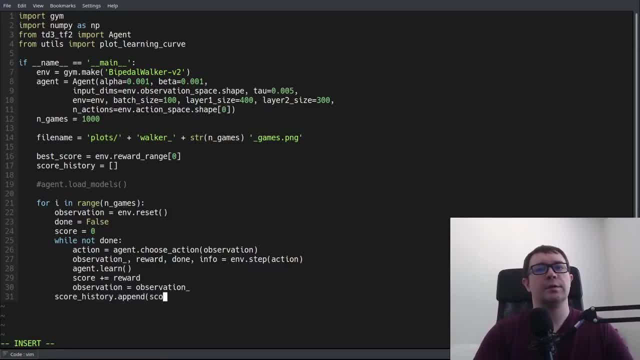 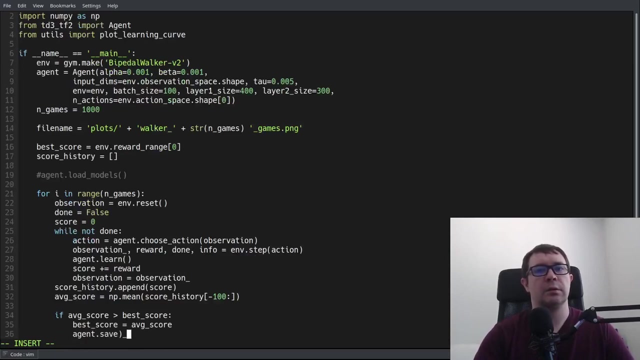 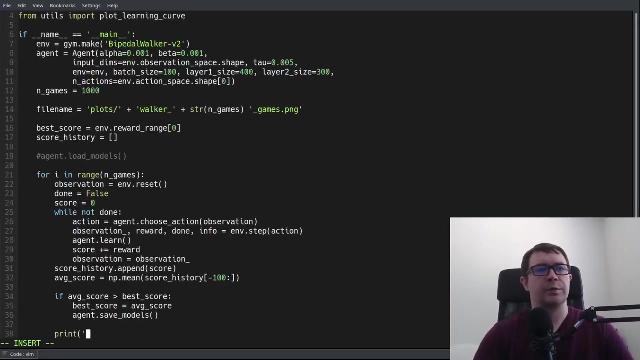 that nothing is going to go well for you. Let's depend on our score at the bottom of every episode and calculate our average Minus 100 onward. If our average score is greater than our best score, then set the best score to that average and save our models. And then we want to print some debug. 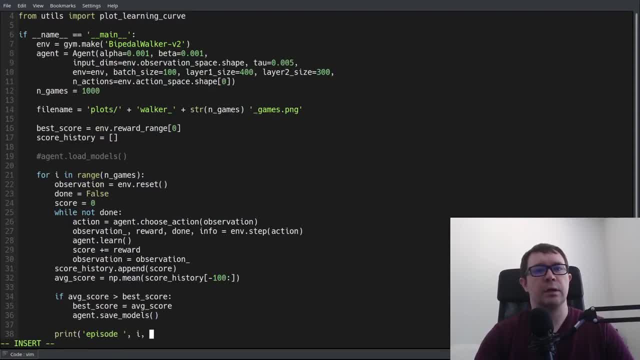 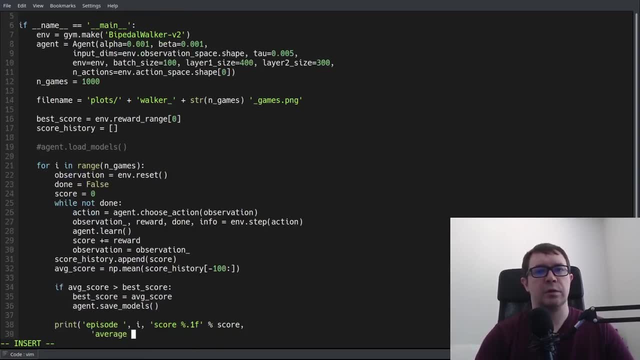 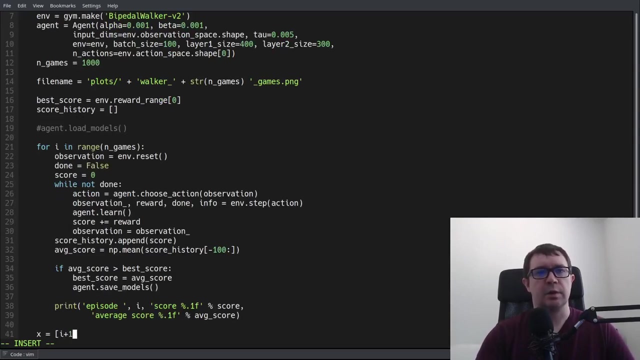 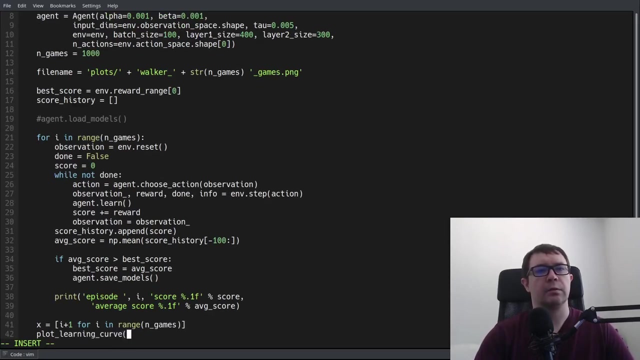 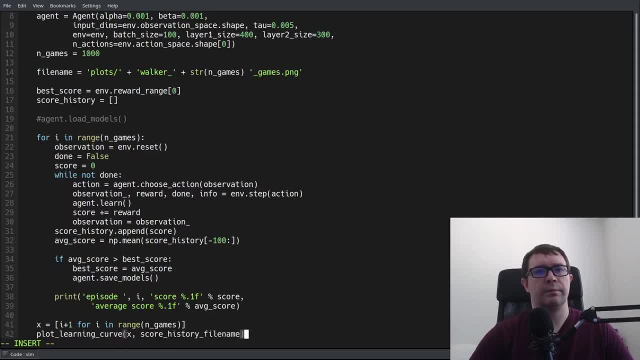 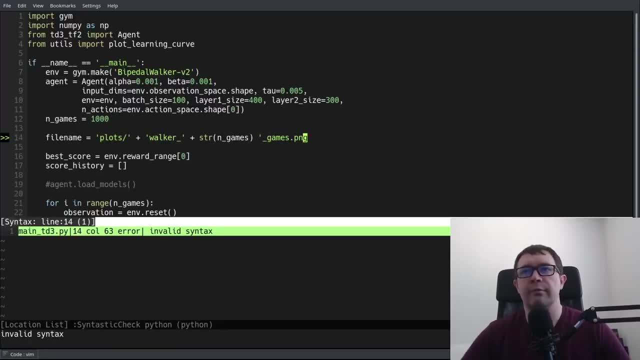 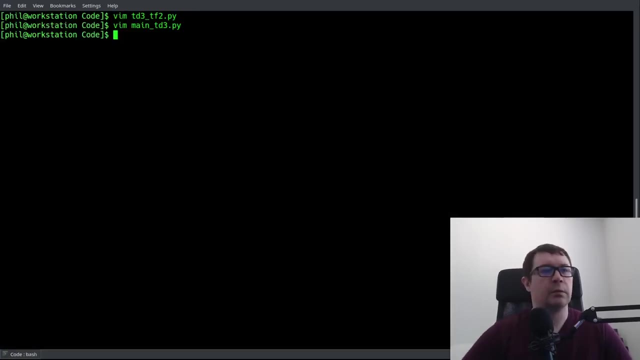 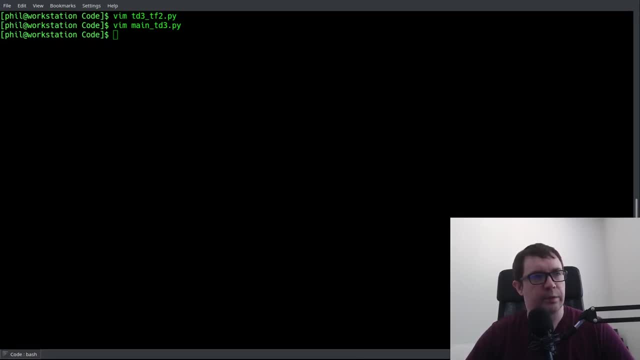 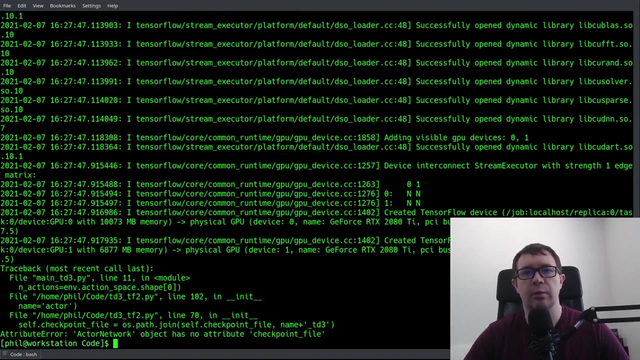 And okay, so it saves models. it is learning. That is good to know. let's do a make der temp slash TD3. I Should already have plots Python main TD 3.5. moment of truth. Okay, so it says actor network object has no attribute checkpoint file. I 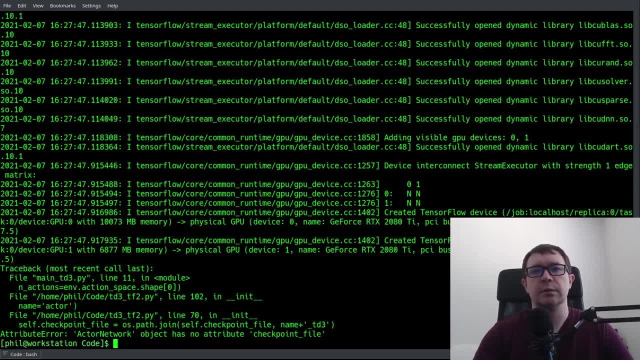 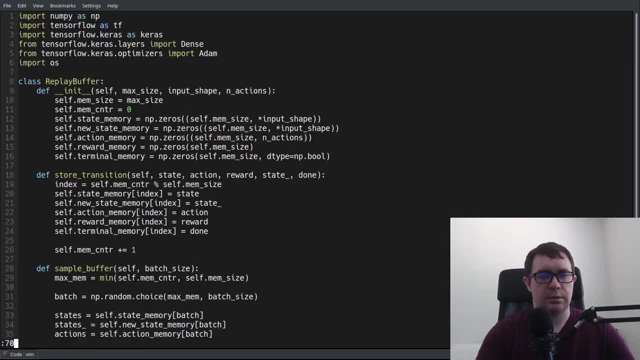 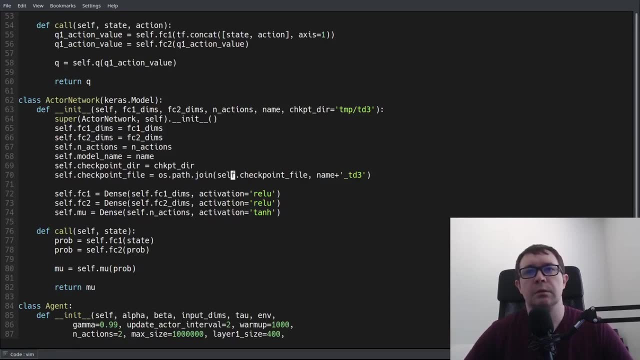 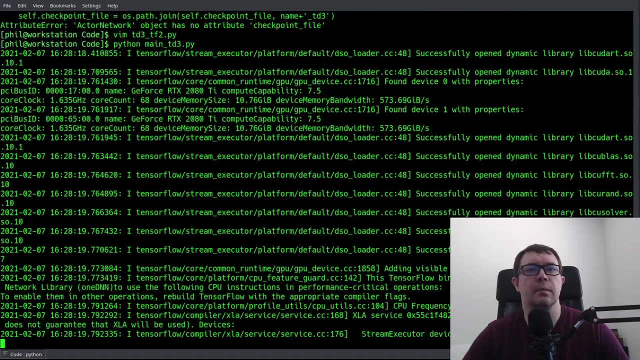 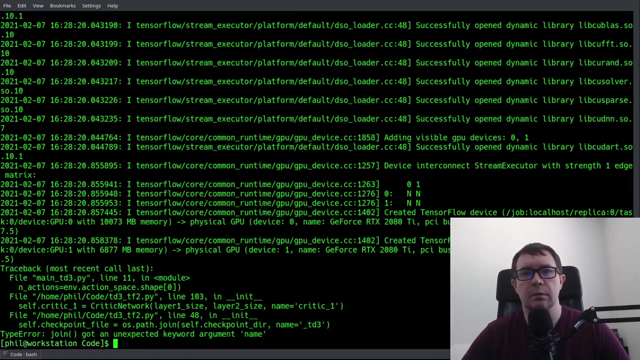 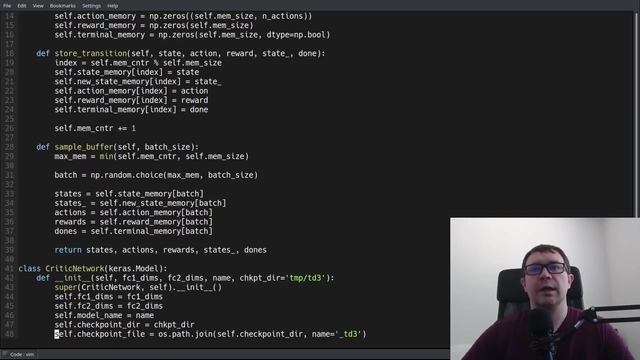 Didn't? oh, it's checkpoint directory, So that is in TD3, TF2. that is in line 70. So That is here. Okay, Try it again. Got an unexpected argument: name that is in: oh, That's because. Okay, that is in line 48. that is super trivial. 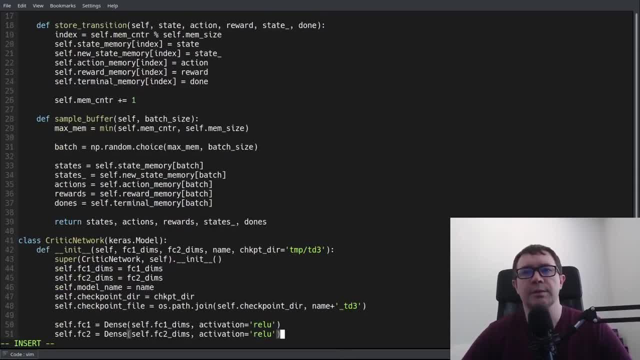 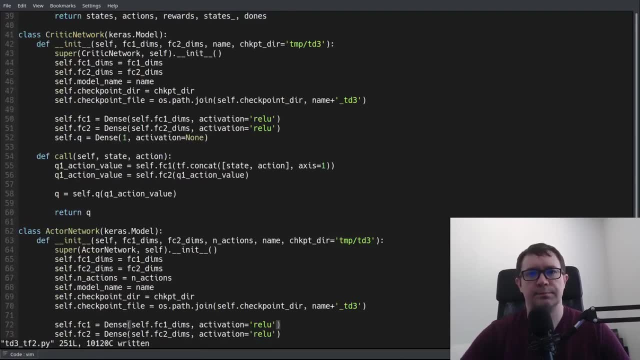 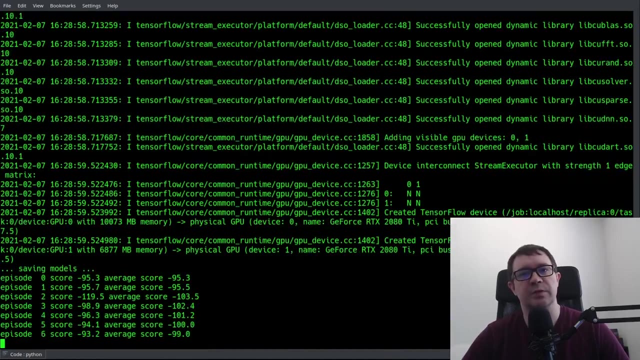 It's not. name equals its name Plus, did I do that Down here as well? No, I did not. I'm not looking forward to editing this. This is gonna be a lot of work. Okay, so it saves models right off the bat and starts running. 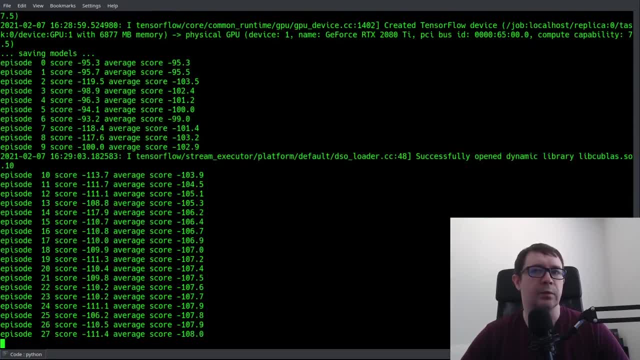 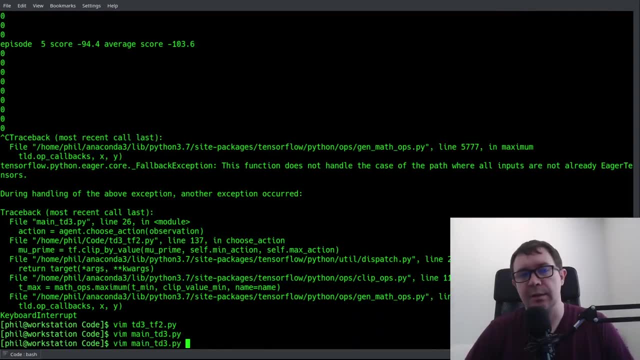 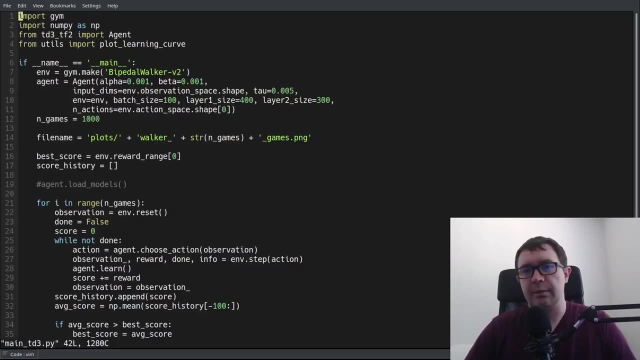 Okay, so I'm gonna let this run for a while And then we're gonna see how it does. Okay, so I did something very stupid and I let it run and noticed it wasn't actually learning, and so That's a problem. And the reason it's not learning is because I forgot to store the transition. 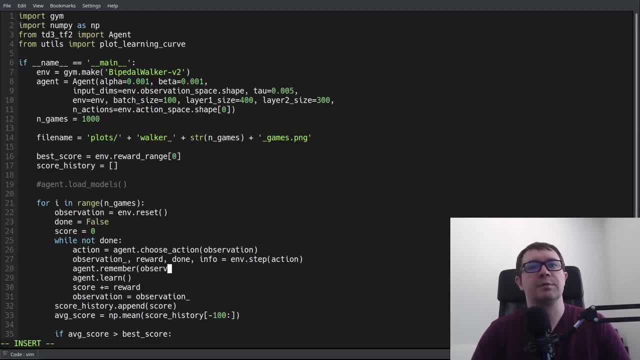 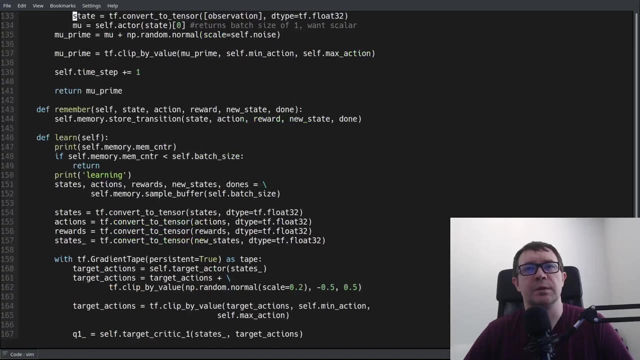 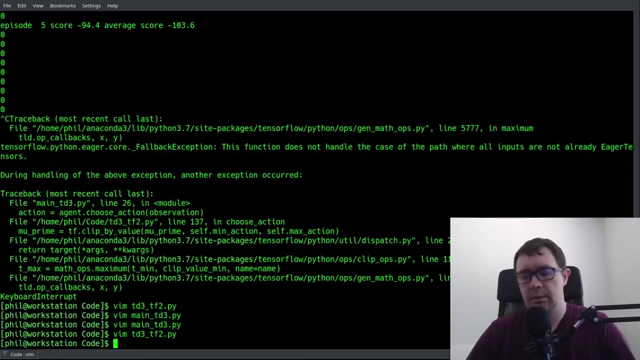 so we have to say agent remember observation, action, reward, observation underscore and done okay. and then I got to get rid of the Print statements. I stuck in here for debug purposes, Because I'm a noob and use debug statements. okay, Now let's do Python main td3. 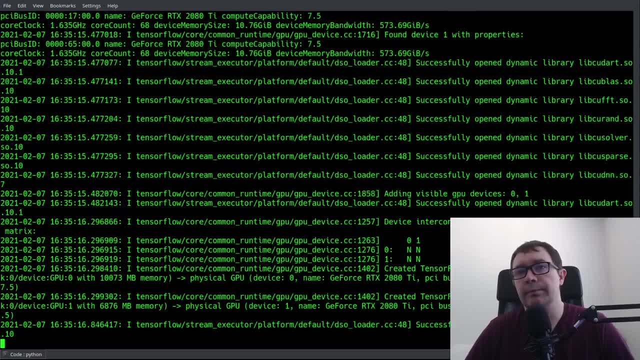 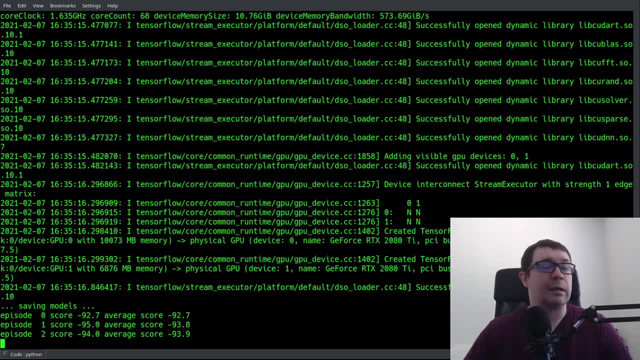 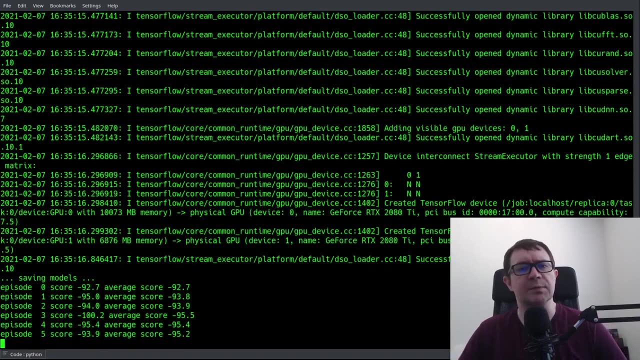 Dot PI, and now it should work Without any funky print statements. okay, Now I'm gonna take off for a little bit and see what's going on, And the reason I noticed this wasn't learning is because it was executing much too quickly. I blasted through 350 games in just about a minute, which tells me it's not doing anything useful on the GPU. 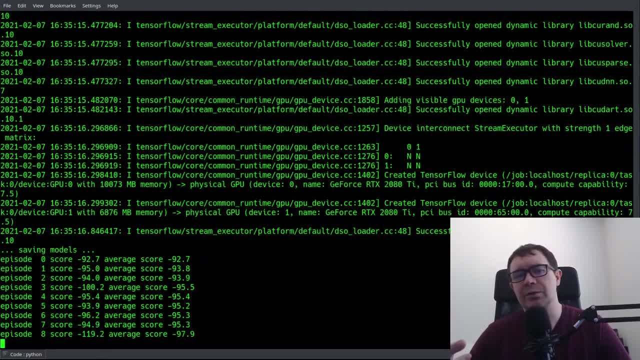 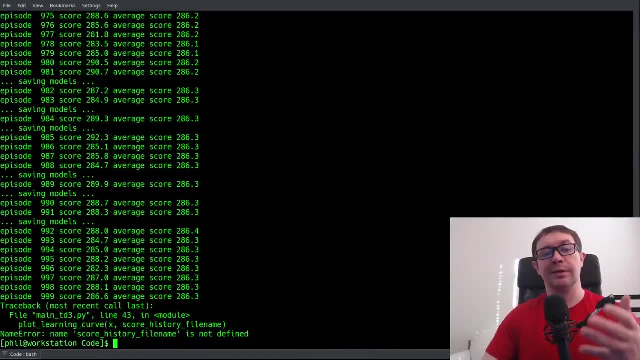 So I'm not this run. that'll probably take an hour or two, and then I'm gonna come back and see how it did and we'll Take a look at his performance. Now, here we are. it's the next morning. this took around six or seven hours to run. 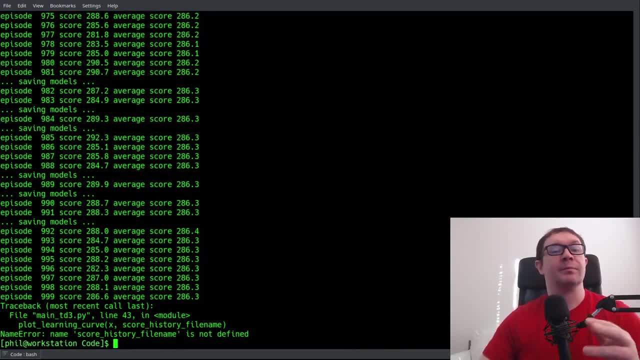 So I just waited until morning to film this, but, in typical Phil style, the file name for the Function call for the plot learning curve function has a typo in it, And so we don't have an actual plot from the performance of this particular run. However, I will show you a plot of a similar run, where it achieved an approximately similar score. 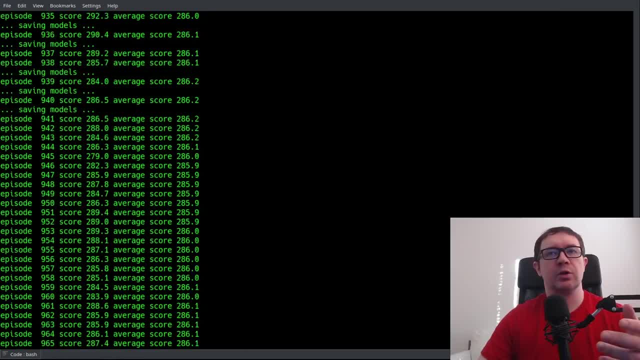 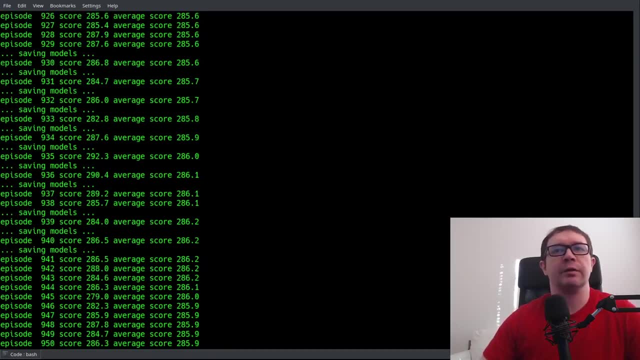 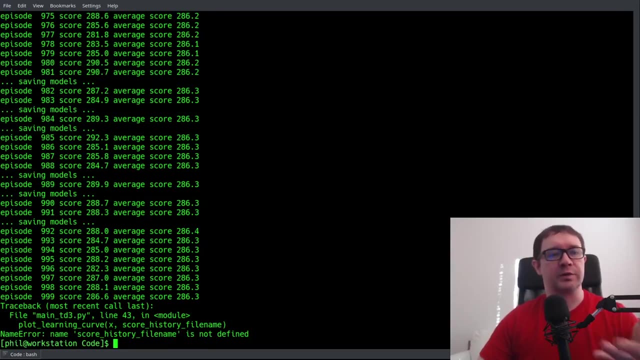 You can see that it does indeed learn it. She's a high score of around 285, 288, about 290 or so, depending on the run. you get some run to run variation and And 300 is the highest possible score you can get for this environment. 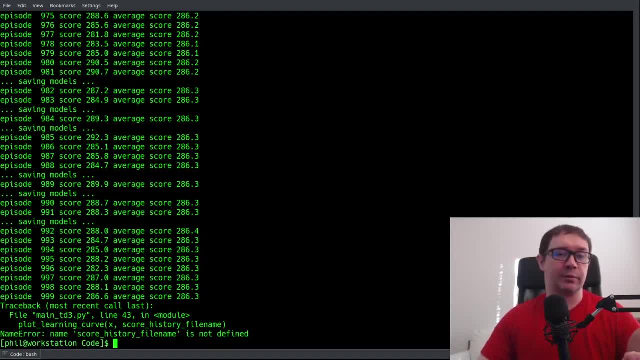 So I would consider this pretty much strong evidence of learning. It's not a world-class result, but that's not what we were aiming for anyway. we just wanted to understand the gist of the algorithm and implement it correctly and Demonstrate that we do in fact understand how it works. mission accomplished: You can pat yourself on the back for that.